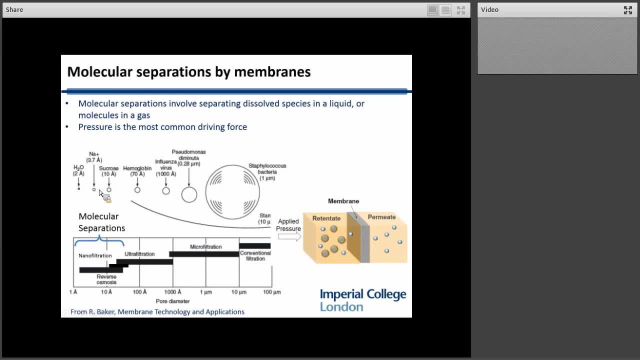 10 angstroms or, for example, in the case of salt, even less than a nanometre. so sodium is 3.7 angstroms. So typically the sorts of pore sizes that we would need in a membrane for molecular separation is in the range of an angstrom to two to three nanometres. So 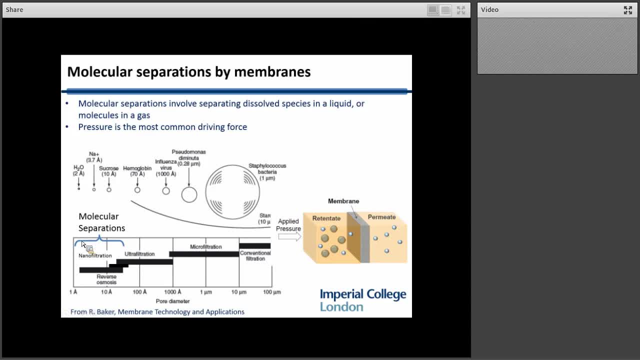 when I talk about molecular separations in this area. here I'm going to talk about the same thing. I'm talking about things like ultrafiltration at the very tight end, nanofiltration and reverse osmosis, And we're talking about removing things that are dissolved in a liquid. 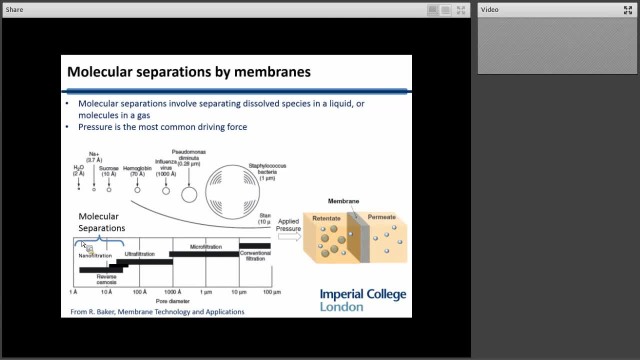 or separating molecules in a gas. The most common driving force for these operations is pressure. So what we'll typically do is have a membrane and we will apply a pressure across that membrane and, depending on the pore size in that membrane, some molecules will be able to permeate through it and some molecules won't, and so we'll achieve separation. 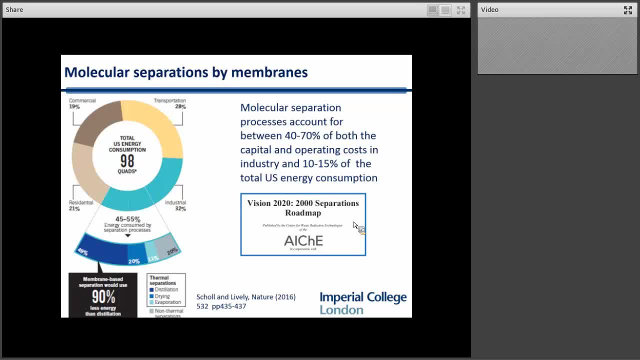 of those molecules. Just to give you a feel for the importance of this topic, I want to share with you some information on the energy consumption in the United States. So the American Institute for Chemical Engineers estimate that molecular separation processes, the kinds of things that I've been talking about, account for between 40 to 70 per cent. 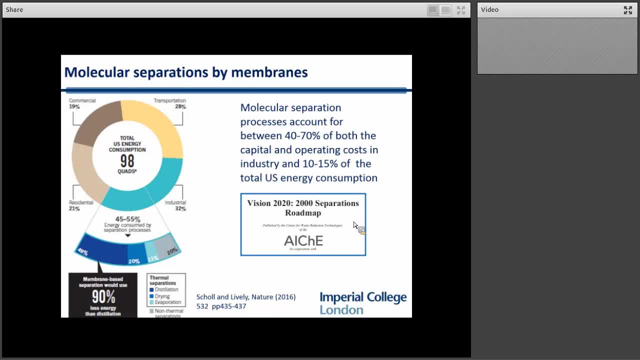 of the energy costs in industry. And if you look at the US data on energy consumption in the US economy and we divide that into residential, commercial, transportation and industrial, you can see from this plot on the left-hand side that industrial use is. 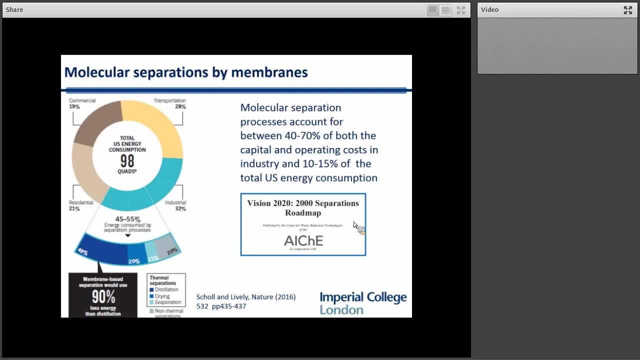 the largest sector for energy use in the US and about half of the energy used in industry is used in separation processes, And of those separation processes you can see that something like half of that amount of energy is used in distillation and another big chunk 11. 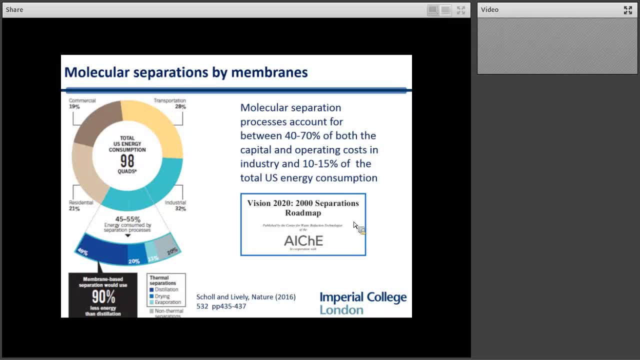 per cent is used in evaporation, And you can see, then, that evaporating liquids, whether it's in distillation or direct evaporation, is a category that's more likely to be used in distillation than in evaporation, And that's the kind of thing that we're trying to do. 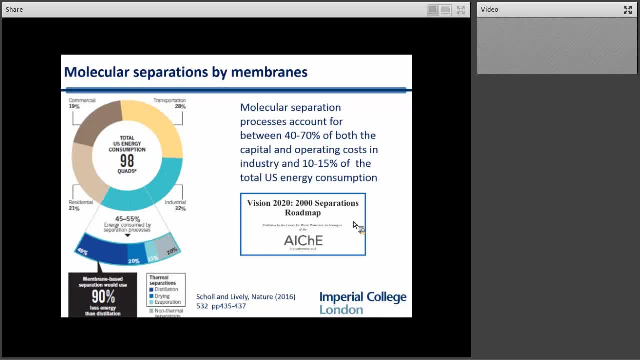 And that's why we're counting for something like 10 to 15 per cent of the total US energy consumption. Why? It's because when you evaporate liquids, you need to separate the molecules in the liquid, And separating the molecules in the liquid takes quite a lot of energy. 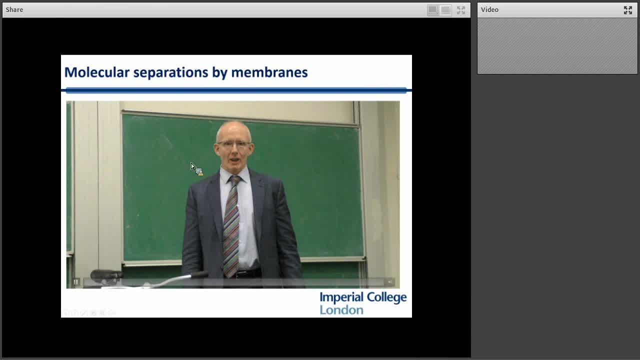 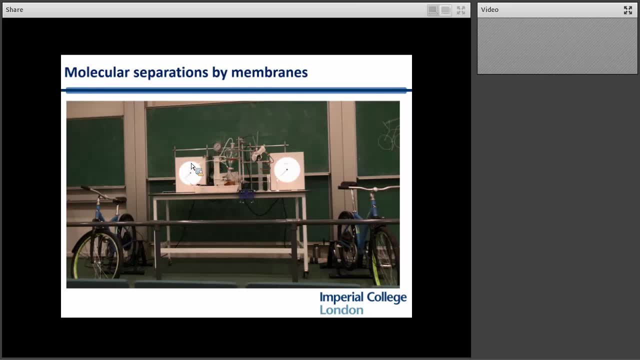 And what I want to do now is just to go to a pre-recorded video that explains to you why that is. I want to go now to a demonstration, using this equipment here, of why membrane technology is so far superior to thermal technology when it comes to purifying water. What I have is: 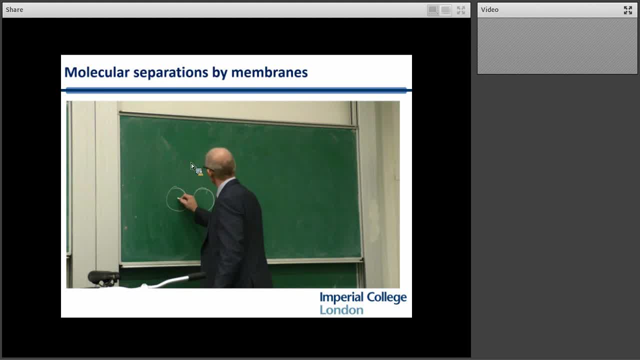 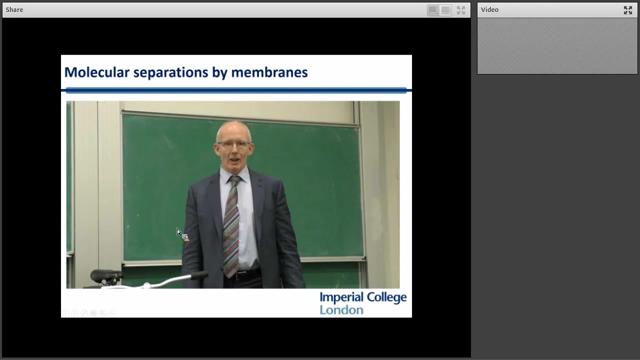 two bicycles, And on this side I have a bicycle which I'm going to sit on, And when I ride that bicycle, what I'm going to do now is to give you a demonstration, using this equipment here, of why membrane technology is so far superior to thermal technology when it comes to purifying water. 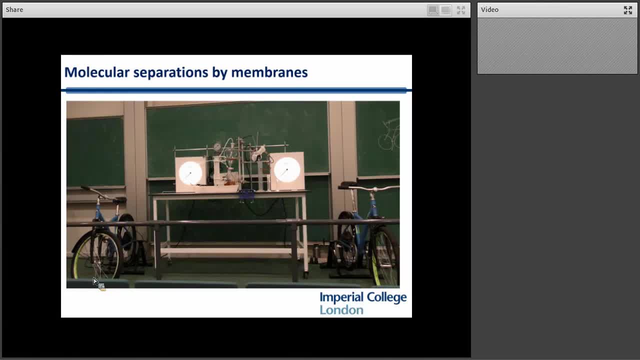 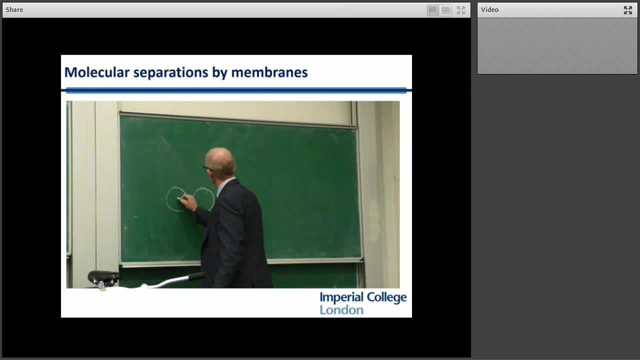 What I have is two bicycles, And on this side I have a bicycle which I'm going to sit on, And when I ride that bicycle, the energy I put into riding the bike is converted to electricity and is generated here, And in this case, that electricity is going to. 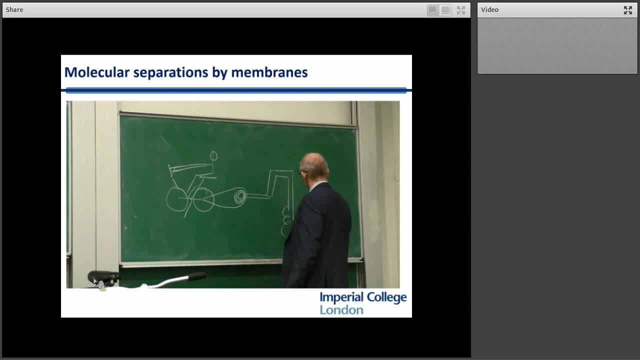 be used to heat a coil, And that coil is like the coil that you have in your kettle when you boil water. So, as I ride the bicycle, the energy that I produce will be converted to electricity and used to provide heat to this kettle, where the water will boil. the 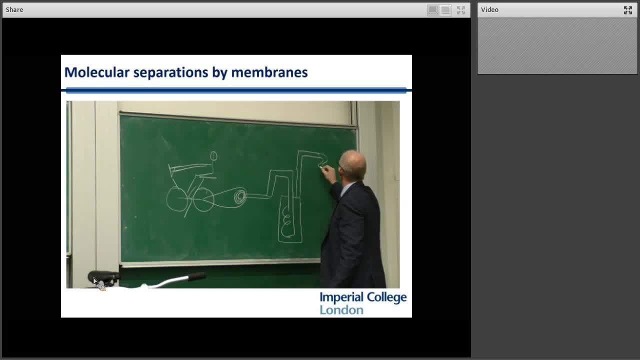 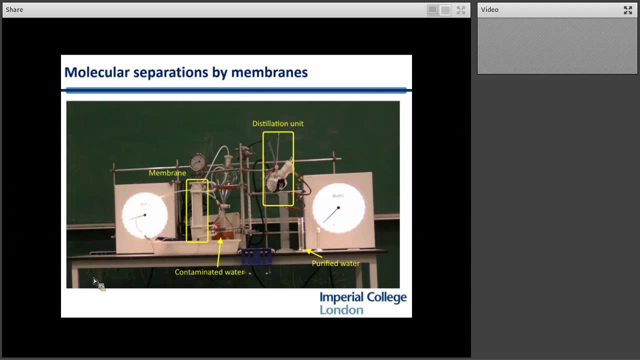 water will come off, it will go through a coil where it pulls down, and purified water will be collected in this cylinder. So you're going to see, as I ride the bicycle, that I've produced energy And I boil water using the energy that I've produced. So let me just get this one warmed. 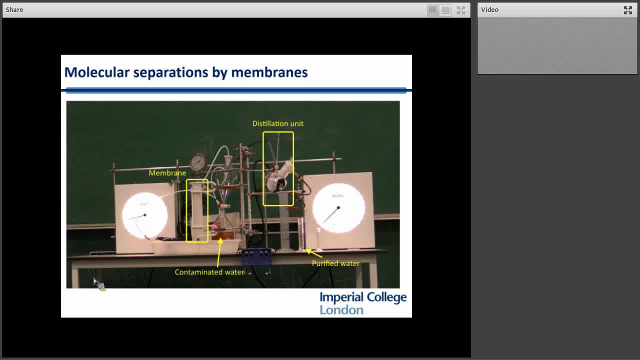 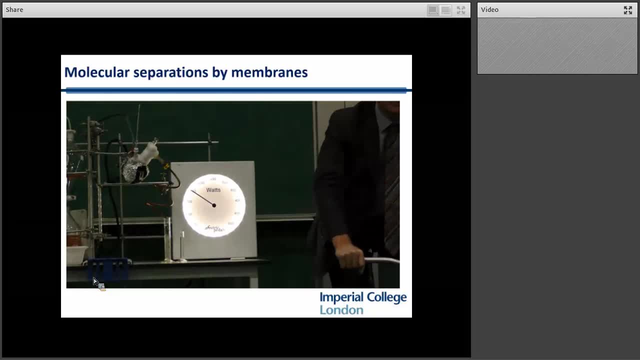 up, get it going up to speed And once I get it up to speed you can see. here's the amount of energy I'm generating. Then the water starts to boil and I recover water. So if I bike and I think I'm not as fit as I maybe should be, I'm starting to get a little bit breathless. 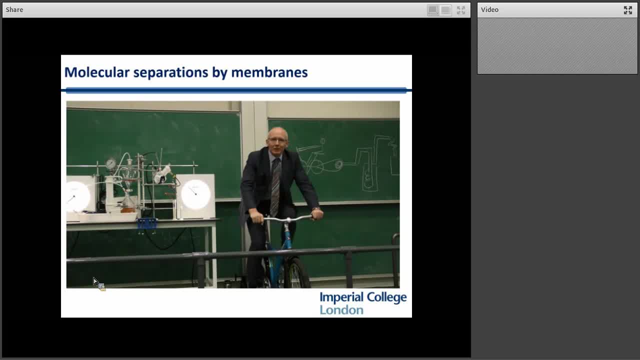 I'm going to time myself for one minute shortly. as I bike and I produce this energy. this energy is being generated, This energy is being converted to electricity and boiling the water, You can probably tell that I'm starting to get a little bit short of breath. I'm into my minute now, So I'm 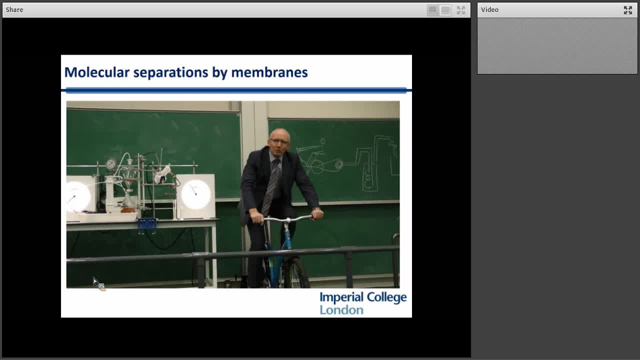 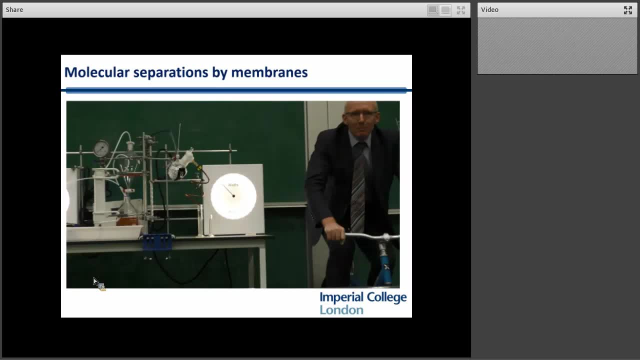 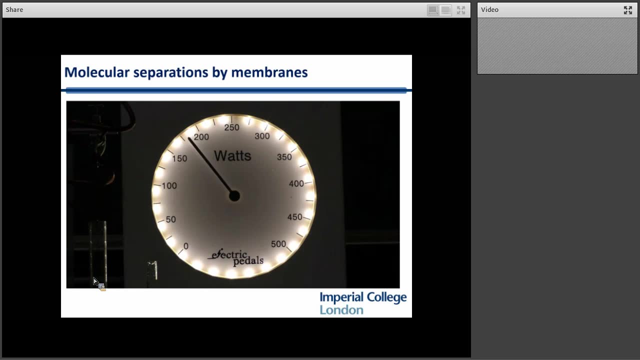 going to bike for one minute and see how much water I can produce. So all of the output of my biking now has been converted into electricity That's being used to heat the water, boiling the water, and I'm about 30 seconds through now. You can see I haven't produced a lot. 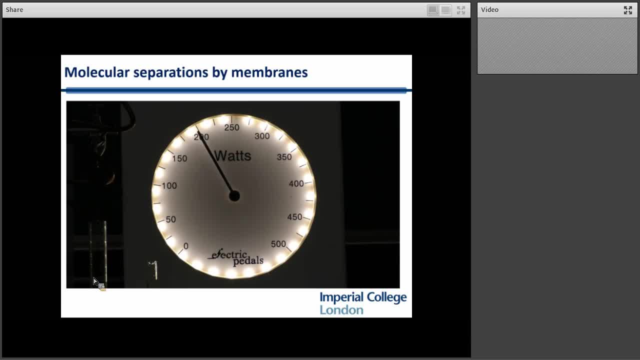 of water. yet This distillation is going to take a little bit longer. but it's going to take a little bit longer. This distillation, evaporation business takes a lot of water. Oh well, someone needs to invent membrane technology. This is just no good. Now under. 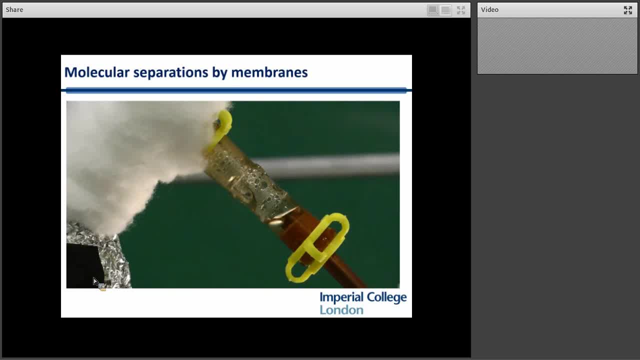 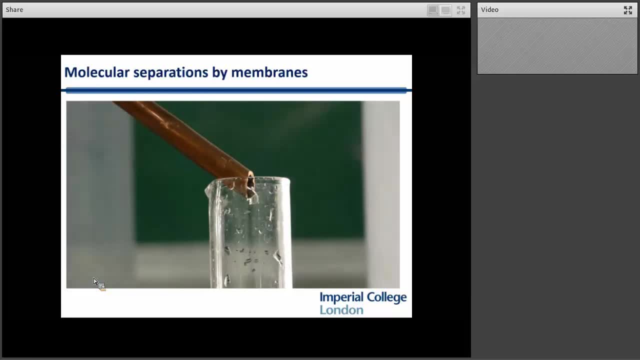 the cave name was so fit. I'm coming up now: 45 seconds. I've got my first drop, my first drop of water After 45 seconds. I've had to go up to over 200 watts and I can tell you I'm feeling it. 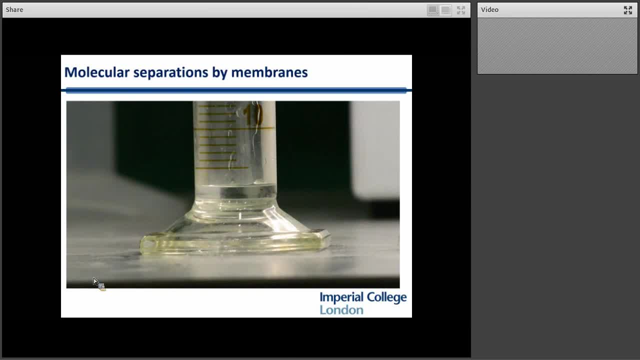 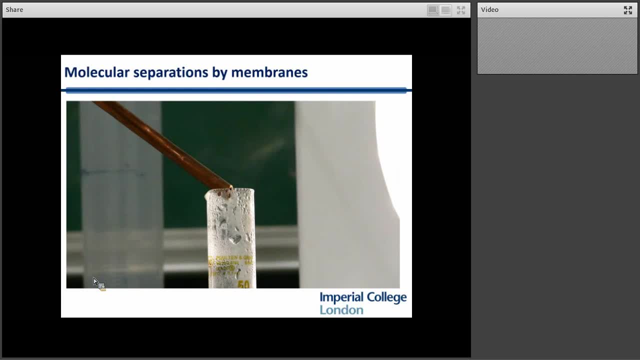 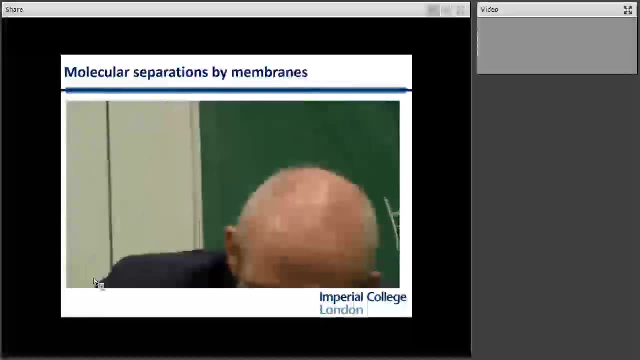 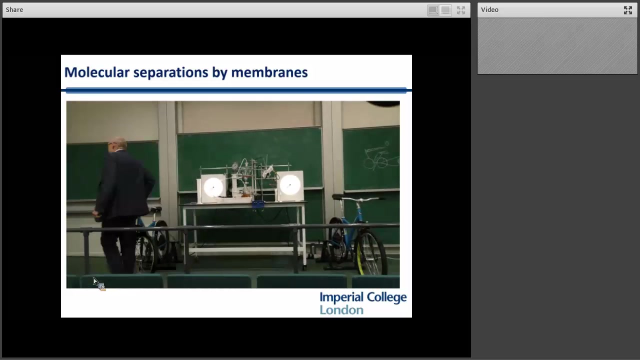 So I've got about five seconds to go. I might have to take a breather after I finish this. Here I come up for my minute. So that's how much energy it takes to produce a few drops of water using evaporation. Now that's where we have technology. So this equipment here, what I have is another bicycle. 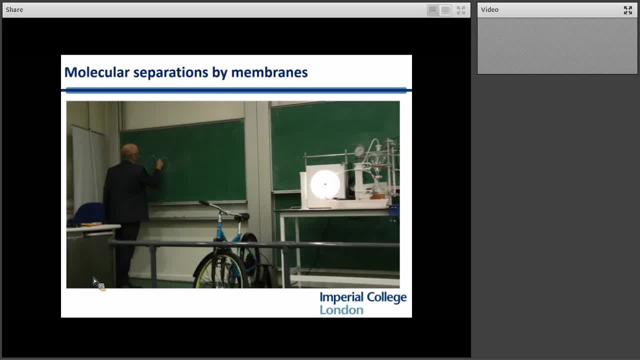 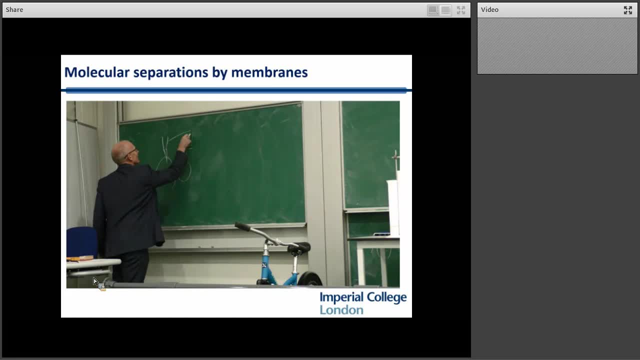 And I'm going to put on this bicycle and again I'm going to pedal, And as I pedal, the energy that I generate is going to be converted to electricity, and that electricity will now drive a pump, So I'm going to use a pump. 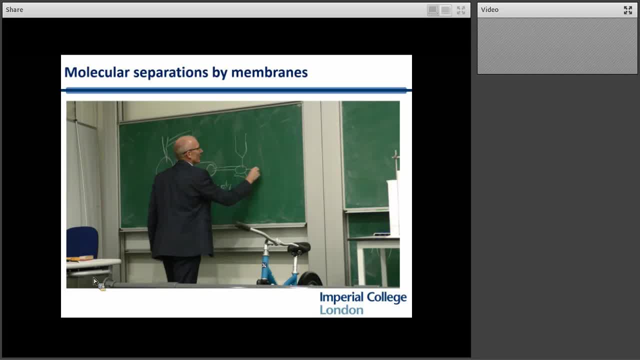 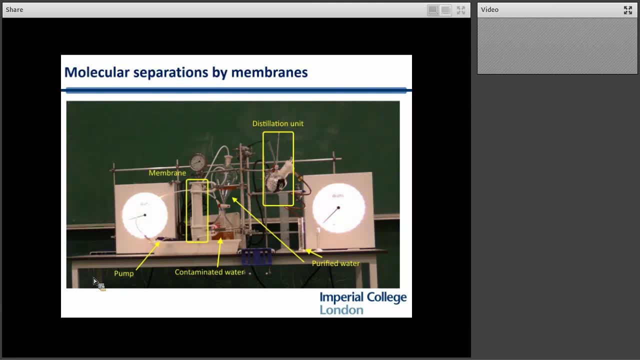 And that pump will come to the tank and it will go to a membrane module, which is this unit here. That's my membrane module and here's my pump. So as I cycle, I'll produce water here, And that water will be fresh water, the same as the water that I was producing in distillation. 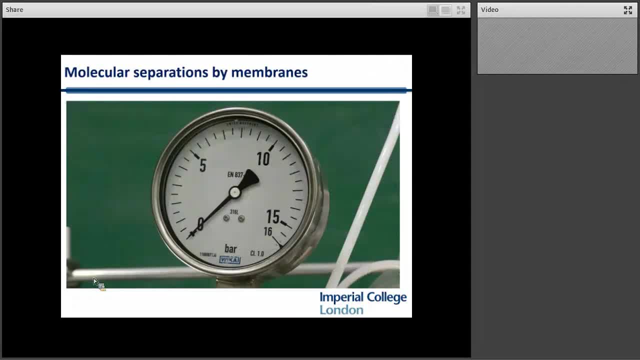 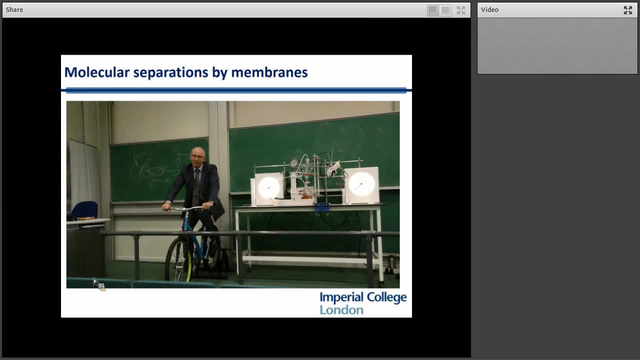 I think I've got my breath back now, So I'll get this bike up to speed. And here I think I'm going to go more gently and just go. I'm going to go for something like 50 watts. A man of my age has to watch how much energy they generate. 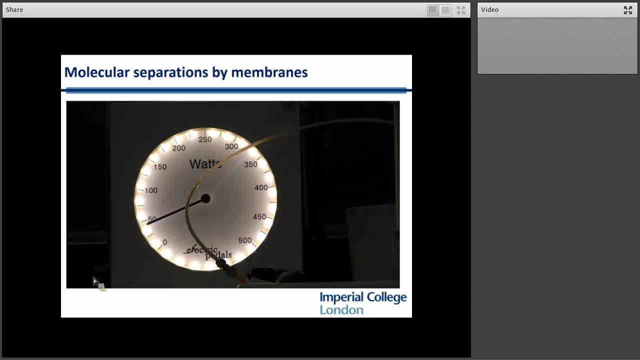 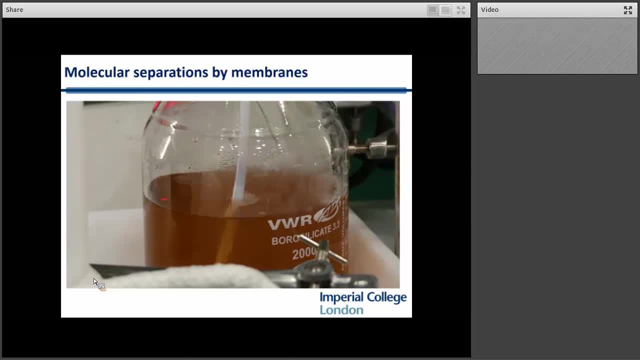 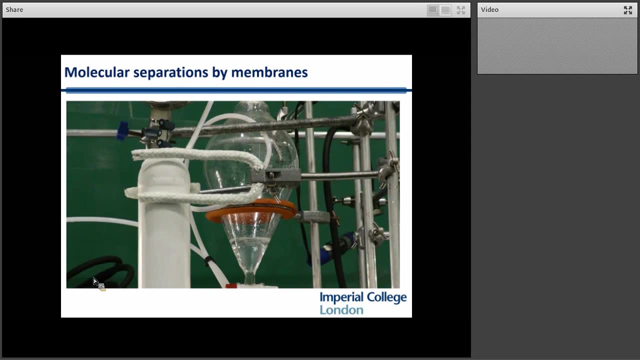 So if I start now, this is my one-minute period, So that you cruise along. I can ride no hands, even when you have a membrane, And I'm reducing 50 watts And you can see the water coming through into the collection vessel. 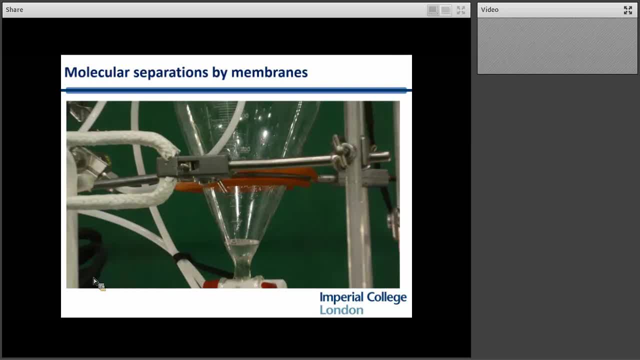 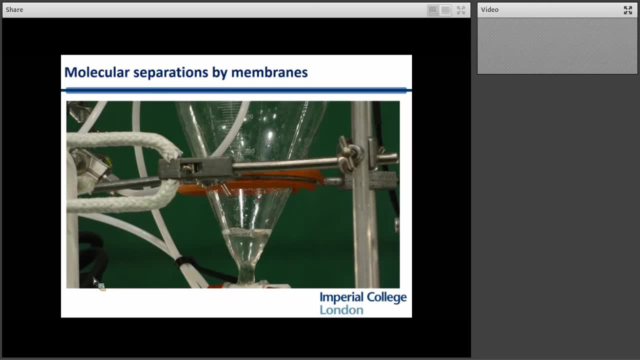 It's starting to fill up. The water's coming through. You can see, with just 50 watts the rate of water coming through is much higher. I'm 30 seconds in. I do have to say this is much more pleasant riding along with a membrane at 50 watts. 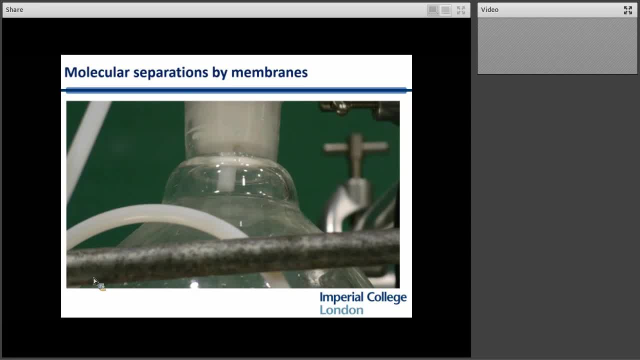 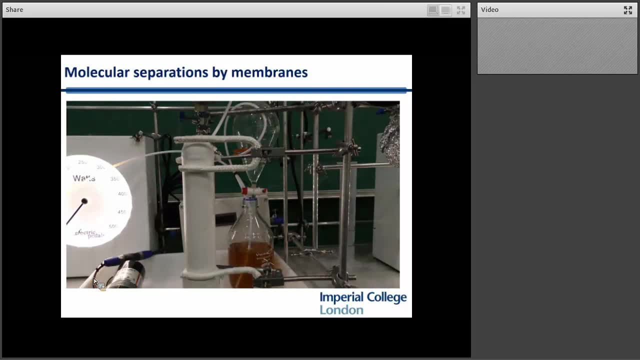 You can see the water starting to come through and building up And the point is that with a lot less energy, and the energy source has been the same in both experiments. The energy source is me And I had more energy when I started that experiment than I do now. 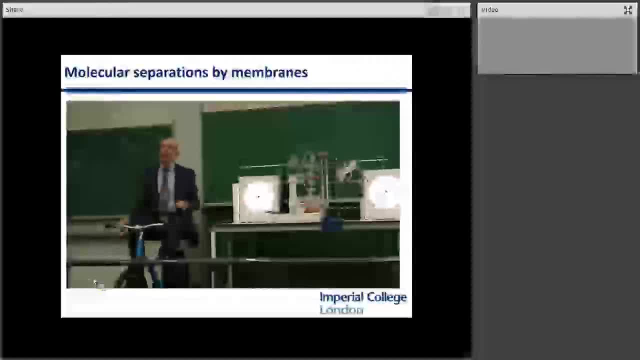 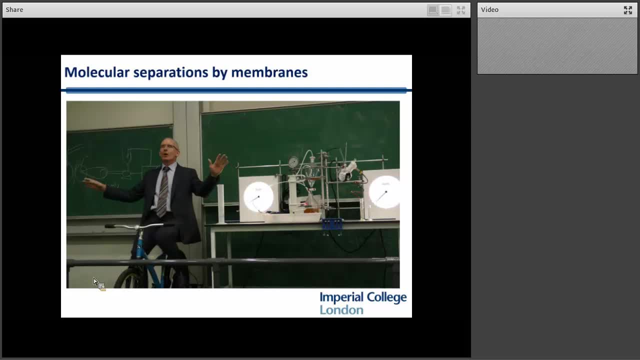 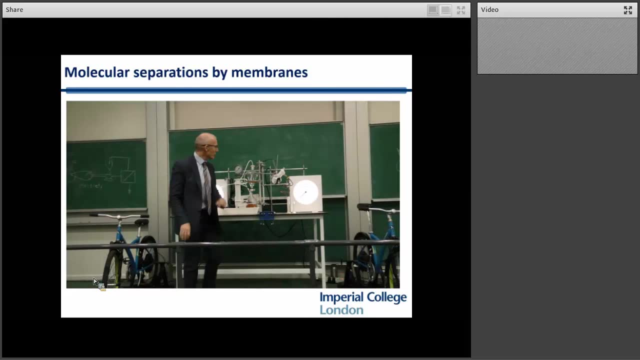 I have to bike him flat out for a minute. I'm reducing less power. I'm only reducing 50 watts. I'm already generating a lot more water. My last second, That's the membrane volume. Now let's compare how much water I've generated through the evaporation with how much water. 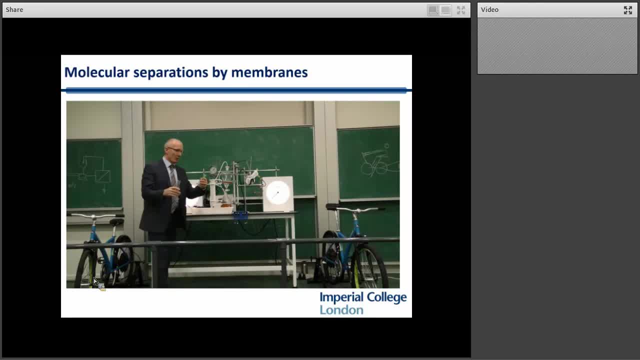 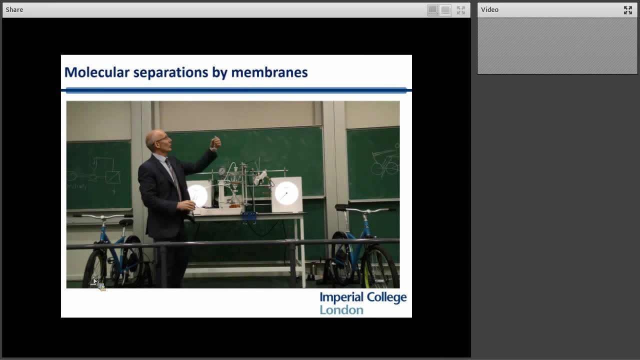 I've generated through the distillation. Well, here's the evaporation water, And this is rather a small quantity. So you put it as a cylinder. What you can see here, if you read the gradations on the side of that cylinder, is that I've 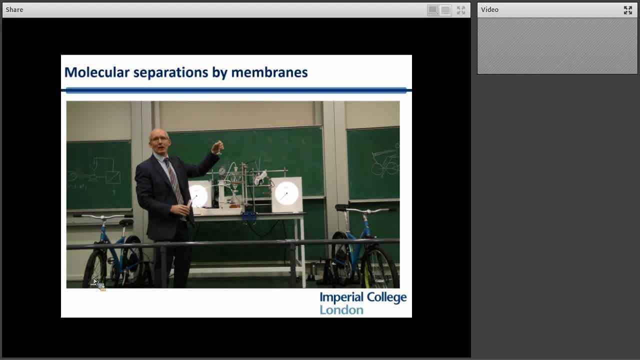 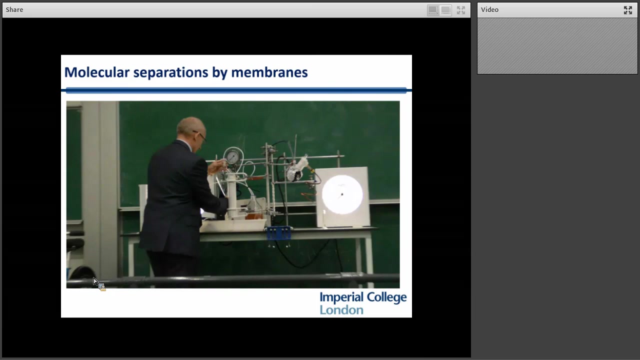 produced about two mils of water in a minute. I'm really cycling hard, producing 250 watts of energy. Here you can see the membrane rate. Here I'm going to lift this up and put the water into this mentoring cylinder so you can see it more clearly. 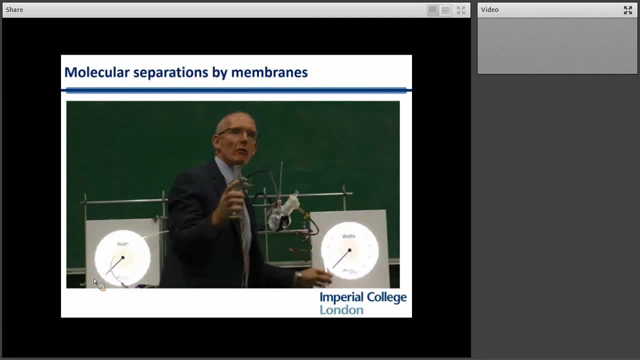 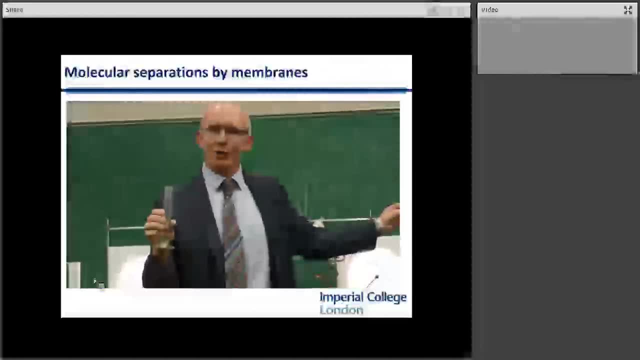 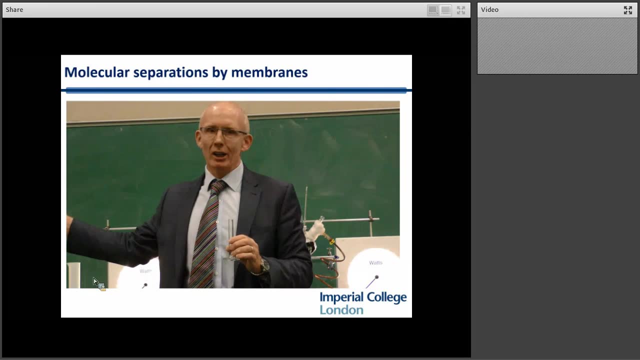 In the membrane experiment, I've generated over 50 mils of water. So what a comparison. Here, cycling for a minute at 250 watts, wearing myself out, I've produced two mils of water. Here, cycling for a minute running at only 50 watts, very sedately, I've produced over. 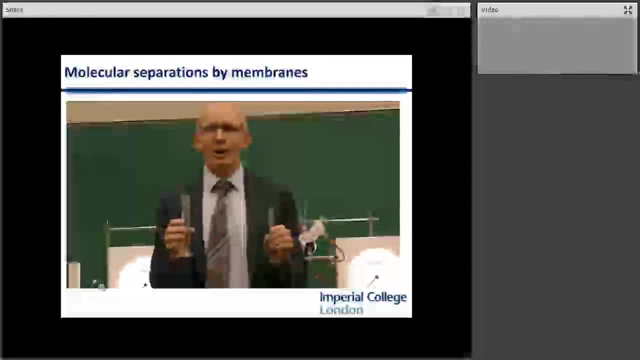 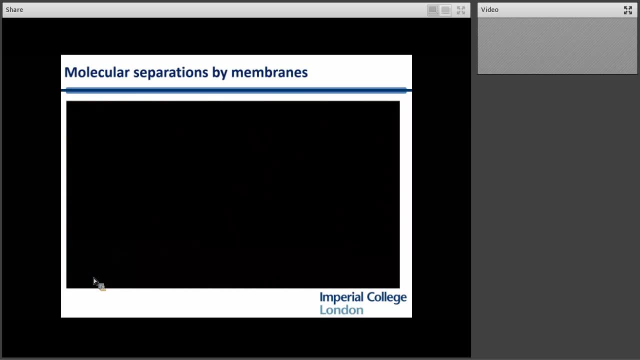 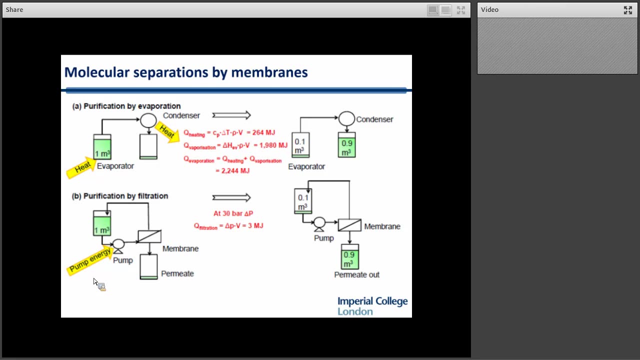 50 mils of water, And that is why membrane technology is far more effective than thermal techniques purifying water, Thank you. So you can see that using membranes you can, with a lot less energy, purify water, And I just want to take you through why that is in terms of the numbers. 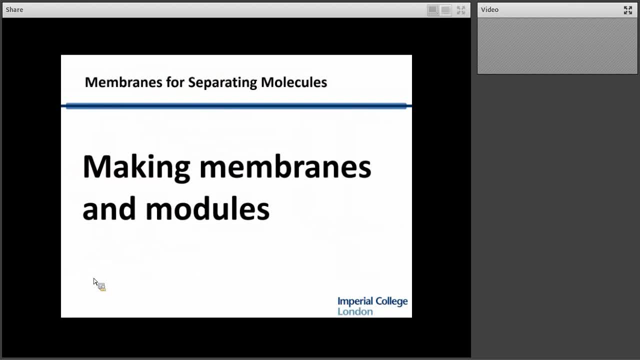 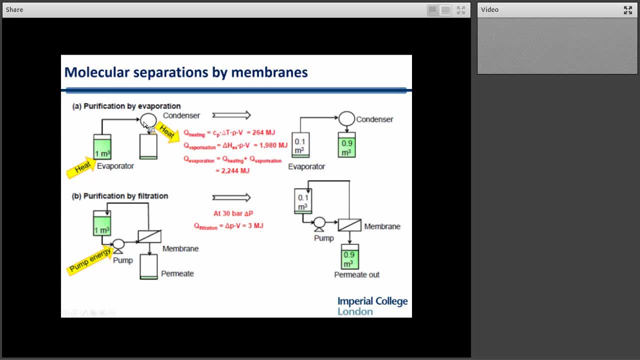 If you think about what I did, I was just using an evaporator to produce heat, which was used to evaporate water and then condense that water. And so if I consider a meter cubed of water and I say that I want to, it's got salt in. 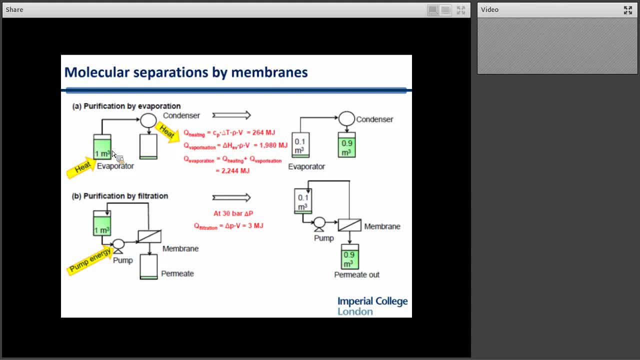 it. so I'd like to evaporate it and then condense it, to recover it as pure water. then it's not pure water. Then if I want to do that, I'm going to have to heat it up. And you can see an amount of heat here: 264 megajoules required to heat it up. 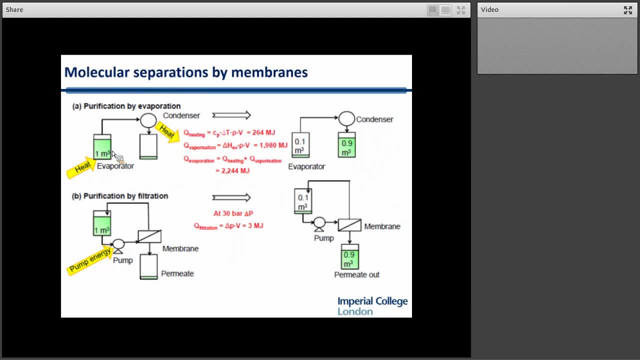 And then we're going to have to vaporize it And that takes me 1,980 megajoules And if I put both of those together and I spend 2,244 megajoules, I can evaporate and then condense 900 litres or 0.9 metres cubed of water. 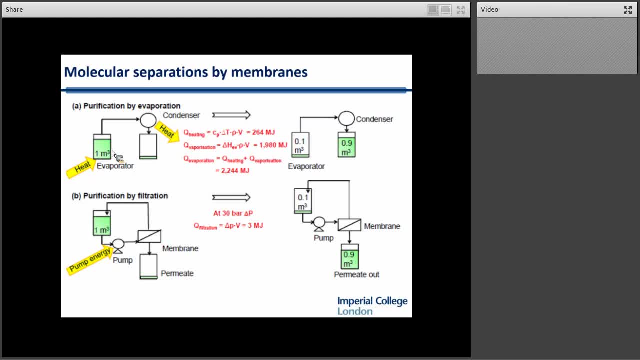 So that's a lot of energy. If I sit on a bicycle and use a membrane and then evaporate it, that's a lot of energy. And then it drives a pump and I put pump energy in in the form of electricity and then I 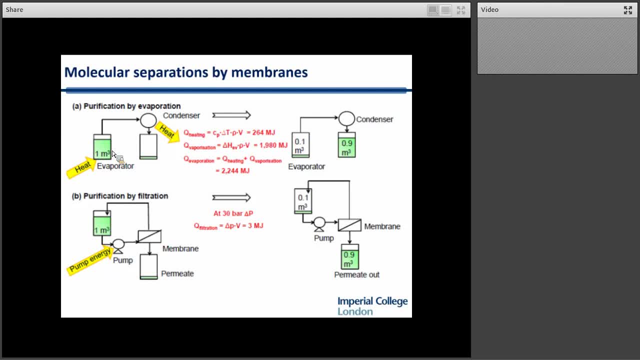 have to run at a pressure drop of 30 bar. If I move the same amount of water through the membrane- 900 litres or 0.9 cubic metres- that takes 3 megajoules. So that's something like nearly three orders of magnitude less energy to produce the same. 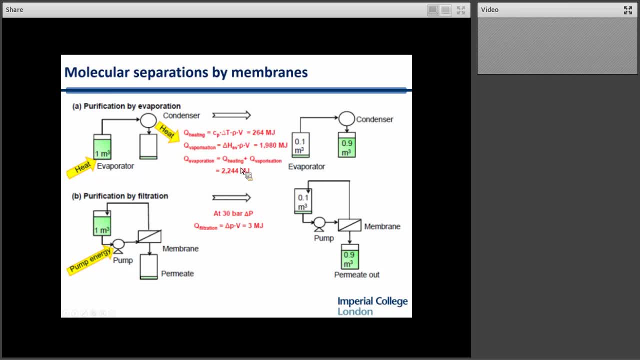 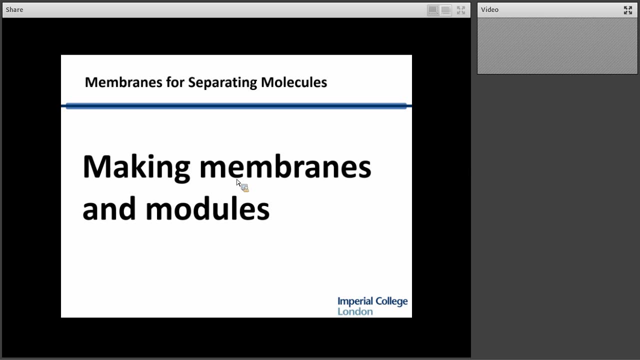 amount of purified water using a membrane than it would take me by using evaporation, And that's why membrane technology is far more effective than evaporation And evaporation for purifying organic liquids and for doing things where you need to separate a volatile organic liquid from other solutes. 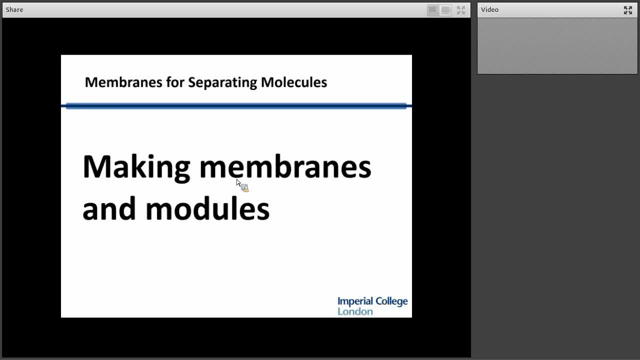 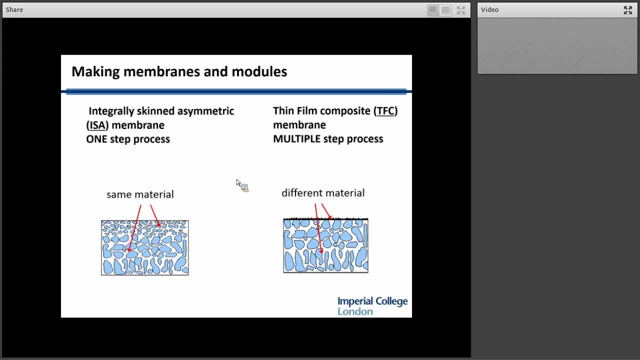 So to do that, of course, we need membranes, And what I want to tell you a bit about now is making membranes and modules. There's two types of membranes that we use. The first type is made out of one material, here on top of a non-woven. we call this an. 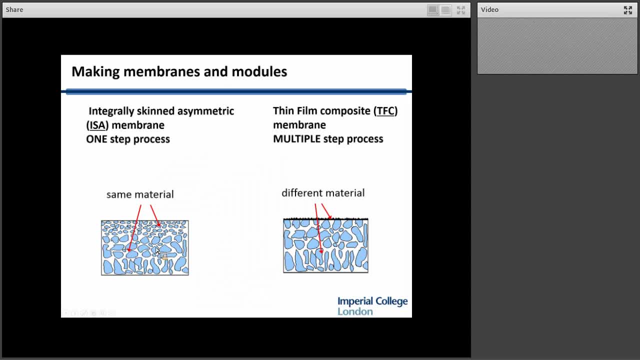 integrally skinned asymmetric membrane. So the point is, the open part of the membrane here and the more closed part of the membrane that carries out the filtration here are all made of the same material. Then the other type of membrane is what we call a thin film, composite, because it has 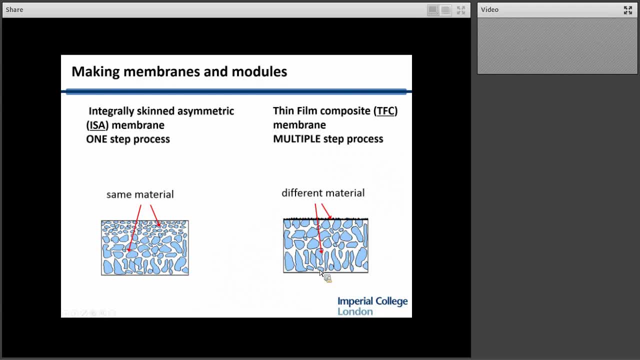 a thin film separating layer on top of a more open membrane material down here. So we make an open membrane and then we coat it. So just a bit about how we do each of those, starting with this integrally skinned membrane. This video shows you membrane casting on a bench top casting machine. 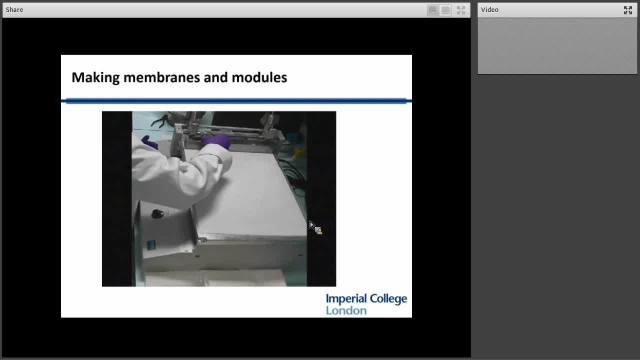 So we start with this, what we call dope material. It's about the consistency of the membrane. We have honey, So it's a brown solution. It looks like honey. What it really is is a polymer dissolved in a solvent, for example DMF or DMSO or a solvent. 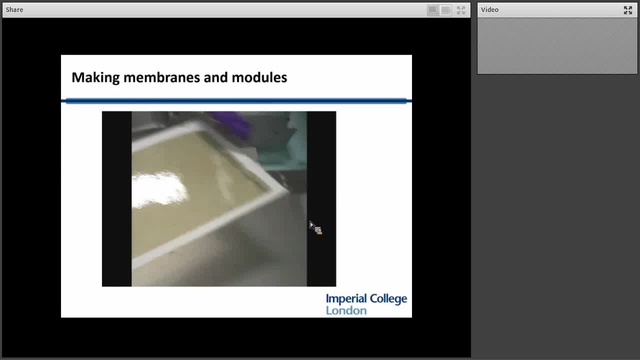 like that, which will dissolve the polymer. We make this thick, gooey dope and then we cast it to a fixed height on top of a non-woven backing, which is like a piece of paper, and then we dip it in water. 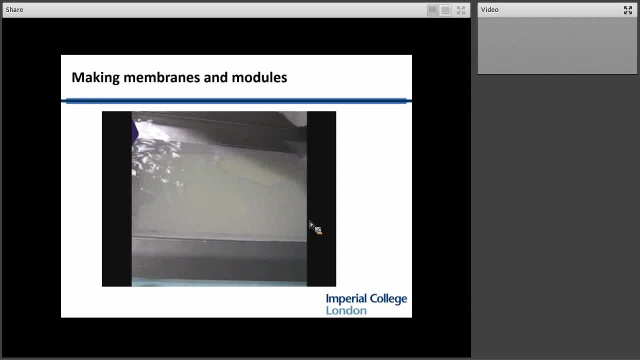 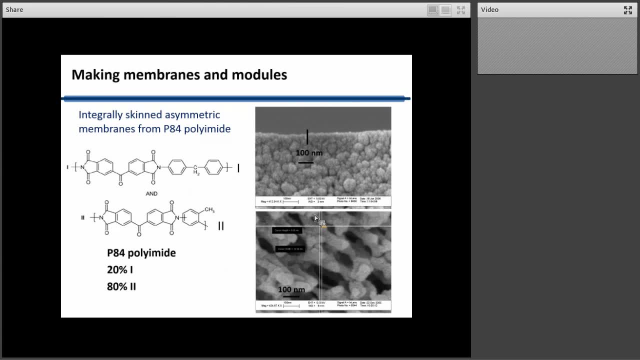 And when we dip it in water, the solvent comes out of that polymer solution and the polymer precipitates on top of the non-woven and we get a membrane that looks something like this. So what you can see here is the very top separating layer of membrane made from this. 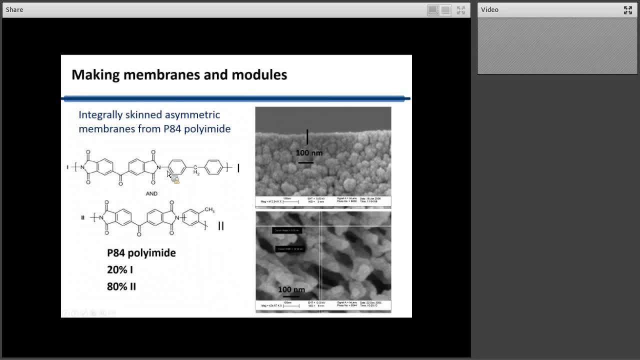 polymer, which is a polyamide, made up of these two polyamides. When we do this phase inversion process, the very top layer of the membrane has these finely divided clumps of polymer, and it's the gaps between these clumps of polymer that gives 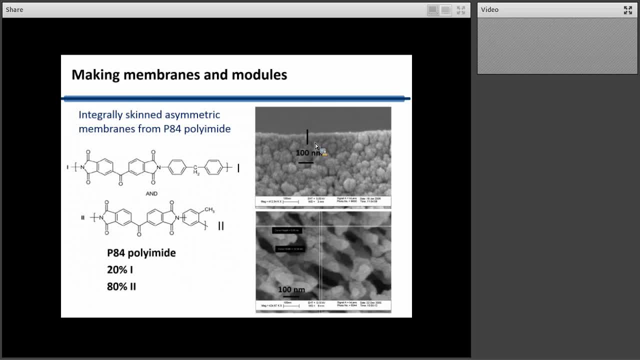 us pores and allows us to separate molecules Through most of the thickness of the membrane. it's far more open, So we get a very open structure which doesn't provide much resistance to flow. So that's asymmetric: Thick at the top and much more open at the bottom. 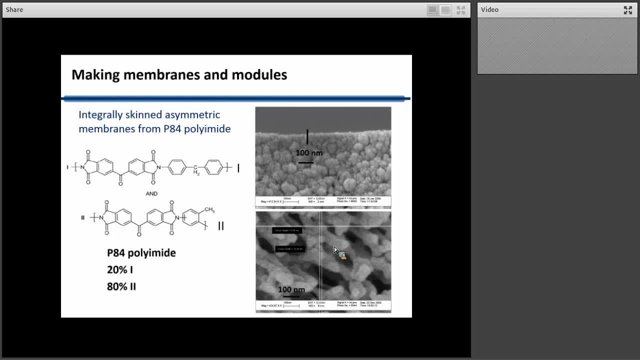 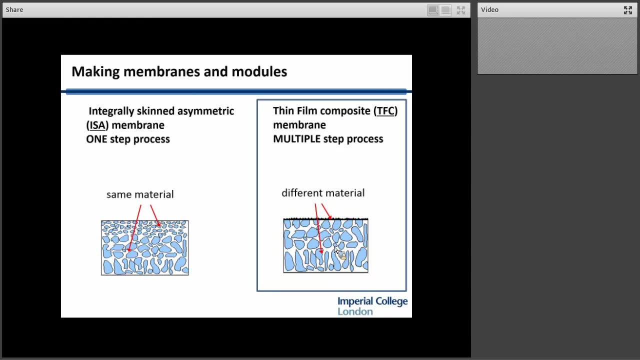 And we can use that to filter liquids and remove molecules from them. The other type of membrane, the thin film composite, is a bit more complicated, So we have to start off by carrying out the same process of phase inversion, but now to make a more open support membrane. 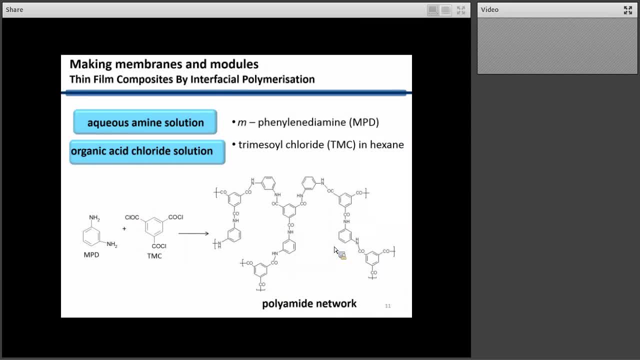 And then on top of that open support membrane we carry out a reaction which gives us a very thin film, And typically this reaction is between an aqueous amine solution and an acetic acid chloride in an organic solution. So typically we'll use metaphenylenediamine, or MPD, and trimethyl chloride. 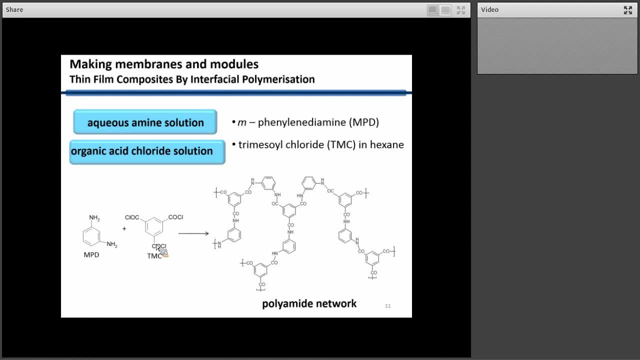 These are the two most common ingredients of reverse osmosis membranes, And this one is present in the organic phase and this is present in an aqueous phase And they react together to give us this networked polyamide layer here. And so the way we do that is we start off with this open, porous support and we impregnate. 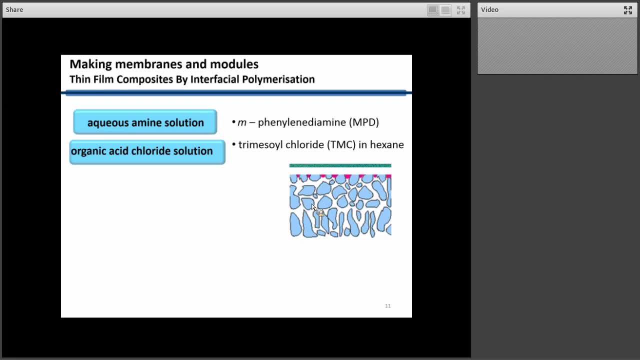 it with the aqueous solution of the amine and we then contact that with the organic solution of polyamide And that's the solution of the trimethyl chloride, And they react together to give us this polyamide layer, a very thin layer at the surface of. 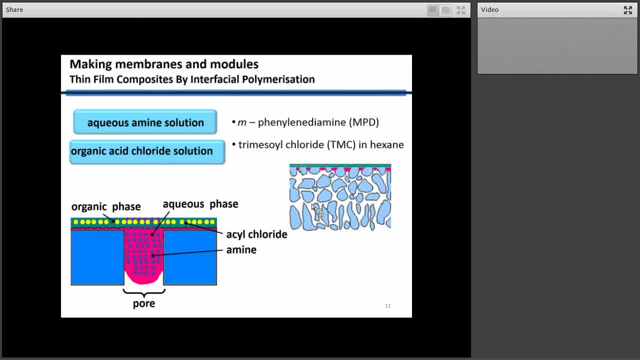 the membrane And it's that polyamide layer that provides the selectivity, For example in reverse osmosis, that doesn't let salt pass through the membrane but will allow water to pass through the membrane. So we have two different ways of making membranes. 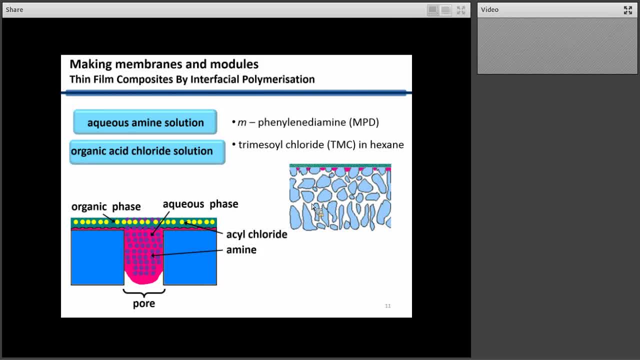 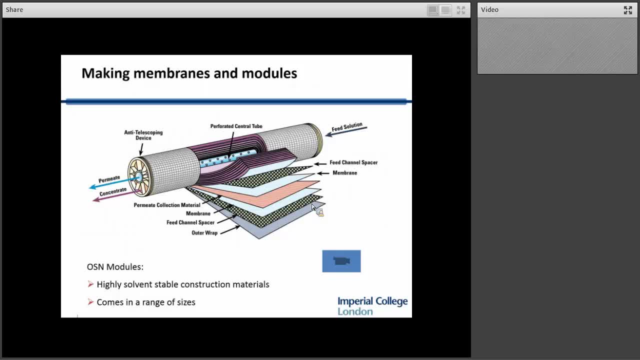 One step. we do it with phase inversion to make an integrally skinned, asymmetric membrane, And then a multiple step process. We put thin films on the membrane. But whichever way we make the membranes, what we end up with is big rolls like rolls of. 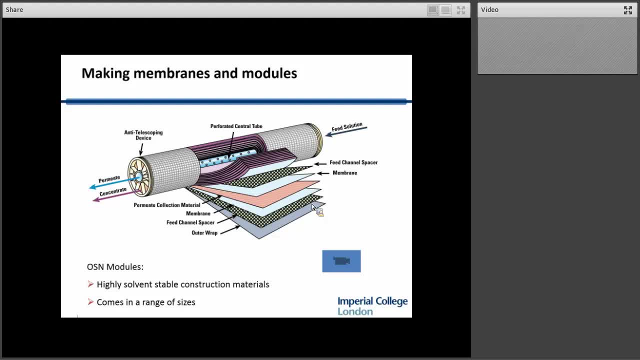 paper And we need to then use these to make membrane modules, And the most common way we do that is using what we call a spiral wound membrane module. So you can see here a perforated central tube And what we're going to do is to wrap leaves of membrane around that perforated central. 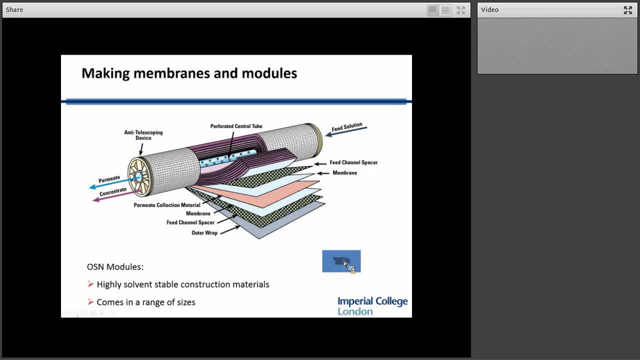 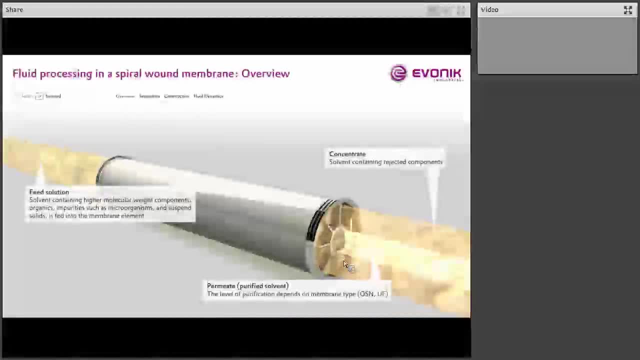 tube. Now it's quite hard to see how those things actually work, So I'm going to show you, with the aid of this video, how the spiral wound membrane module works. The feed solution actually flows in to the membrane module and it flows down between. 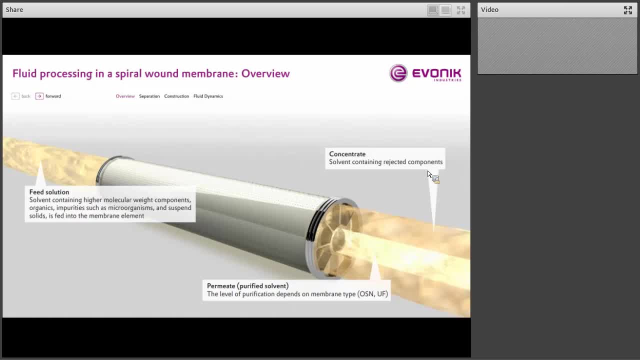 the leaves of the membrane, So that comes out as a concentrate, The purified liquid, for example water- if you're desalinating salt water comes out through the central permeate tube, And so the way that works, if you look into that module, is we have a series of leaves. 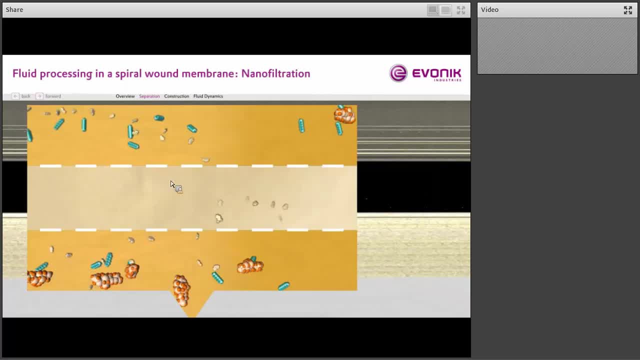 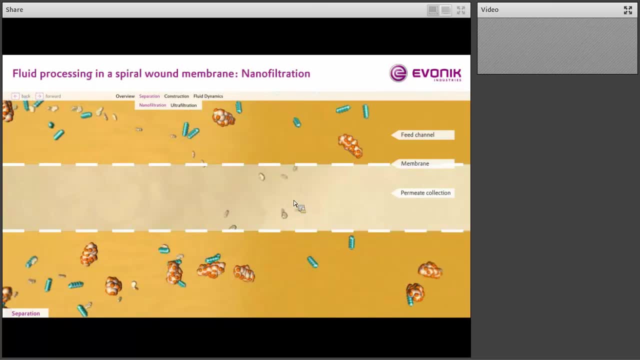 And in each of these leaves we have a permeate module. This is the membrane here and here, and then this is what we call permeate side or permeate collection, And that flows down and into that central permeate tube. 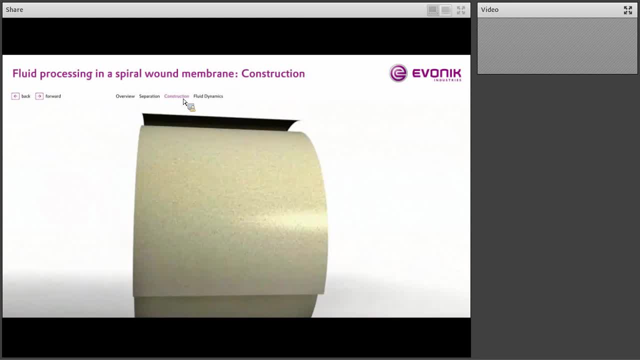 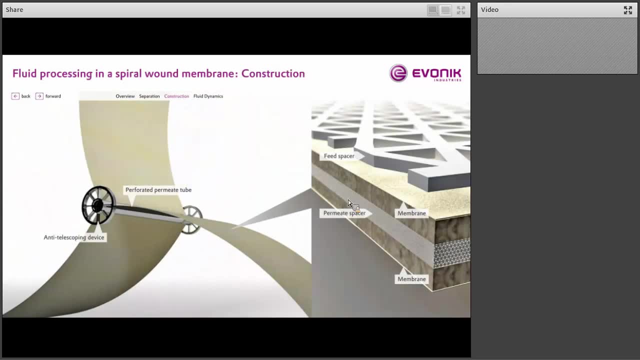 So to construct that, what we do is we take a whole series of membrane leaves, And each one of these membrane leaves is hollow, So it's a membrane on both sides. So what you've got is a permeate spacer and you've got a membrane on each side of that. 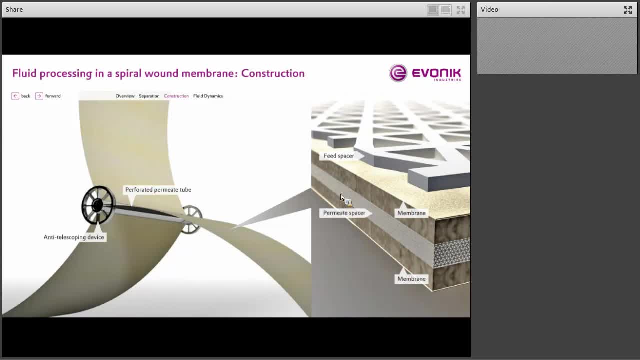 so that each one of these leaves has a membrane and a permeate spacer. There's a membrane, then a permeate spacer and then a membrane. So as fluid pushes down into this membrane, it goes through the membrane. it will then pass down through this permeate spacer until it reaches this perforated permeate tube here. 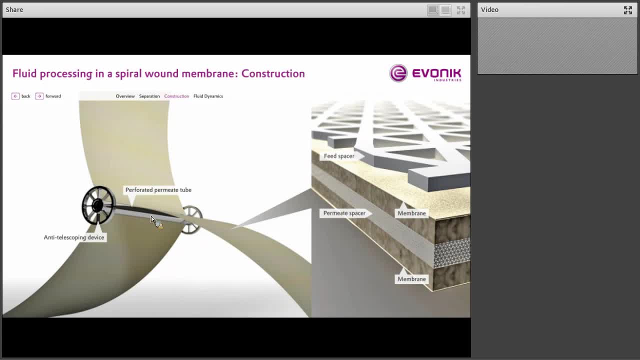 in the centre When we wrap that up. of course, we don't want the feed side of the membrane to touch one membrane, to touch the other, because if this membrane touches this membrane, there won't be any room for flow. So what we do is we add a thing called a feed spacer that holds these different leaves apart. 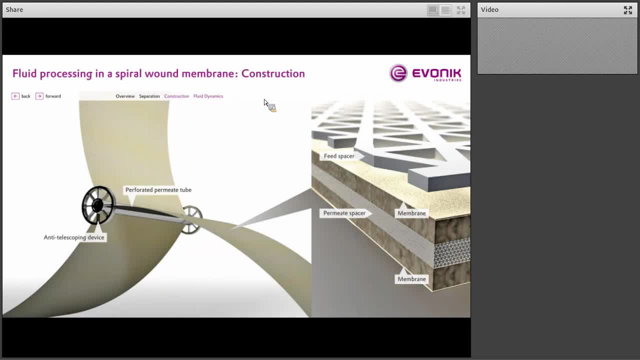 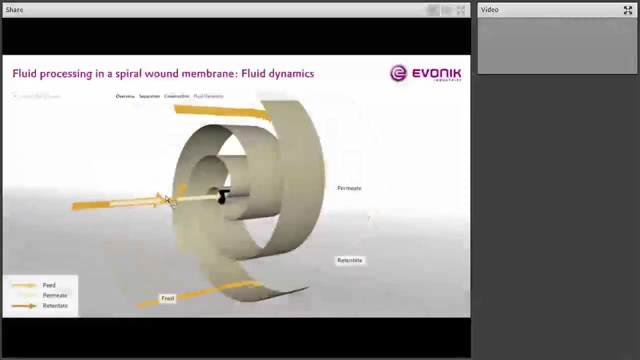 and stops them from crushing together and allows flow to pass down the module. So, in terms of fluid dynamics, when we pass flow through the membrane module, we're typically feeding a flow in this direction And that flow is then passing into the permeate side of the membrane leaf, going into the 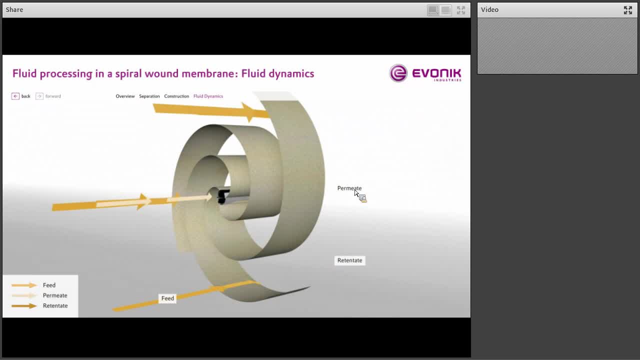 permeate tube and flowing out the permeate tube. So you can imagine it as a Swiss roll where the process fluid is passing down where the jam goes. in the Swiss roll, The fluid that you are collecting, the permeate fluid, is going through the membrane. 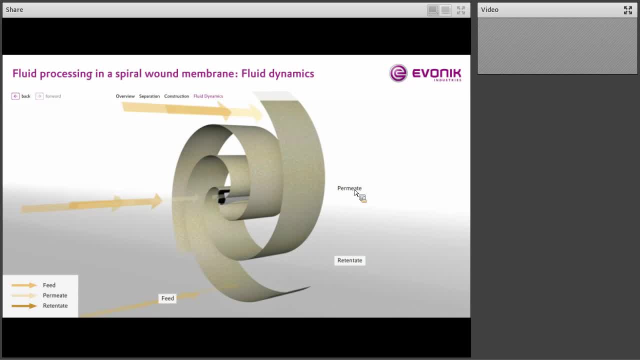 The permeate is going into the inside of the sponge and coming around to the middle of the Swiss roll and flowing out. So this is the most common type of membrane module that is used in liquid separations. So what we do when we have these membrane modules is we take them and we put them into. 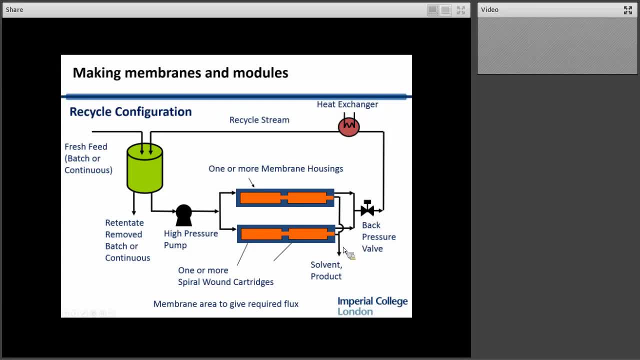 what we call membrane housing. So a typical membrane plant will have a few key components. One is a high pressure pump. You need a pump using electrical energy to push the fluid up to the operating pressure. A back pressure valve that holds the pressure. 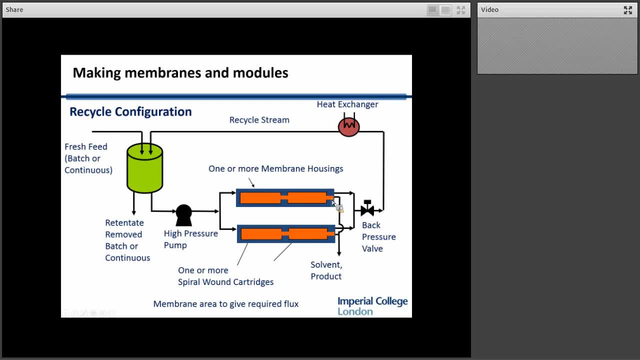 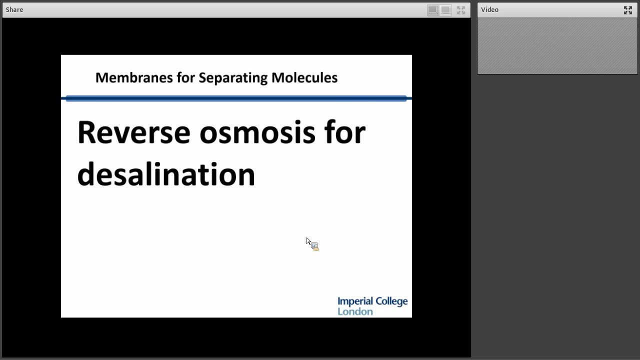 It holds the pressure on the membrane housings And in each membrane housing, which is essentially a pressure vessel, a number of membrane modules that carry out the processing. So that's a bit about membranes and membrane modules, And what I want to do now is to touch on the first application I want to mention, which 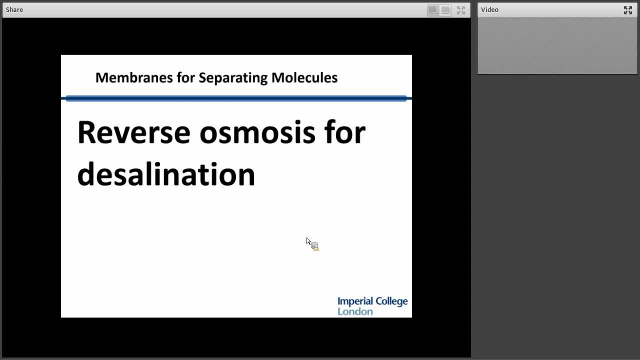 is reverse osmosis for desalination. So in reverse osmosis what we're doing is taking a salty water and we're applying pressure to it and contacting it with a membrane so that the water will pass through the membrane And the salt is held back by the membrane. 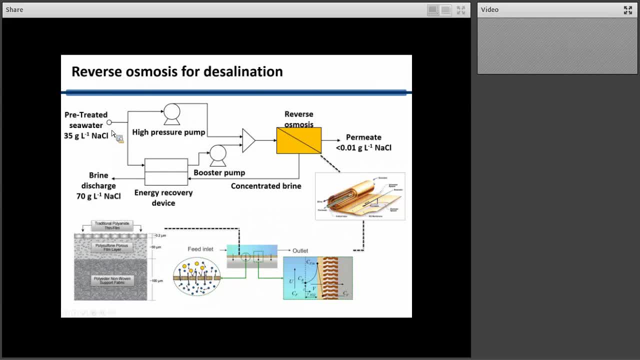 This will be a classic layout for a reverse osmosis plant here. If you have seawater, you'll typically pre-treat that to remove algae, bacteria, slime and everything else, And you'll have a dissolved solution of salt, typically 35 grams per litre of sodium chloride. 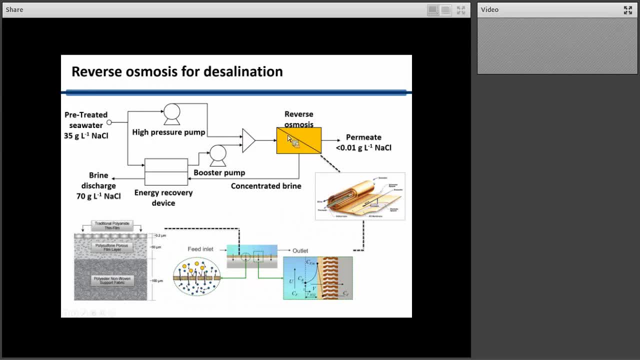 You'll put that through a high pressure pump and pump it against the reverse osmosis membrane module. Some of the water will pass through the membrane. That's the permeate with a low salt concentration, And in some of the water it will pass through. 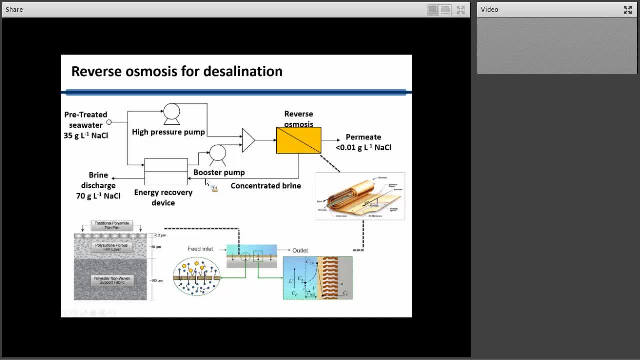 We'll be returned as a concentrated brine. Of course, this is still under pressure And so generally, in the interest of energy efficiency, we'll try and recover the pressure energy from that recovered brine which we'll take out here. 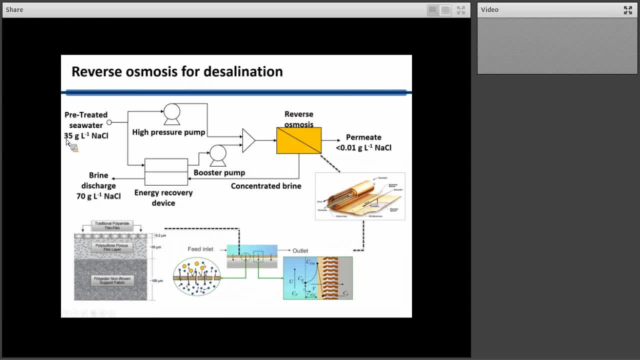 And you can see that typically I would double the concentration of the salt from about 35 grams a litre to 70 grams a litre, which means I'm recovering about half of the feed seawater as low salinity fresh water. And of course, to do that I use one of these spiral well membrane modules. 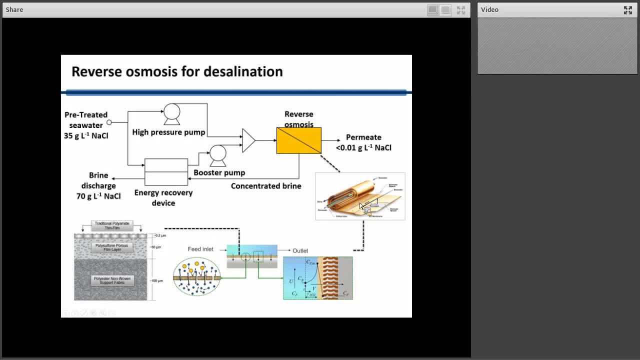 And that spiral. well, membrane module is made up of a whole lot of leaves rolled around a permeate tube. If you look at the level of the individual membrane, there'll typically be a layer near the surface of the membrane where there's concentration gradients because the water 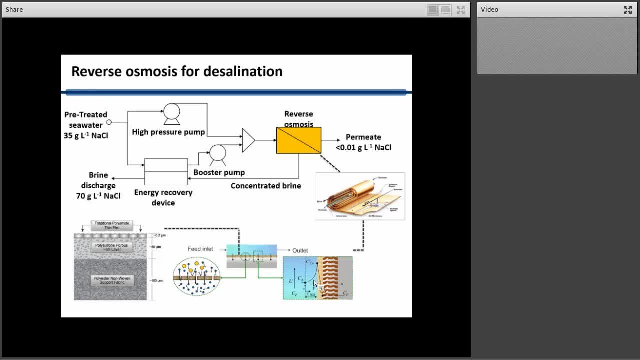 is passing through the membrane. We call that concentration, polarisation- And at the very separating layer of the membrane, what you've got is water passing through and salts hopefully being rejected from the membrane. As I alluded to, this is a thin film composite, so we'll have a non-woven material that we 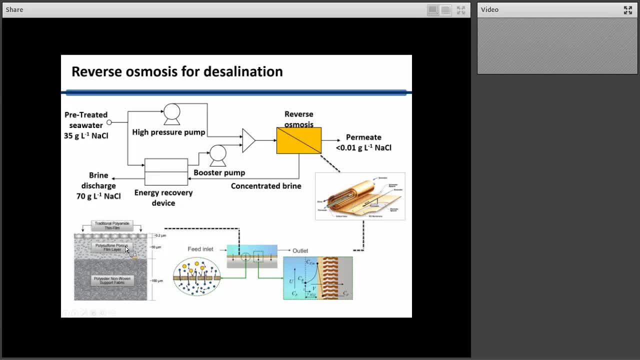 use to cast an open membrane on using phase inversion and then a traditional polyamide thin film. Now we've done an amount of work on this under the BP iCAM project with BP, And the reason this is interesting for the oil and gas industry is it turns out that 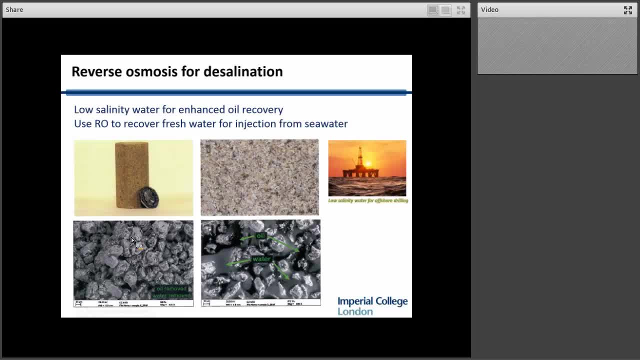 one application of desalination is to produce fresh water which is then used to inject into rock structures. And you can imagine that when you have oil in a rock structure- and this picture here shows you water and oil in a rock structure, Then the way that the oil and the water hang onto the rock or interact with the rock is 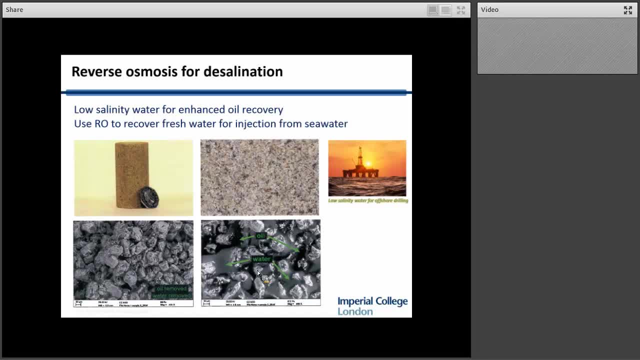 key in determining how much oil you can extract from the reservoir. So if you can make it so that the oil will more easily come out of that rock structure, you'll get a higher oil recovery. And enhanced oil recovery can be worth literally billions of dollars in an oil field. 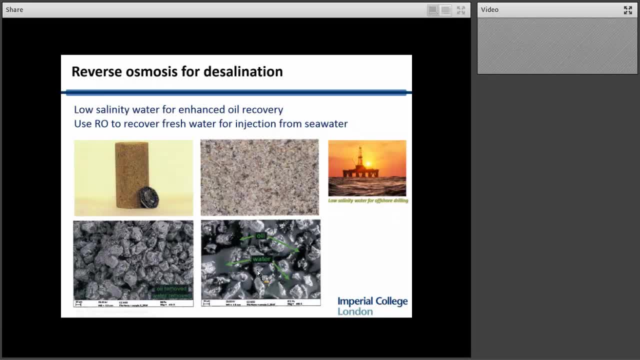 It turns out that research in BP has found out that if you use fresh water to inject down the well, to repressurise the well, then that fresh water is going to come out of the well And that fresh water means that the oil more readily lets go of the rock and comes up to. 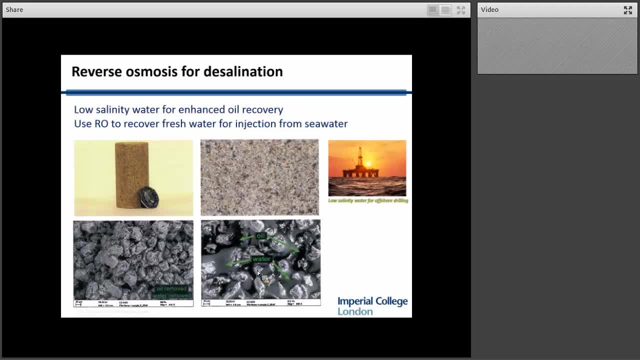 the surface. So by injecting fresh water down an oil well, you can recover more oil, And so there's an interest in desalination of seawater for use as injection water. And if you look at the state of the art in desalination, I think the current challenges 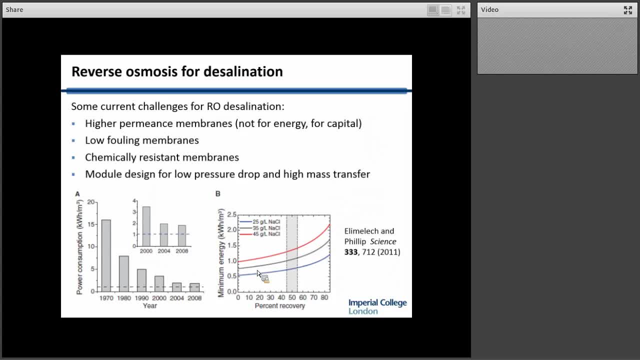 for reversal, osmosis, desalination, very simply put, are here. So one thing people are looking at is higher permeance membranes, In other words, getting more flow through a given membrane area. Now there's some confusion around this, because some people think that if they have 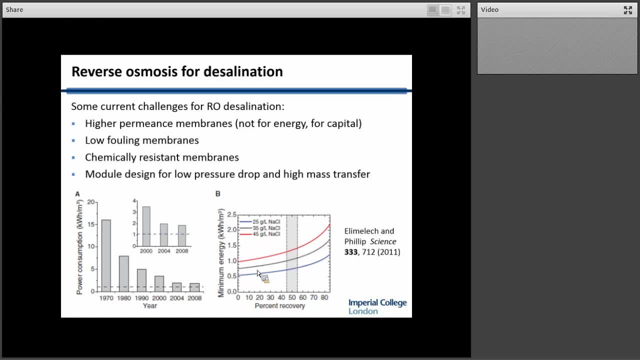 higher permeance membranes. it's going to reduce the amount of energy that we need for desalination. There's a very good paper in Science from the Alignelic group at Yale which points out that isn't going to happen. So the amount of energy that we need to desalinate water has gone down the last three decades. 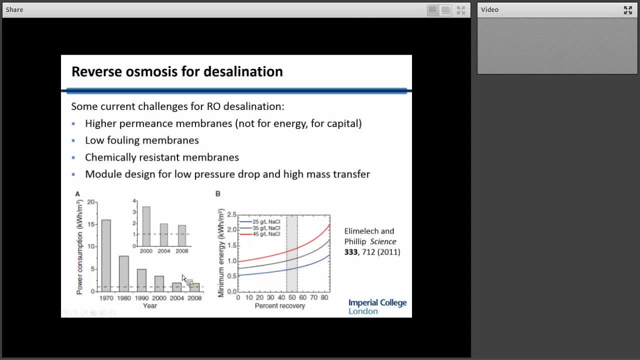 from up over 15 kilowatt hours per metre cubed down to around two kilowatt hours per metre cubed. The theoretical minimum amount of energy you need for water desalination will depend on the amount of water you recover and the starting salt concentration in the water. 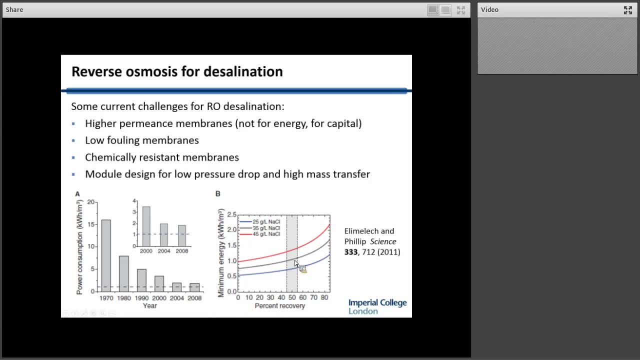 But as a midpoint, the theoretical minimum amount of energy you'll need is a bit over one kilowatt hour per metre cubed, So actually we're just under two now. We're quite close already to the theoretical minimum amount of energy we need. 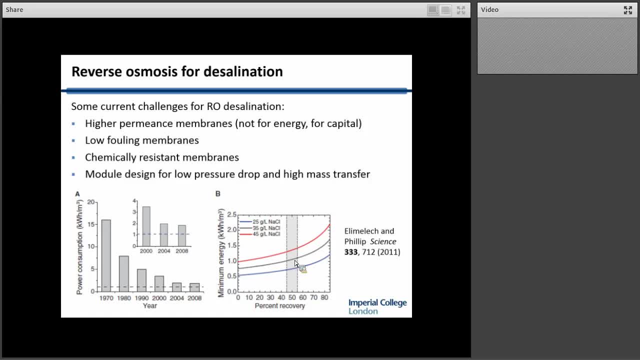 So the real reason that we might be interested in higher permeance membranes is because we'll need less membrane area for a given installation. And if we need less membrane area and we're working in an offshore environment, for example to produce water for reinjection, then the weight or the size of the membrane plant 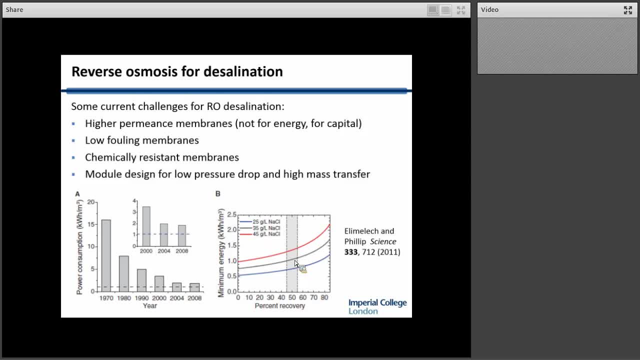 can be very important in its overall cost effectiveness. A couple of other key considerations in reverse osmosis currently are how we go about producing low fouling membranes, Eventually reverse osmosis membranes foul with biomass or scale. how we can produce chemically resistant membranes that we could more readily clean or sterilise. and also 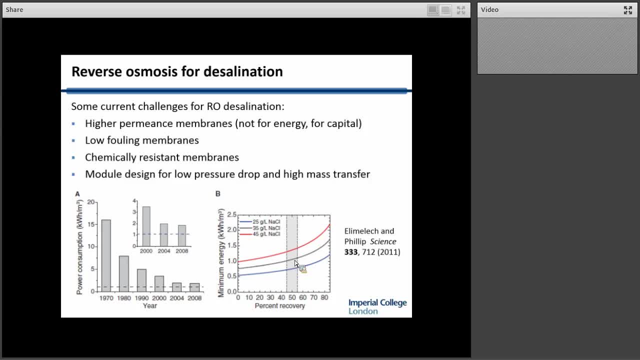 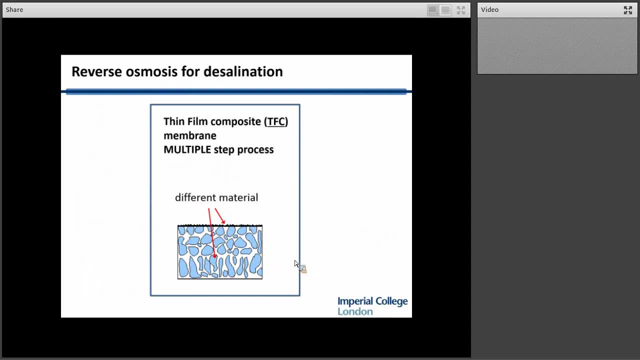 how we can produce modules with lower pressure drops and high-mass membranes. I'll come back to that at the very end of my talk. But one way of trying to develop better membranes, of course, is to understand how the membranes we have work. 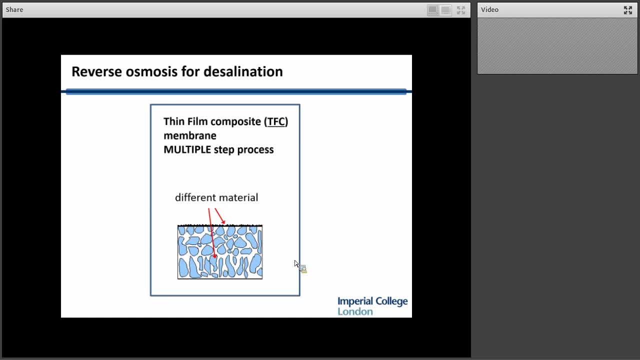 And in the next few slides I'm going to be talking about thin film composite membranes made by this multiple step process that I talked about before. So there's going to be a support layer and then a thin film layer on top of the membrane where the separation is affected. 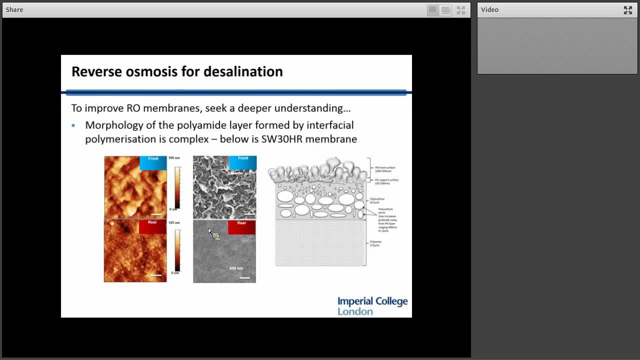 Now the interesting thing is, when you look at these membranes- and I've showed you a diagram that shows them more or less as flat membranes- They're flat sheets on top of the support- When you look at these membranes under electron microscope or using atomic force microscopy- 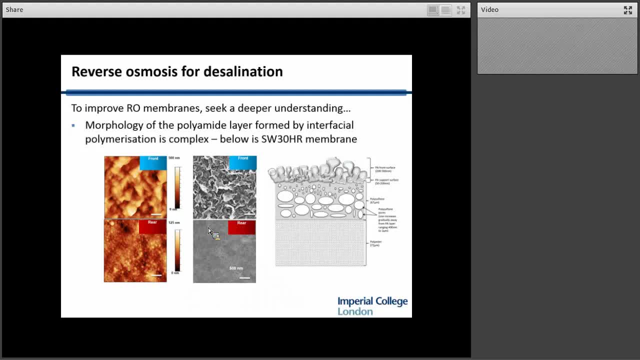 so you can see here on the left electron microscopy- sorry, atomic force microscopy, and in the middle we have SEM. they're not flat So they actually turn out to very complex morphologies. So if you look down at the surface of one of these membranes, there's actually all sorts. 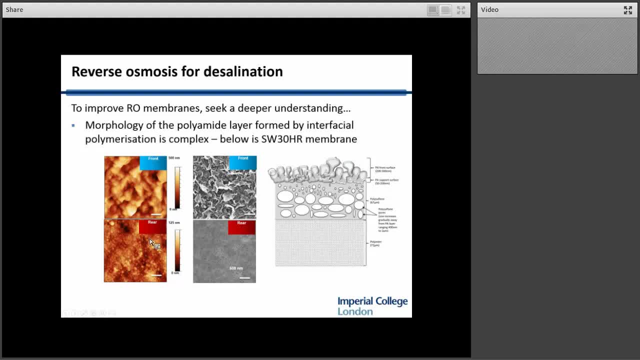 of things sticking out the top of it, and if you look at the rear side, the back side of where the film is, that's much smoother Under the SEM. here you can see what's happening. Here we have all sorts of ridges and in fact this is called a ridge and valley structure. 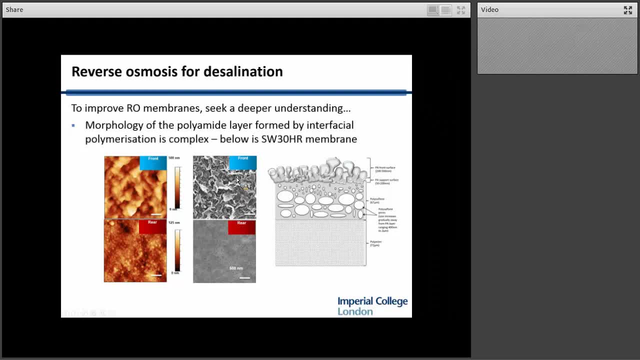 This structure isn't what you think it's going to be. before you look at it, You think you're going to get a nice flat polyamide film through which permeation occurs, and what you really have is a polysulfone layer on top of a polyester support. 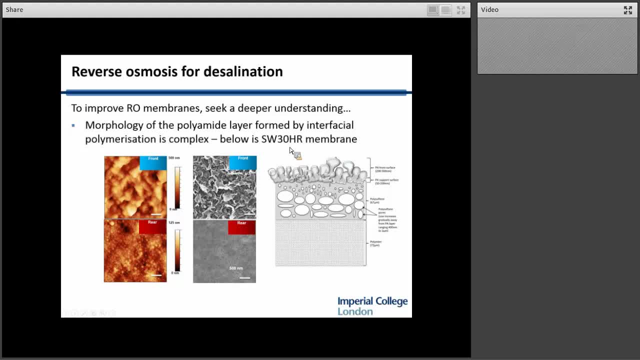 This is an SW30 HR membrane, which is a membrane made by Dow Film Tech, and what you can see here is we have this very complicated structure, and the question is: how does that structure impact on how we do research? How does reverse osmosis and how does reverse osmosis perform? 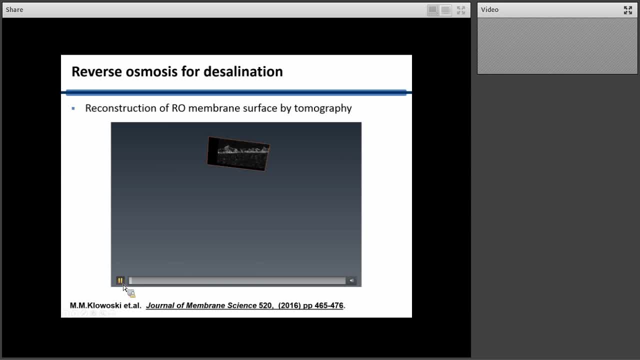 So a key thing in figuring that out is to try and understand that structure and with colleagues in the materials department we've worked on using focused IMD milling to chop sections of one of these top layers of these membranes- reverse osmosis membranes to go. 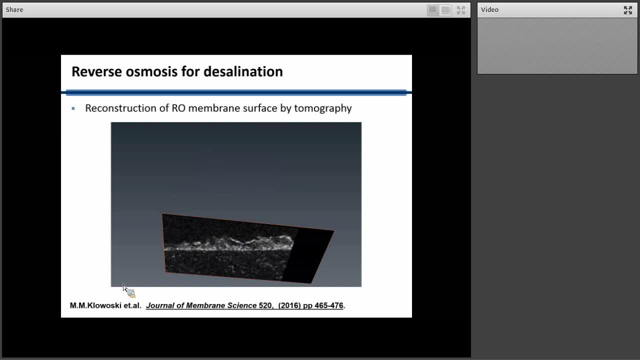 through it and cut sections out of it, then to analyse each of those sections under a high-resolution SEM and then by using tomography to reconstruct those slices and come up with a picture of what the ontology looks like. So you can see, as you saw in the SEM, that we can now get a physical representation of 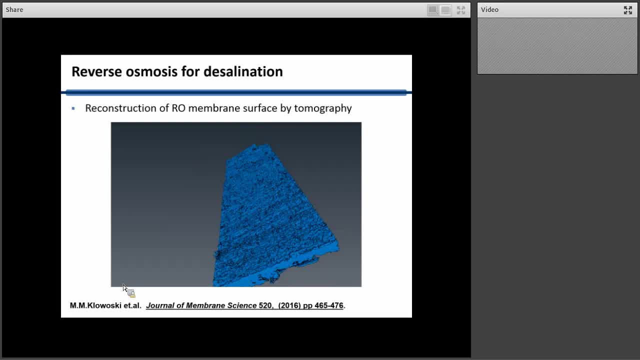 this membrane in terms of the structure and the morphology on the top layer and on the back side of the membrane, And obviously we're interested in a bit more detail in that. so what we can do for each of those slices is look in each cross-section how the surface of the membrane looks. 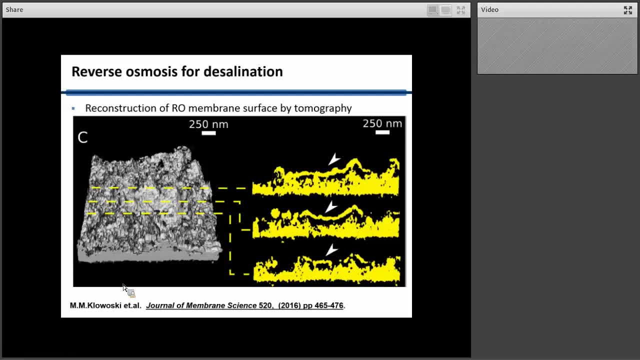 And I think there's one word for that, which is it's complex. So the membrane looks quite complicated. so how do we go about trying to describe how we can transport through a membrane where you've clearly got different layers, you've got these leaves, you've got protuberances sticking out and so on? 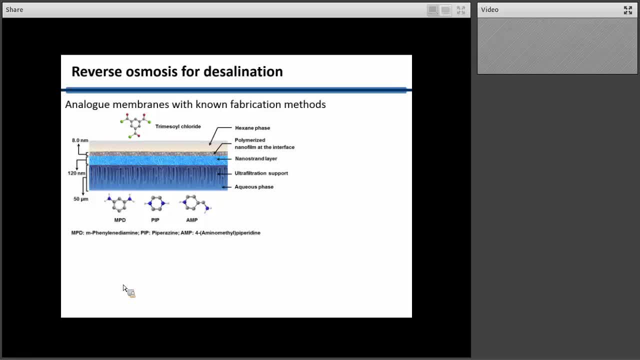 So the way we have approached that problem is to make our own membranes, because the commercial suppliers of membranes, for very sensible reasons, generally won't tell you exactly how they make their membranes. That's a commercial secret. So you know they make a membrane, you know that it works for reverse osmosis and you 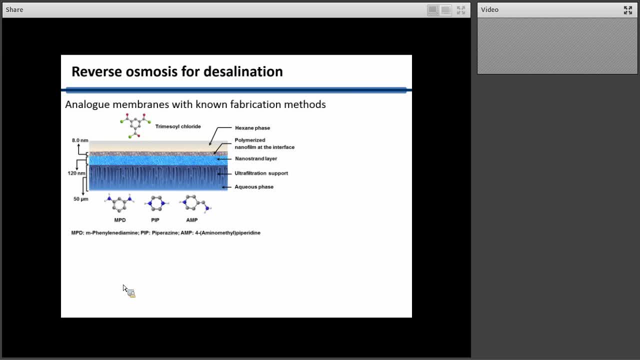 can study it by doing electron microscopy and so on. but if you want to try and change the chemistry, you can't really do that. You don't know how they've made it. So we decided to make our own membranes, And one of the challenges was how we would manipulate the morphology of that membrane. 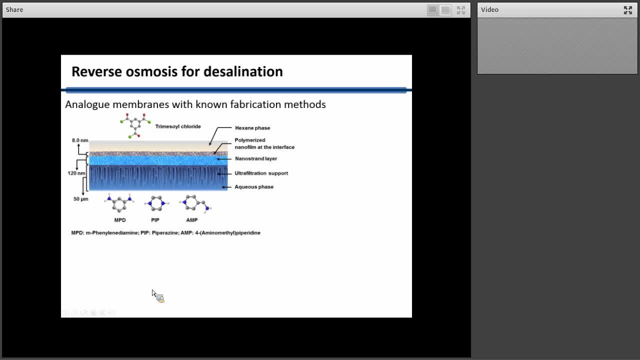 And what we did in order to do that was to take a rather unusual fabrication technique which was known in literature but not widely used, and that was to make cadmium hydroxide nanostrands, And we use these in a layer here, so we filter a very smooth, flat layer of cadmium hydroxide. 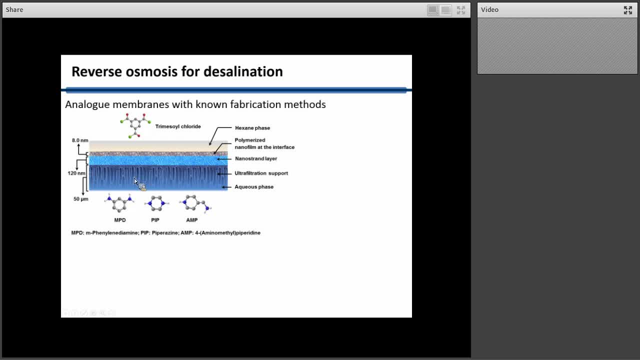 nanostrands on top of an open ultrafiltration support And we soak this layer here with an aqueous solution And then we contact that with a hexane solution of trimethyl chloride and we get a polymer nanofoam forming at that interface. 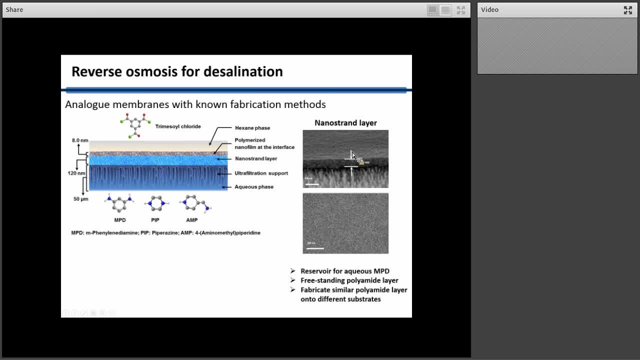 So if you look here, you can see that this nanostrand layer is very, very flat- That's 120 nanometres- and this forms a very flat layer on which we can form membranes, So it acts as a reservoir for aqueous MPD. 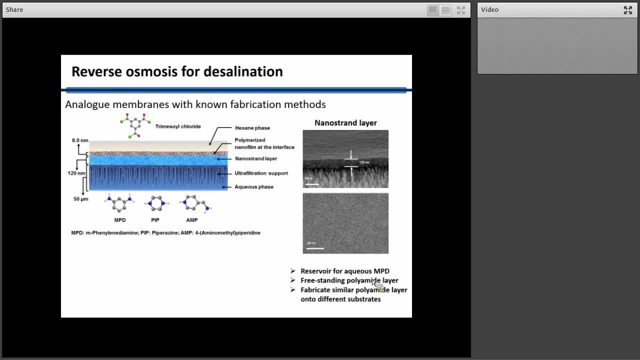 It allows us to fabricate freestanding polyamide layers, and then we can move those on to different substrates. Well, what we found when we did this is that if we used cadmium hydroxide, nanostrands with a low concentration of amine and trimethyl chloride, we can get extremely flat, very 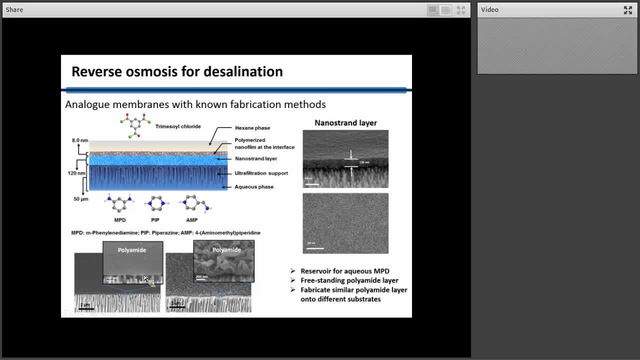 flat films made of polyamide. As we increase the concentration of the reactants, we get these rugose structures, the crumpled layers that you typically see in the commercial RO membranes, And we think that's because, as this interfacial reaction is happening, it's releasing heat. 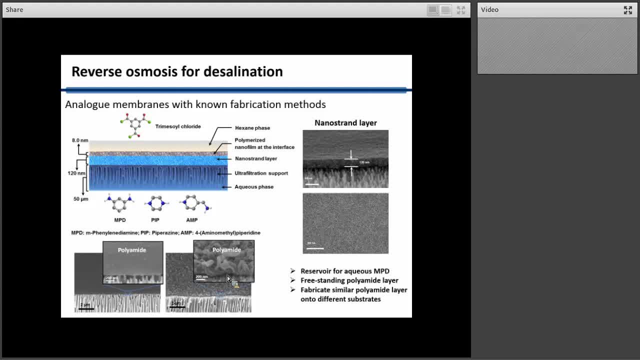 and that heat is creating instabilities and buoyancy effects at the interface and those are essentially frozen at the time of the reaction When you form this film- interfacial film- But we use this technique to make flat films and take them off supports and we can then 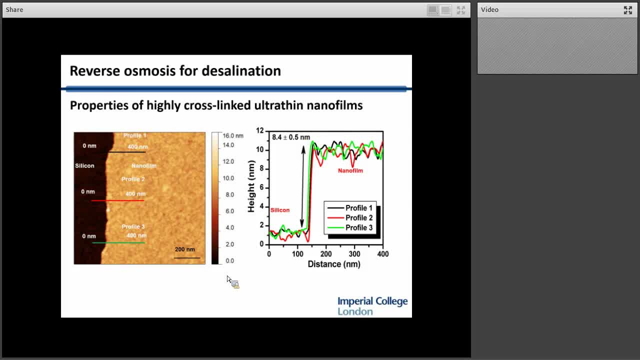 analyse those films. For example, now we could start to look at the thickness of the polyamide layer, And what you can see here is one of these very thin films laid onto a silicon wafer and we've dragged an AFM tip across the lip of that film. 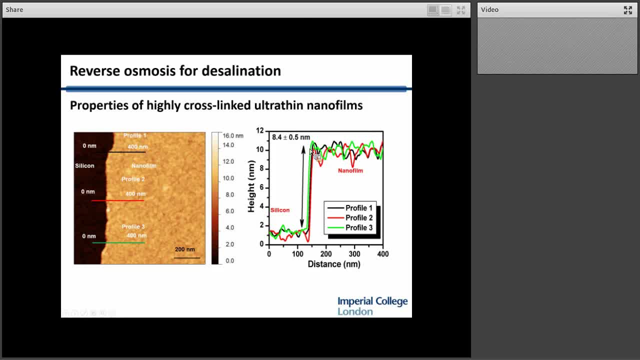 And what you can see is you drag the tip across, it jumps up by about eight nanometres And that tells us that the thickness of that nanofilm is about eight nanometres. Up to now, people have stated that the thickness of reverse osmosis membrane thin films are 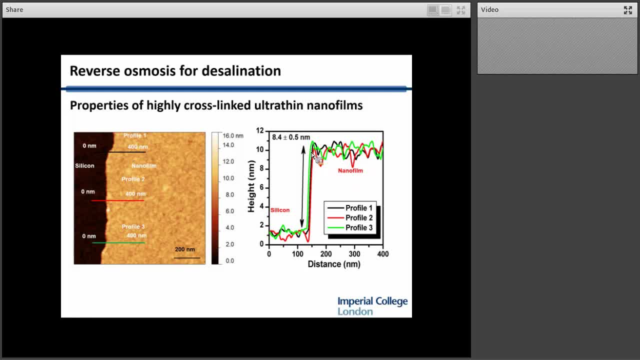 in the region 50 to 100 nanometres, And what they're really measuring is top to bottom thickness of that rugose, rough layer. But what we think the membranes comprise is these very thin films that then crumple up. So the real thickness of the separating layer is less than 10 nanometres. 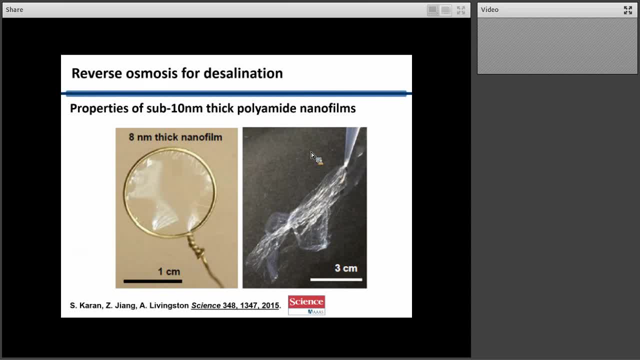 The surprising thing with these films is that actually they're very strong. So you can see here, we made a lasso which is about 1.5 centimetres in diameter, and then we attached one of these eight nanometre films to the lasso. 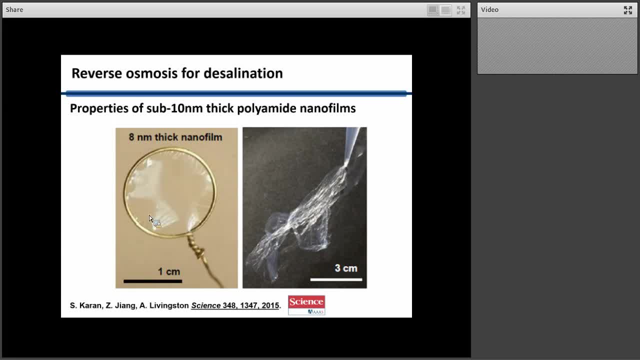 So if you just think about that for a minute, you've got an aspect ratio of something like a million here, one times 10 to the sixth, because you've got a film which is less than 10 nanometres, which is more than 1.5 centimetres in diameter. 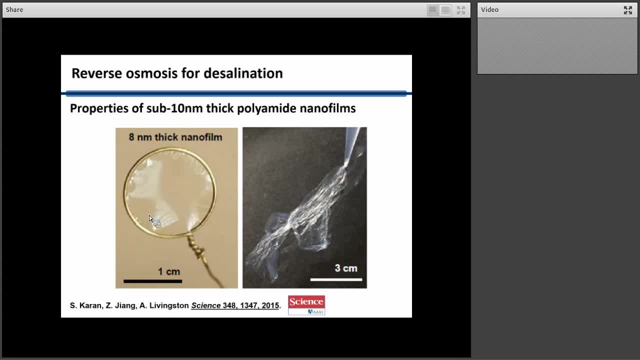 So it's about 20 molecules thick. And another surprising thing about that film is that it's very strong, so that if you laid the film on the lab bench and got a pipette and you sucked it up a pipette, which is what we're doing on the right-hand side here- 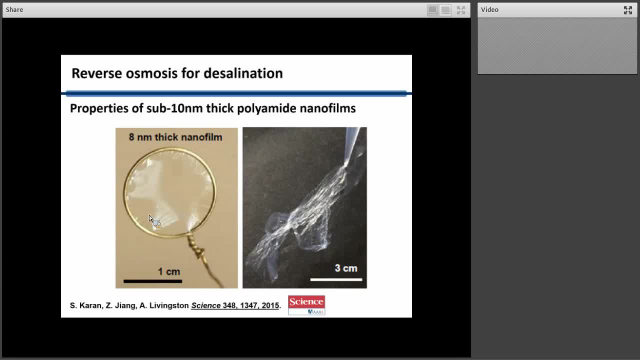 the film doesn't break. You can suck it up the pipette, get it out and spread it out again. So it's very thin, it's very flexible and it's very strong And that's what goes on the top of these reverse osmosis membranes. 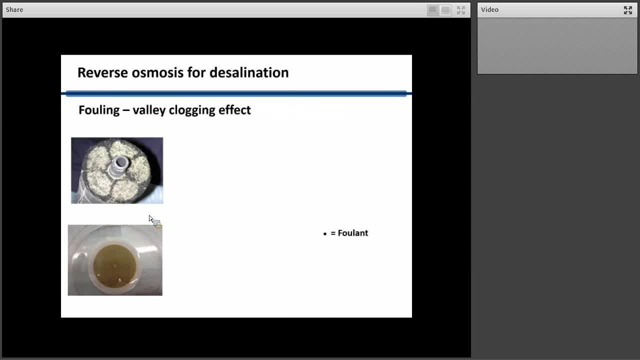 So we can use that for all sorts of interesting experiments, And what I want to do is just touch on one of the experiments we've done around fouling. So you can see here a fouled membrane module. This is all gunged up at the end of the spiral. 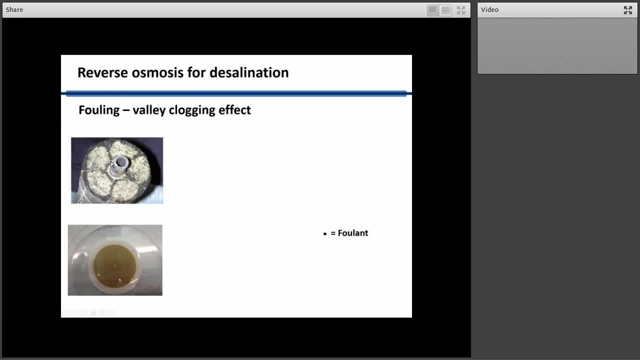 It's a spiral-wound membrane with grey sludge and scale and so on, And what we've done is tried to imitate this fouling with a defined model system. You can see one of our membranes here. we've been filtering BSA. 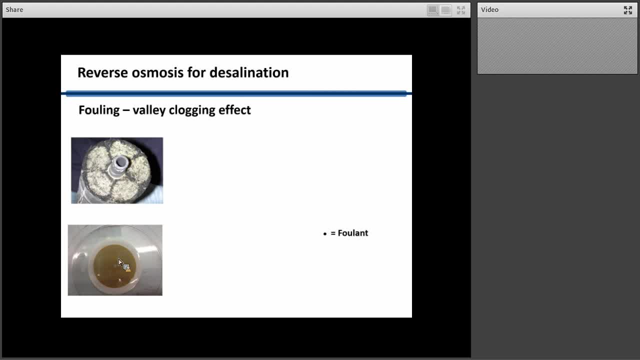 which is a protein typically used in the model fouling, And so the question we can ask is: what is the effect of the roughness of the membrane on fouling? So I can make a very smooth membrane, I can make a very rough membrane. 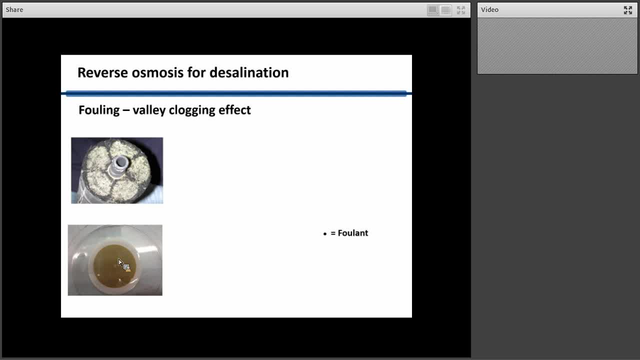 what is the effect on fouling? Now, when you think about that, you probably will think that the rougher the membrane, the more easily it's going to foul, And in fact, that is the received wisdom. That's what people have claimed. 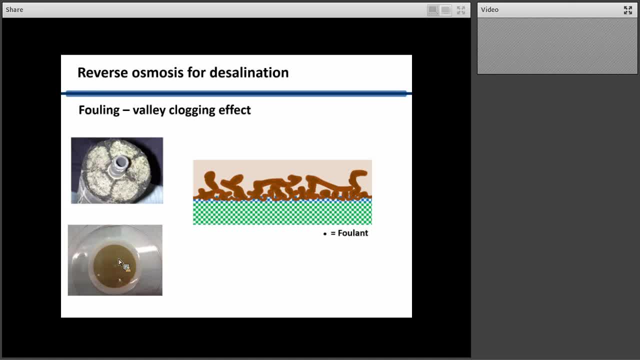 that's what people think: that a smooth surface will foul less. So we can imagine you've got a rough surface here and this is a cartoon of one of those rough, crumpled up films that I showed you. So it has the peak and valley structure. 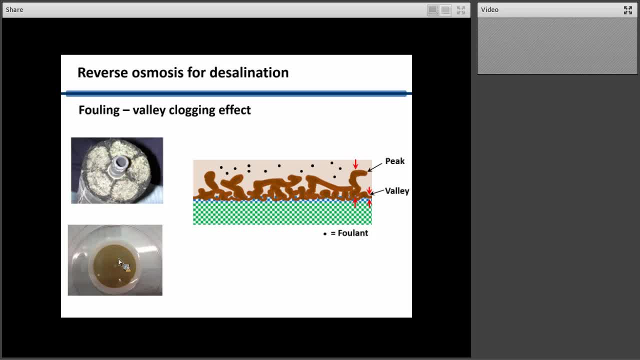 and then, as we apply, cross flow across the membrane, the permeate flow will be down to the surface of the membrane and that will tend to carry the foulants down into the membrane. If we have a flat membrane, then we'll have cross flow going across the membrane. 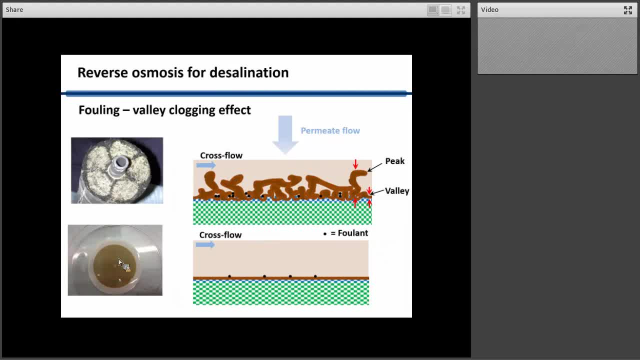 and the permeate will go down into the membrane. but you can see that if the foulants on the surface of the membrane, the smooth membrane, then we would expect that we'll have less fouling. And in fact, if I show you a couple of results from that, 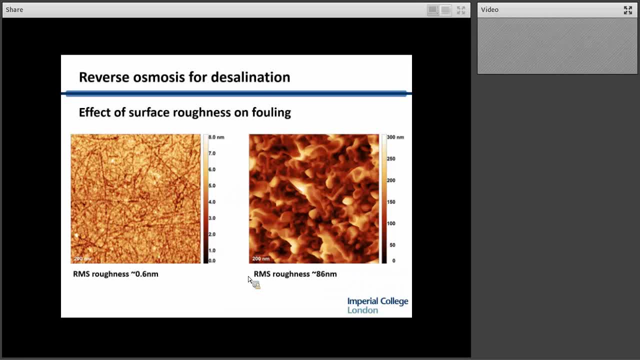 so on the left we have a smooth membrane that was made on these cadmium hydroxide nanostrands and on the right we have a membrane with a roughness of 86 nanometers. So if you look at that side on, the effective thickness looks like about 86 nanometers. 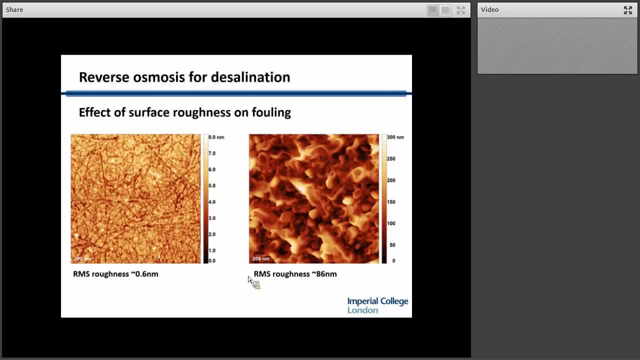 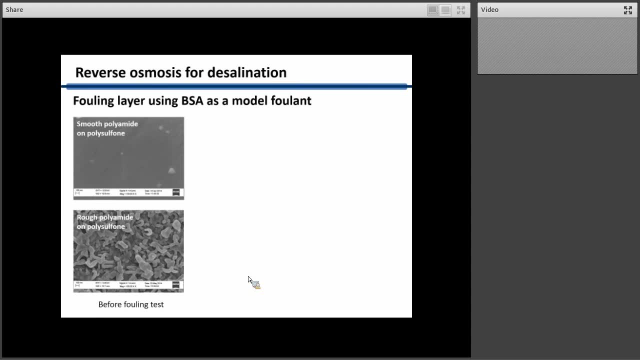 but actually it's a whole lot of films crumpled up that are probably only about 8 nanometers thick each, And if you take one of those smooth polyamide films on a polysulfone support and compare its performance in fouling to a rough polyamide film on polysulfone supports, 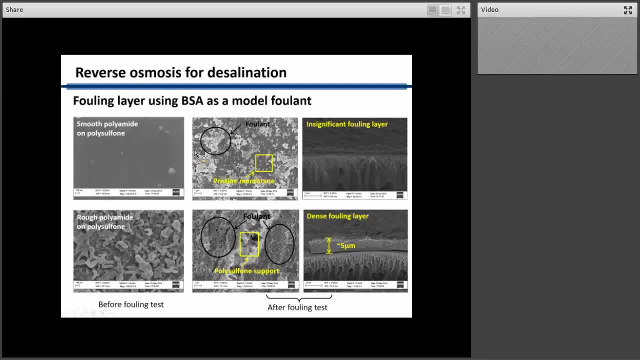 here's what you find. So you can see that in the smooth membrane you have some foulant. this is BSA building up here. but you have large areas of pristine membrane where we don't get much fouling at all And under the electron microscope you can see here. 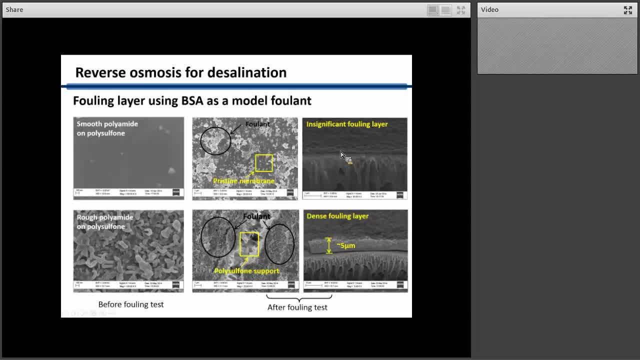 there's really an insignificant fouling layer If you compare that to the rough layer. so here we have a rough polyamide film on top of a polysulfone support. we have much less pristine membrane. we have a lot more foulant building up. 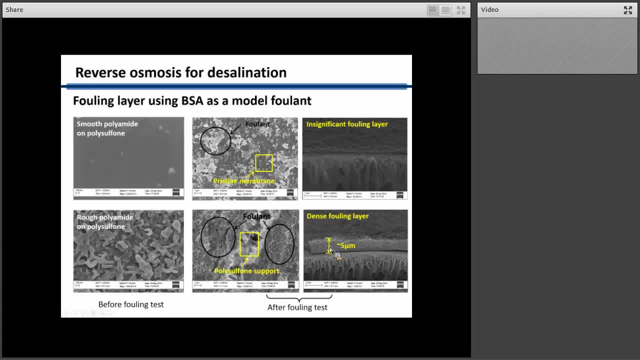 and we get something like a 5 micron fouling layer. So looking at that data, you think it's clear that the roughness of the membrane is leading to more fouling of the membrane. It's not quite as simple as that. When you look at the permeance, 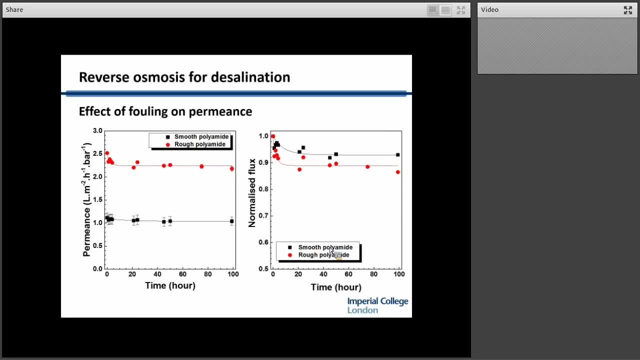 or the flux of the membrane. it turns out that the rough membrane has a permeance of double or more the smooth membrane- I'll come back to that shortly when I get on to organic solvent- So it has a higher permeance. So it turns out that the membrane, which appears to be 90 nanometers thick, 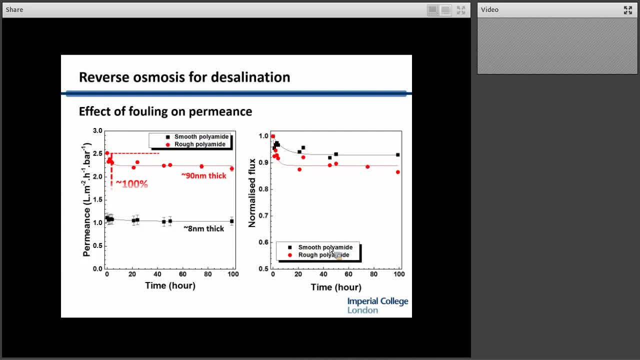 has a much higher permeance than one which is 8 nanometers thick, and the reduction in flux that you get is higher for the membrane, which is rougher. So you get 12% flux reduction. this is normalised flux. on the right 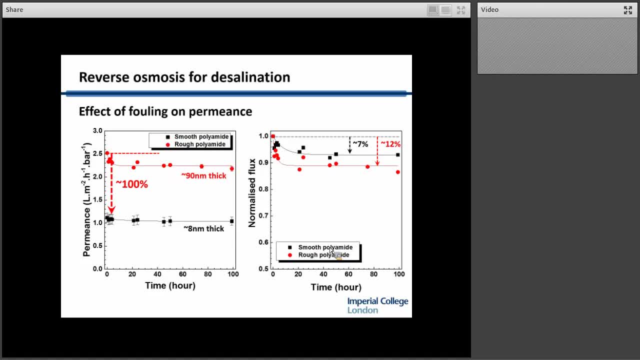 versus 7% flux reduction on the smooth film. The thing is that's not a well controlled experiment because you've got two things that are different: the roughness of the membrane and the permeance of the membrane, And the higher the permeance. 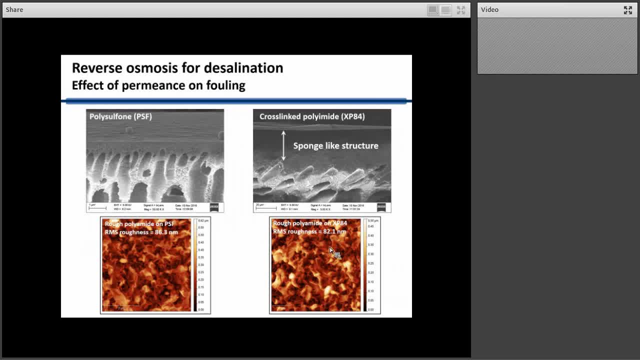 the more rapidly the foulant is brought down to the surface of the membrane. But with this platform technology we've developed of making these very thin or rough or smooth films and putting them on supports. we can actually put this film on different supports And the support can affect the permeance of the membrane. 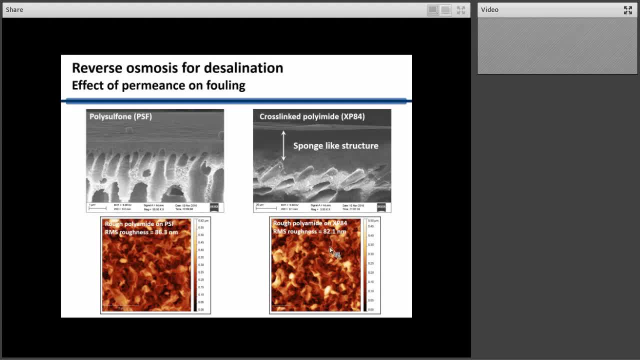 So what you see here is two different supports- polysulfone on the left and the cross-linked polyamide on the right- And this support gives you much lower permeance. So what we did now is we made rough membranes on both of them. 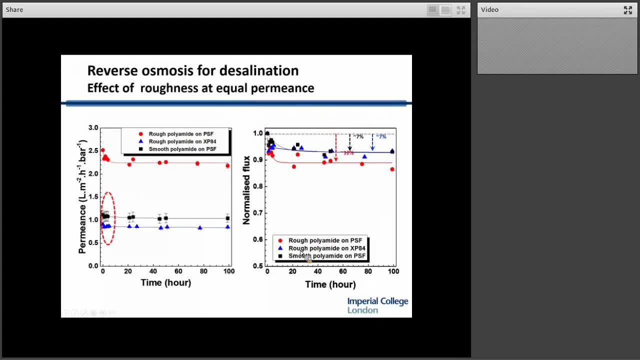 So both of these are rough membranes. But the rough membrane made on the polyamide support- the cross XP84, these blue points- is of the same order of permeance as the smooth polyamide. So now we can compare the membranes which have the same permeance. 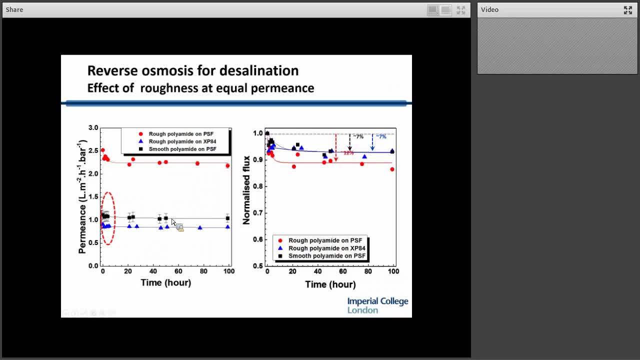 the black and the blue points, which are rough and smooth, And what you can see when you look at the data here is they lose about the same amount of permeance. So the rough membrane and the smooth membrane both go down about 7% in fouling. 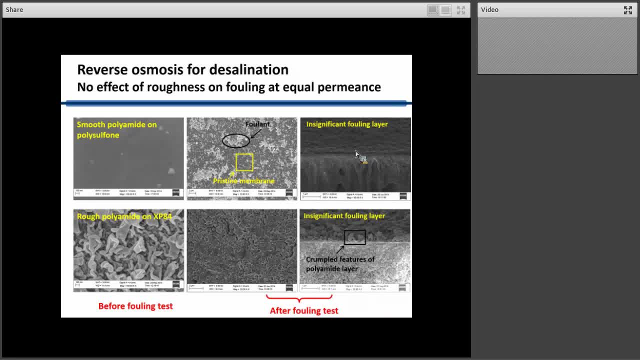 when you expose them to the BSA And in fact, with the rough polyamide which has the same permeance, you can see there's quite a lot of pristine membrane and there's an insignificant fouling layout on both the smooth membrane and the rough membrane. 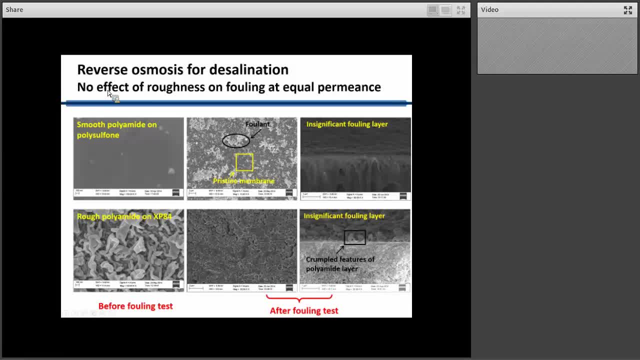 So that tells us that actually, if you control the experiment by using these thin films and playing around with the supports, there's actually no effect of roughness on fouling at equal permeance. So, counter to what we've believed up till now, 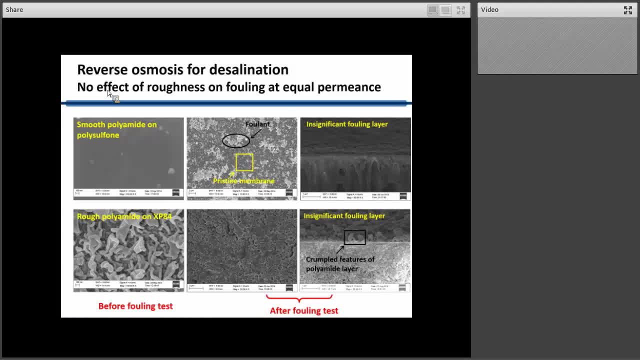 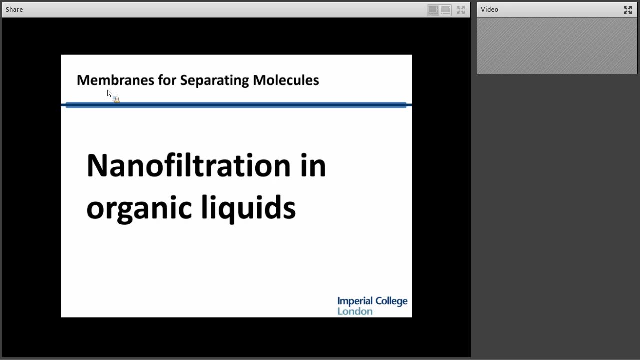 the roughness of the membrane doesn't impact on the fouling. More important is the permeance that the membrane has and the rate at which the foulant is brought to the surface of the membrane. So the second application of membranes I wanted to talk about in molecular separations. 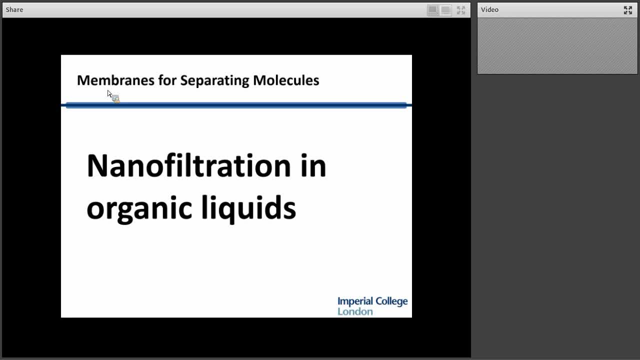 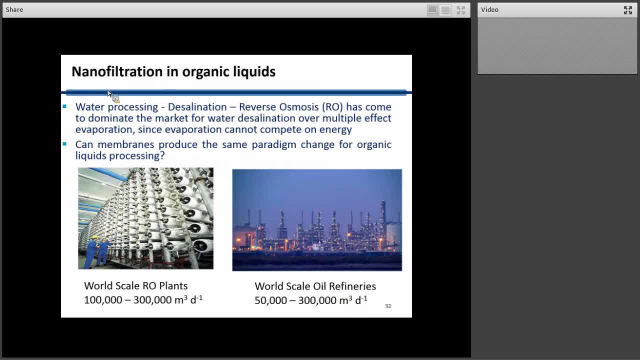 is nanofiltration in organic liquids, And this is something which, as I mentioned at the start of the talk, my own research group has worked on for the last decade or so, And it's an interesting one because, if you think about water processing, 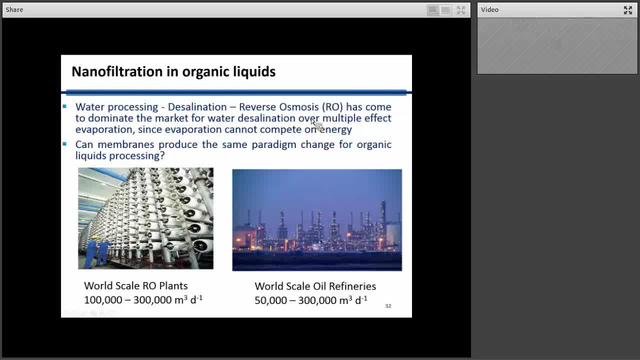 and desalination. reverse osmosis has come to dominate the market for water-delt desalination over multiple effect evaporation, And the reason for that we've already been through, with me sitting on my bicycles: It's just because evaporation cannot compete. 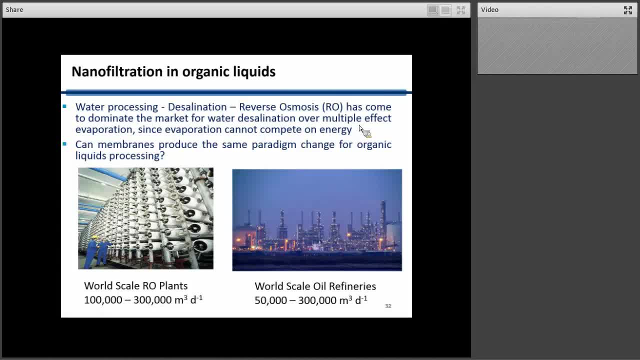 on energy with desalination by membranes. So this is a picture of a modern desalination plant. They handle 100,000, 300,000 metres cubed per day, so large flows. But if you look at the same equivalent. 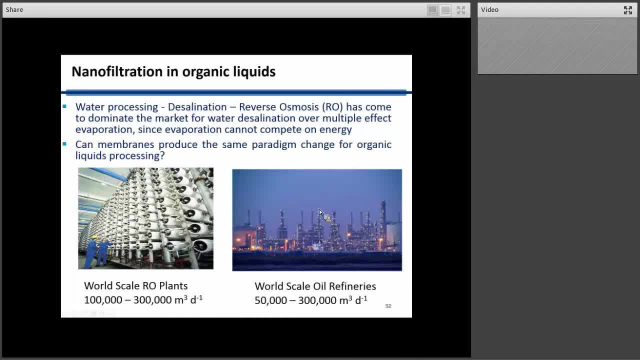 volume processing plant for organic liquids, for example, an oil refinery- all you can see is distillation columns. So membranes haven't made anything like the inroads into distillation and to organic liquids processing that they have into water processing. So the question is: 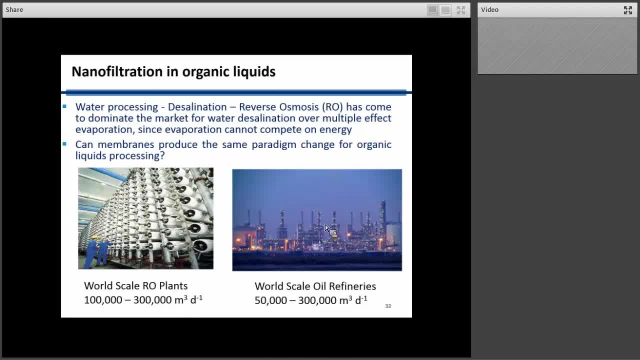 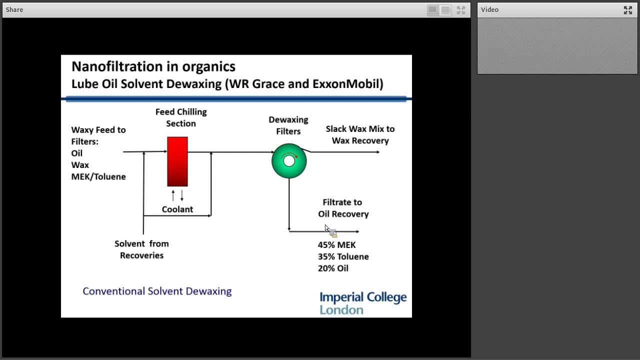 can membranes produce the same paradigm change for organic liquids processing as they have for water? And the answer is maybe in some cases. And I'll start off by giving the example of the largest liquid organic liquids filtration plant ever built so far, And this is used for. 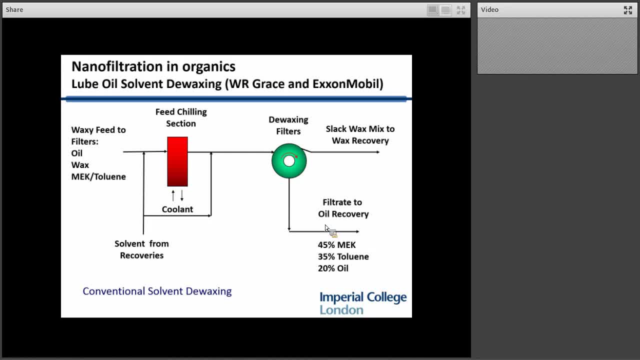 de-waxing of lube oils And this was invented by WR Grace and they made the membranes and installed by Mobil and became ExxonMobil. Now the idea here is you have a waxy feed, which is a mixture of oil. 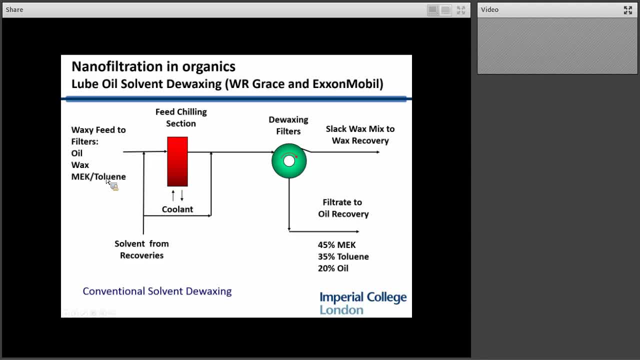 these are high molecular weight molecules and MEK and toluene is solvent And you chill that down and the wax precipitates out as a white waxy material which you take out in these de-waxing filters and the slack wax goes off to recovery. 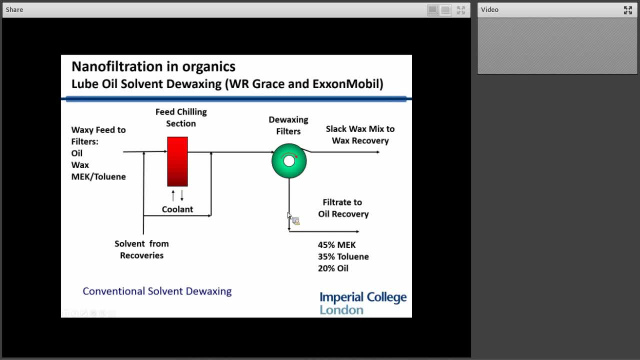 and then coming through at something like minus 10 degrees C, you'll have your filtrate off to oil recovery, which is high molecular weight oils and solvents, And what you have to do with these is to heat them all the way back up to the boiling point of the solvents. 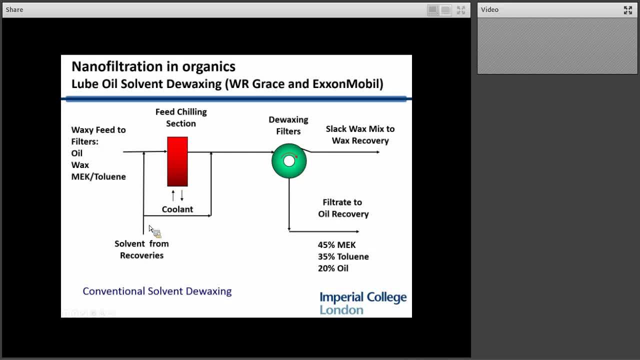 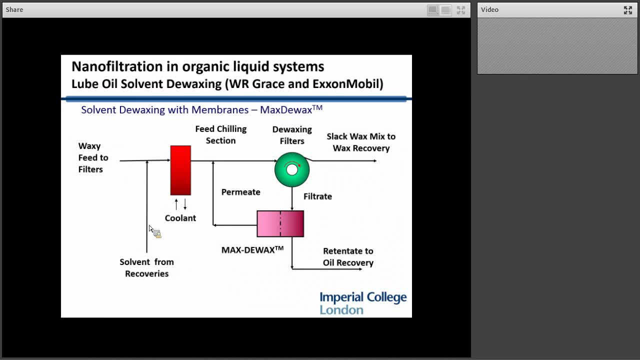 to recover the solvents and put them back in here. Energetically that's not sensible, because you have to refrigerate the solvent, then you've got to heat it up to evaporate it. So what they did was come up with a process. 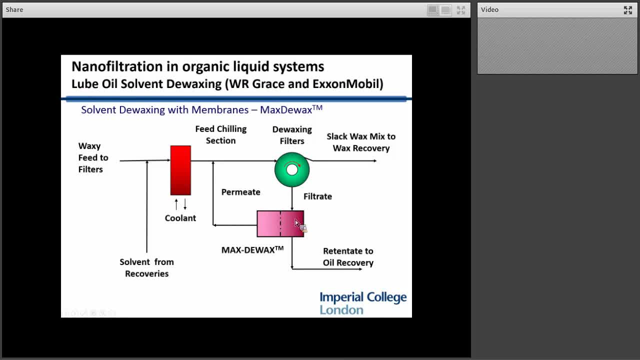 where they could do the separation of a large quantity of the solvent at low temperature. So when it comes through the filter at minus 10 degrees C, apply a membrane. If that membrane is stable in MEK and toluene, you can recycle the solvent. 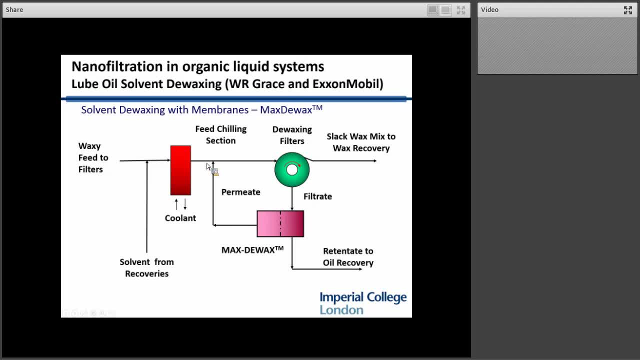 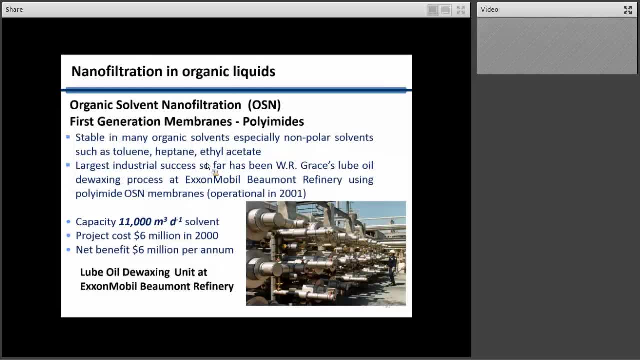 back around into the system and add it in after the refrigerator, drastically reducing the load on your refrigeration plant. So they came up with what I call the first generation of organic solvent nanofiltration membranes. These are stable in solvents like toluene. 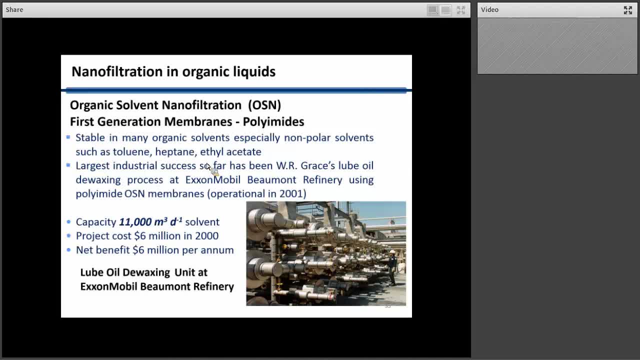 heptane ethyl acetate and they're membranes made from polyamide And WI. Grace and ExxonMobil worked together to build a plant at their Beaumont Texas refinery. This is a shot of the plant here So you can see. 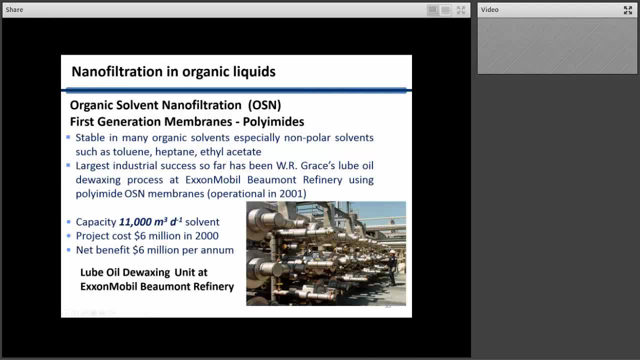 it's a whole lot of insulated pipes. Those pipes are housings I alluded to earlier. So in each of those pipes you've probably got four or five spiral well membrane modules put together in a string And they're operating with a solvent mixture. 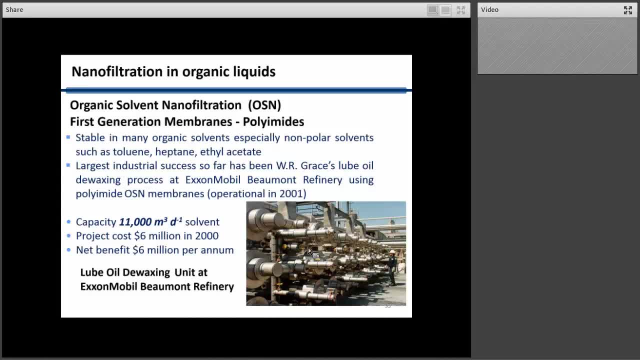 And that can handle up to 11,000 metres cubed per day of solvent. It cost $6 million to build in 2000 and the net benefit was $6 million per annum, So it had a one year payback. Just to give you an indication. 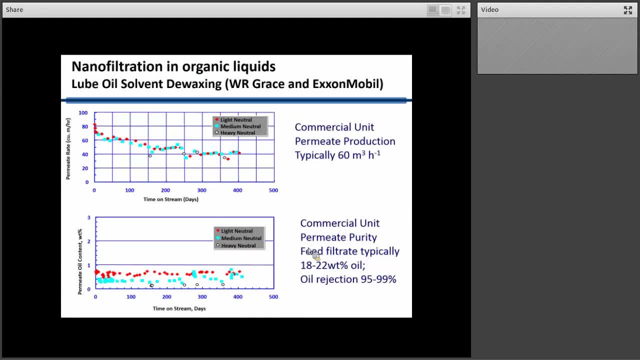 of the performance of that plant. this is data for a period of over a year on the commercial production of lube oil And what you've got on the top plot is the permeate rate in cubic metres per hour. You can see that goes down. 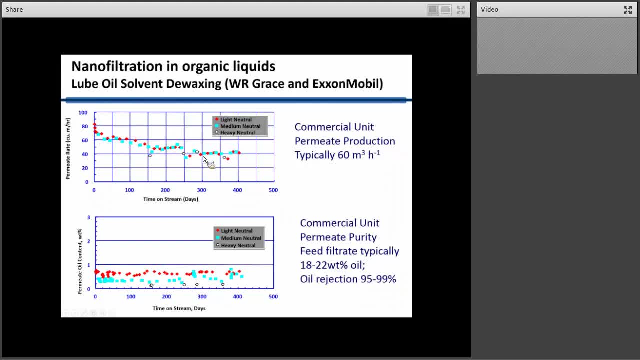 That's one of the problems with membranes is the flux goes down over time. That can be due to fouling on the surface or ageing of the membrane, And what you can see here is the oil content. So going in the oil content's typically. 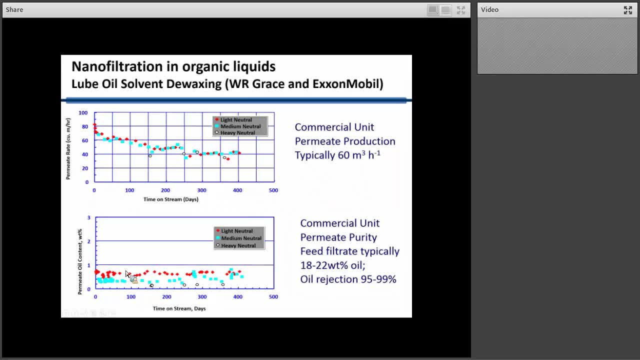 18 to 22 weight per cent And, coming out, the oil content is always less than one weight per cent. So the oil that you're recycling back around, the solvent you're recycling back around, is essentially clean and you're rejecting 95 to 99 per cent of the oil. 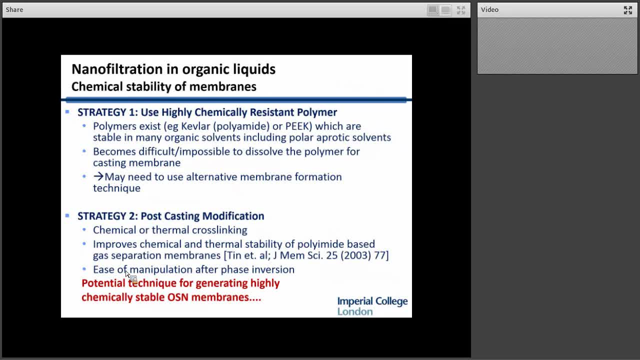 But the trouble with those membranes, in terms of using them more widely outside of refinery applications, is they're not very chemically resistant. So in fact that polymer P84, that was used to make those membranes is the polymer I showed you in the video. 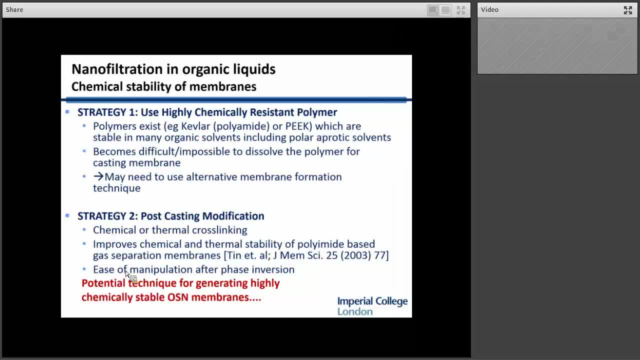 of how we make membranes. So it's clear that that polymer will dissolve in solvents like DMF, and that's how you cast it. So how are we going to make membranes that are more generally stable across all sorts of solvents in different chemical regimes? 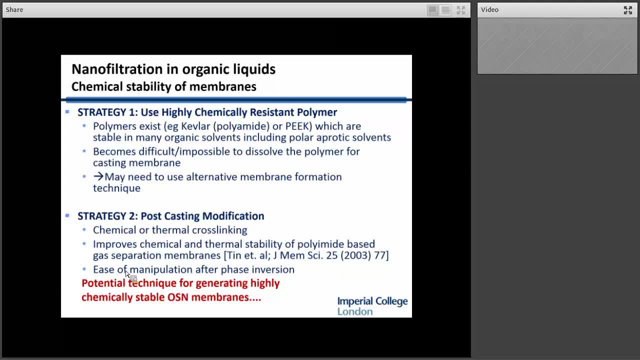 Well, you might think about using a very chemically resistant polymer, For example Kevlar, which is a type of polyaramide or PEEK. These are stable and inorganic solvents. The trouble with using those polymers is you can't dissolve them. 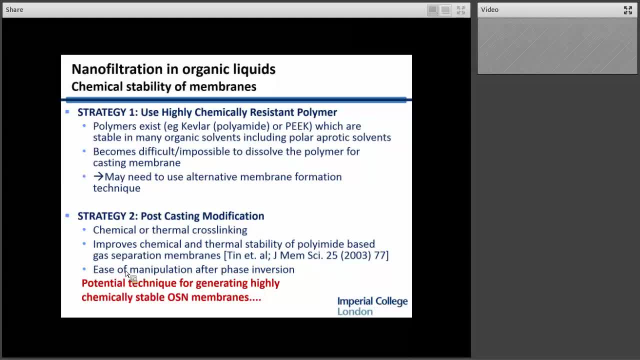 And it's a problem if you can't dissolve them. So the problem with using those polymers is you can't dissolve them. And the problem with using those polymers is you can't dissolve them. And if you can't dissolve them, it's extremely difficult. 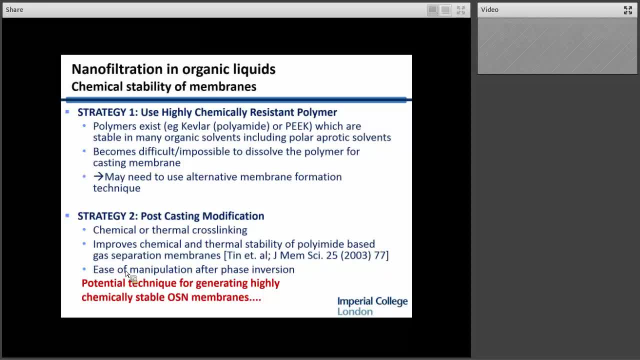 to cast them as membranes. So you have to think of another way of making them into a membrane. A second strategy for making membranes will be to take something like the polymer I showed you the polyamide, cast it and then, after you've cast it, 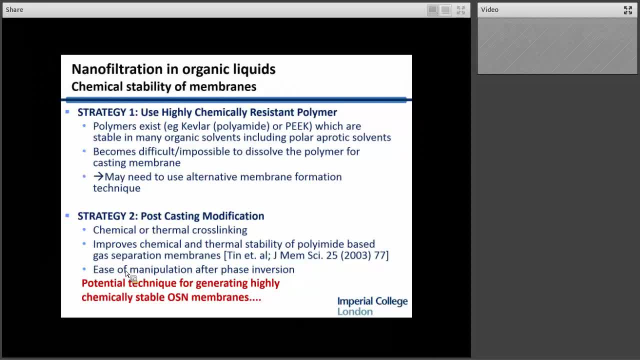 cross-link it, so that the polymer becomes, instead of being a series of chains, becomes chains that are linked together by other smaller molecules, cross-linking molecules, And that should make them insoluble. So that's a strategy that we use to make membranes. 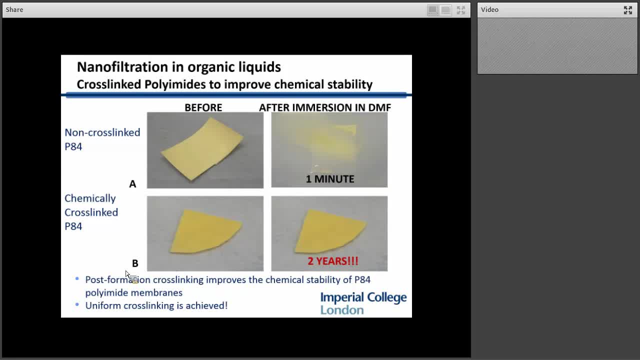 Now what we found is that if you take a membrane and you cast it, this is from P84 polyamide. if you put it back into DMF as a solvent, in less than a minute the membrane is totally re-dissolved here. 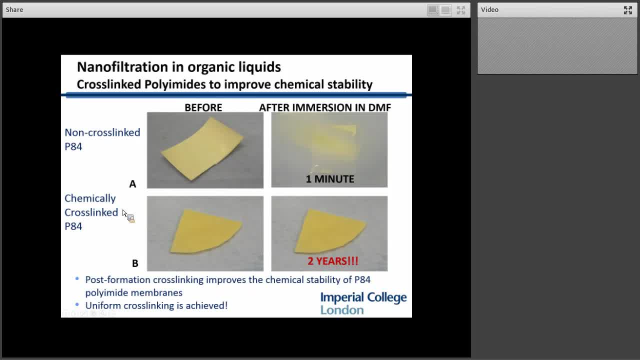 But if we chemically cross-link that- and we did this using diamines to break open the polyamide ring- then after two years the membrane's still stable. So by casting a membrane and then cross-linking it you can make it stable. 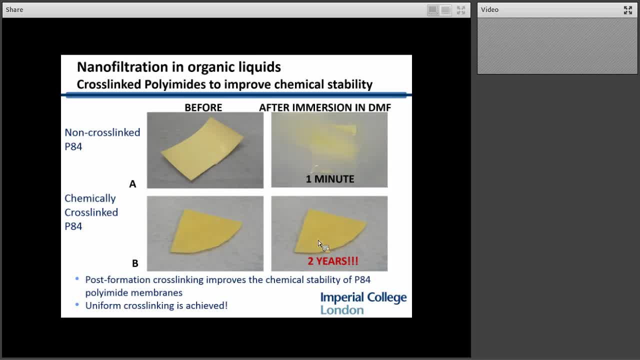 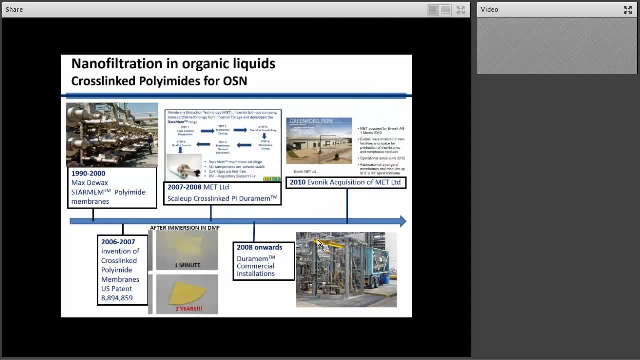 to even the solvent in which you originally dissolved the polymer, So that developed its own story. The original membranes made from polyamide were made by Grace for this Max-D wax plant, And in my research group we came up with the idea of cross-linking. 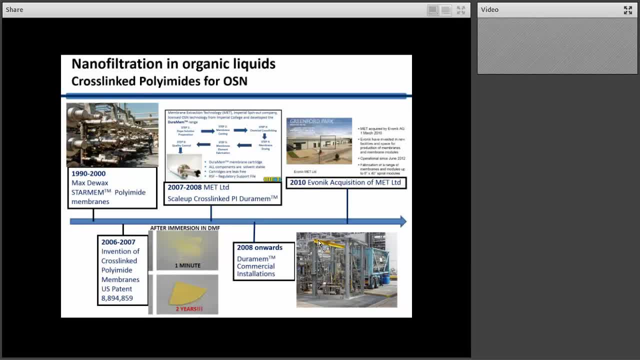 these polyamide membranes. Actually, as it turns out, we patented that idea, We granted patents for it in various jurisdictions, And then we decided that we would start to manufacture those membranes. So we had a company that came out of Imperial College. 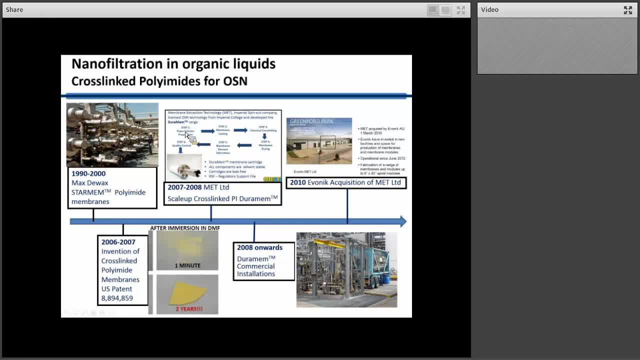 in membrane extraction technology And we developed a process for making these membranes: dissolving the polymer and casting the membrane, cross-linking them chemically- all of this at larger scale- drying the membrane, making these spiral-well membrane elements and then, finally, 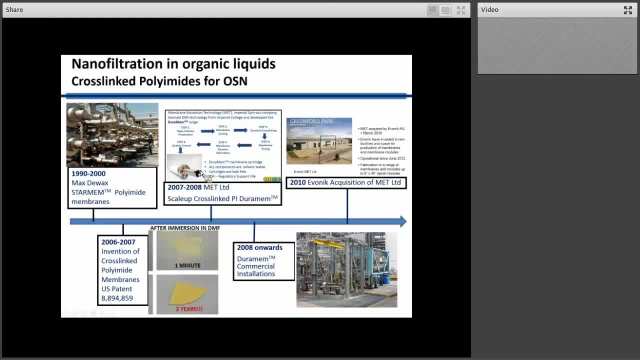 using quality control on them. Many of our customers actually were in the pharmaceutical industry, And so we had to have a cartridge, a spiral-well cartridge. Of course, all of the components had to be solvent-stable and the cartridge had to be leak-free. 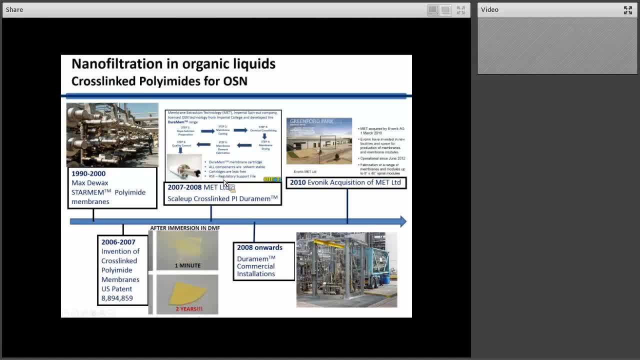 Importantly, we also had to meet regulatory requirements for pharmaceutical applications And we managed to do all of that with our first commercial installations of this membrane, which we trademarked the Duramen membrane. We were in pharmaceutical factories. You can see one here. 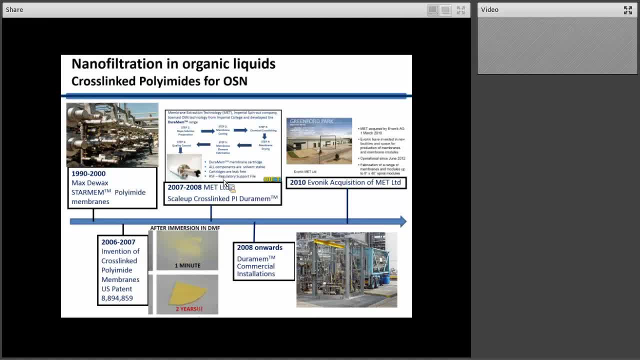 at a GlaxoSmithKline factory in Cumbria And around 2010, that business, MET, was acquired by Evonik, which is a large German chemical company, And Evonik built a larger facility in West London. 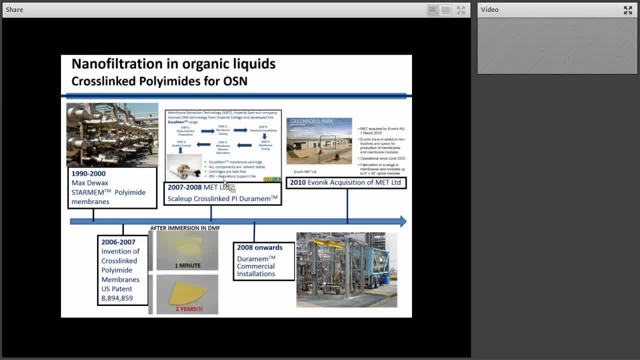 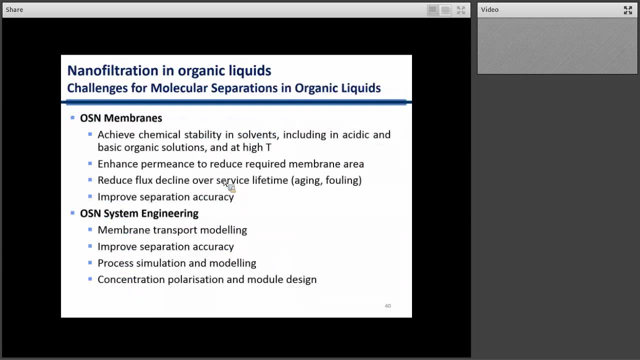 where they currently manufacture spiral-well membrane modules up to eight inches in diameter. So four and a half inches in diameter of the membrane. So that's the large-scale spiral-well membrane modules for organic solvent nanofiltration. So 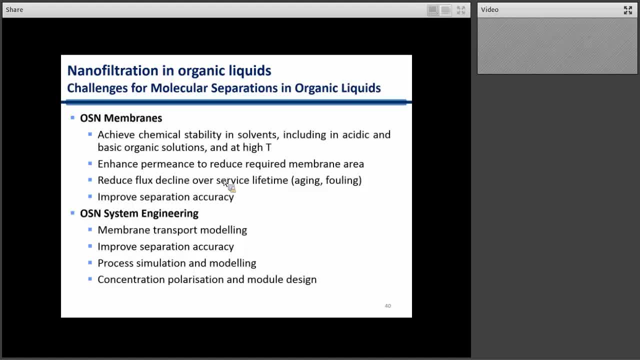 that's the story of the cross-linked polyamide, which has a number of applications, But the question is: what are the challenges for molecular separations in organic liquids now? And I think some of the interesting points are: how do I get better chemical? 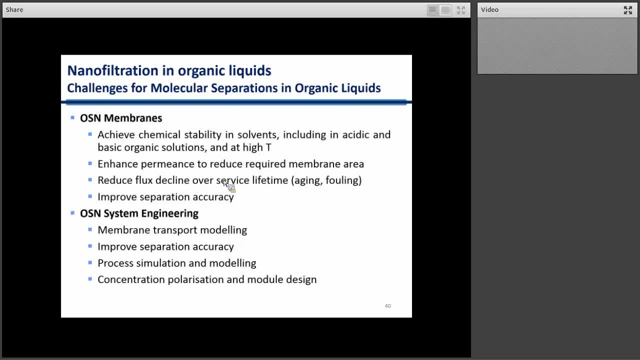 stability? How do I improve the permeance? How do I get more accurate separations? How do I do process simulation and modelling? How do I get over concentration, polarisation and module design. And I think it's fair to say that some of these 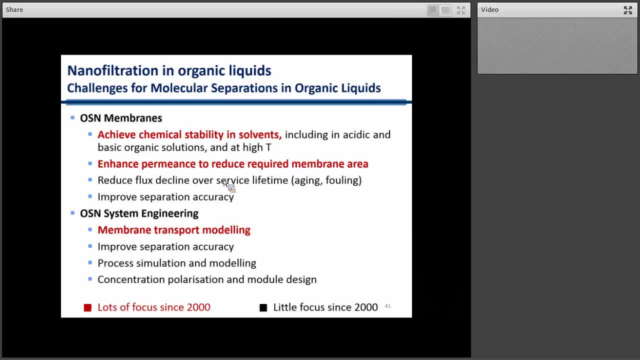 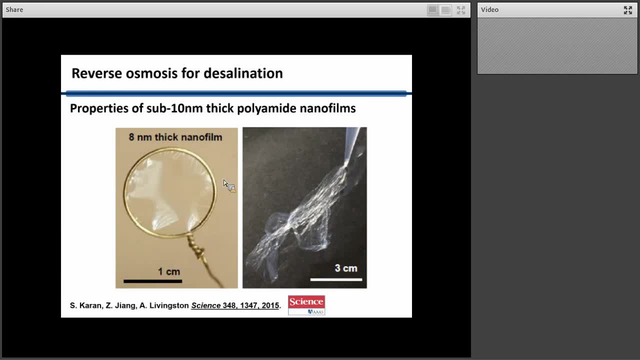 questions have received a lot of attention: Chemical stability, the permeance, the transport modelling- and some of them have received a lot less attention. I'll come back and make some comments on that at the end of my talk, But I want to return. 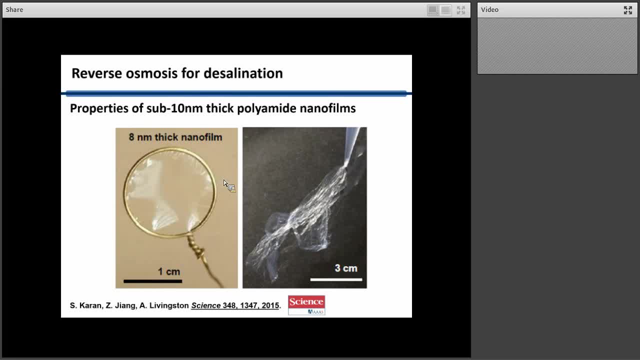 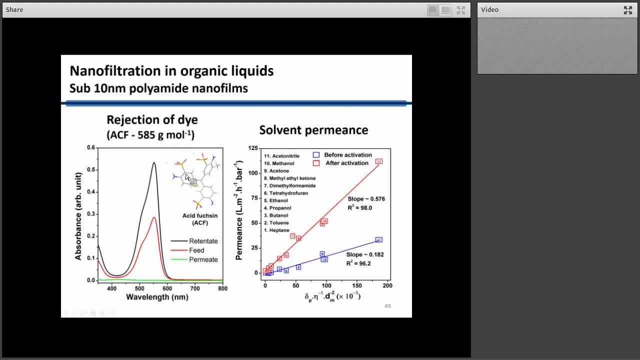 to these 10 nanometre polyamide films that we made. So we made these, and these are also quite interesting for working with organic solvents, And what you can see here is the rejection of the dye. This is the structure of the dye. 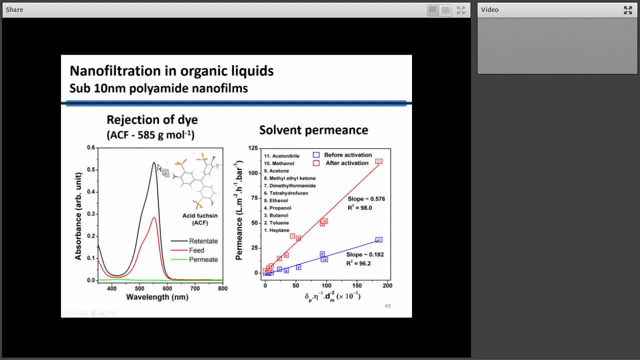 This is the dye in the feed. If we filter this feed through the membrane, the concentration goes up in the retentate because the dye can't pass through and there's almost no dye in the permeate. So these very thin polyamide films. 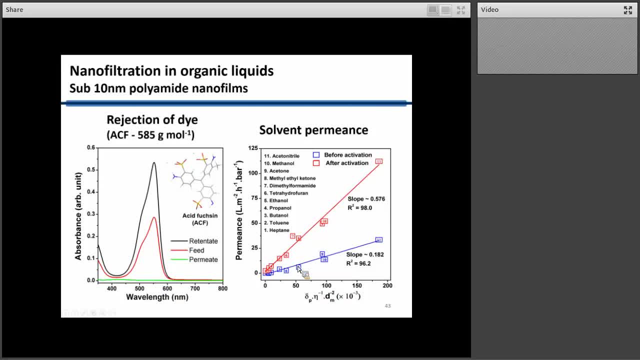 have very good rejection of solute molecules. We also found that if we treat them with DMF as a solvent, it can go up by a factor of three or four from this blue line where we tested the permeates of a number of different solvents. 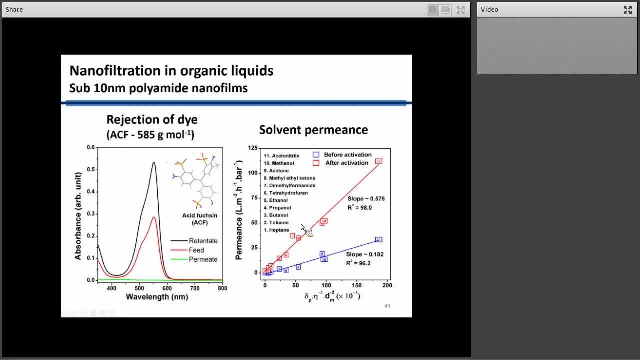 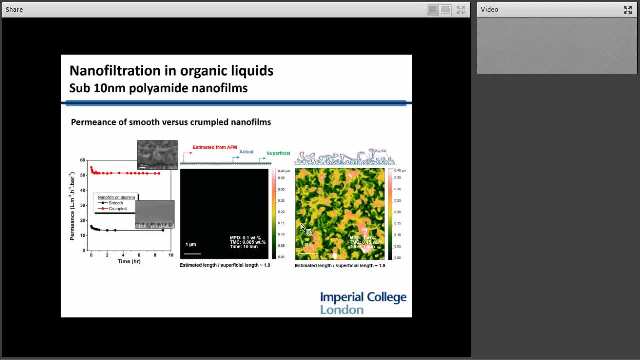 to the red line, which is what we call activated with DMF. So these very thin polyamide films are interesting membranes for organic solvent filtration And I promised you earlier in the talk that I'd come back to why the crumpled membranes have. 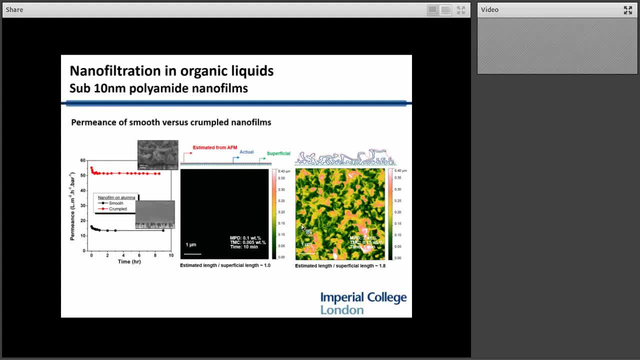 a higher flux than the smooth ones or higher permeates. So what this data shows you is the permeates of acetonitrile, a solvent through a crumpled membrane. So you can see the crumpled membrane here and the smooth. 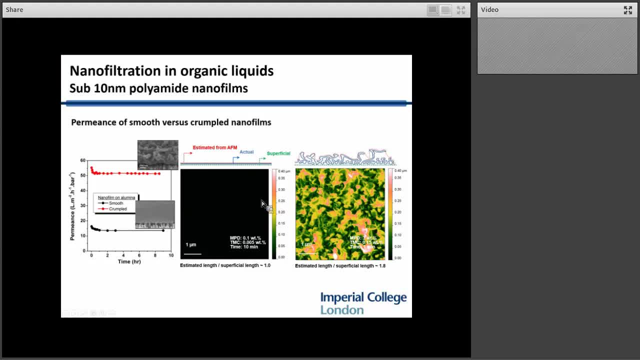 membrane here. If you look at the surface of this crumpled membrane, it's really rough. The surface of the smooth membrane is, of course, smooth And the reason we think that the flux is much higher through these crumpled membranes. 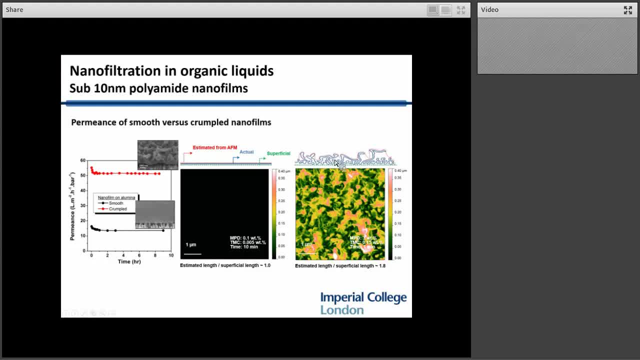 is a lot of these things that stick up here are actually hollow, So you've got a whole lot of extra area per area of membrane in the form of all these hollow protuberances and things sticking up into the fluid, which is what we 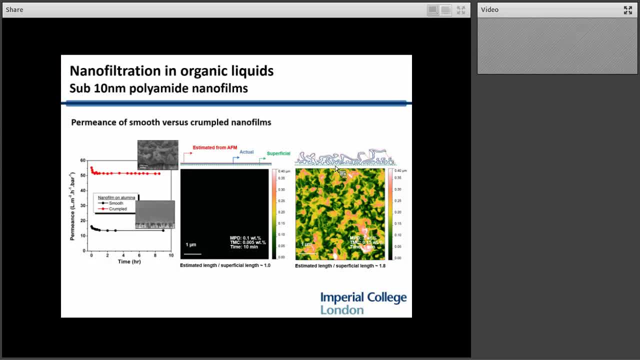 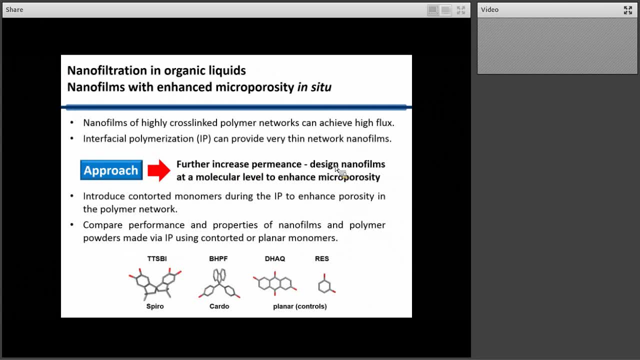 call the crumpled membrane. So the reason the crumpled membranes have a higher permeates is just because they have a higher filtration area per area of support. We didn't stop there. We got very interested in this idea of very thin 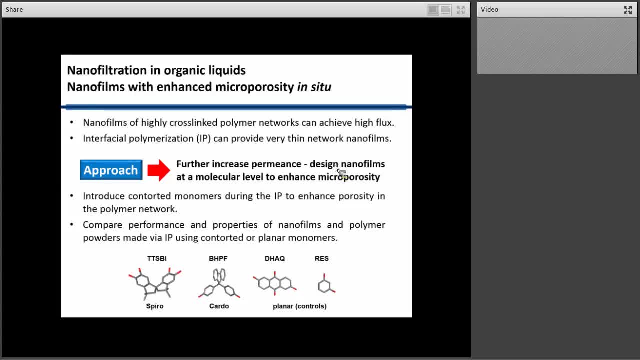 nanofilm membranes and we wondered whether we could, by changing the monitors we used for this interfacial polymerisation reaction, change the pore structure inside the thin films. So we realised that these nanofilms of highly cross-linked polymer networks can achieve high 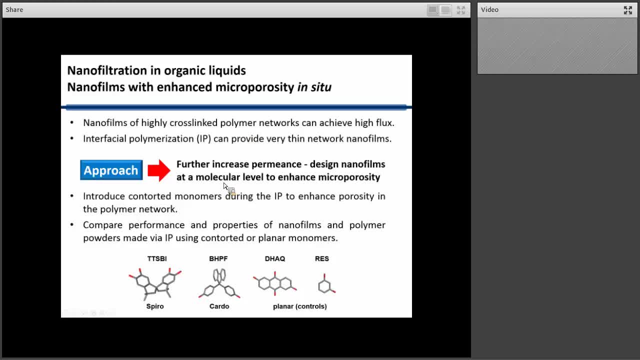 permeates. So we started asking ourselves: could we design the monomers that we use for this interfacial polymerisation reaction to influence the pore structure in the membrane? So to test that, we tried two what we call contorted monomers. 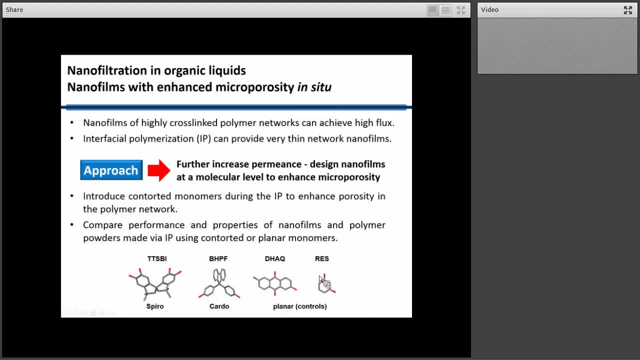 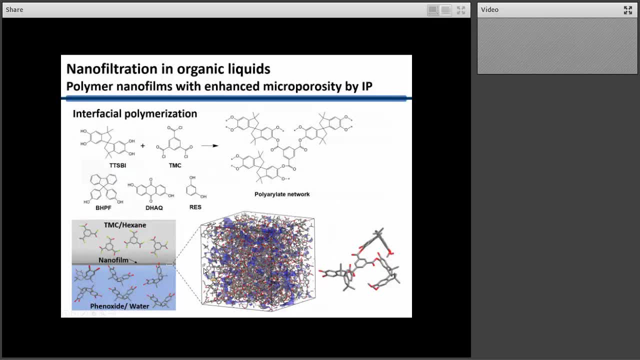 These are monomers like this, where they have angles that can't bend very easily, and we tried two flat monomers. So we wanted to understand whether membranes made from these flat monomers and membranes made from the contorted polymers would offer different properties. 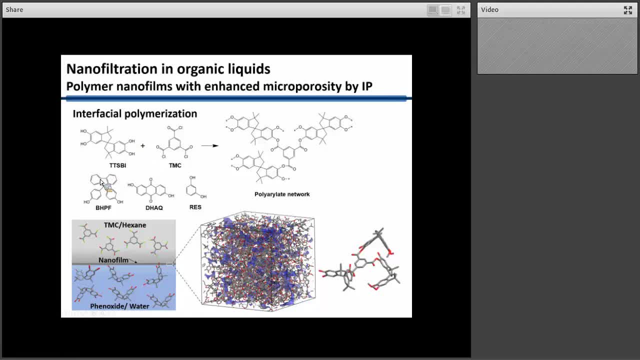 The way we did that was to carry out a polyester reaction and various contorted and non-contorted phenols in a sodium hydroxide solution. So these react together to give us a polyester or polyarylate network and you can get the idea of what that. 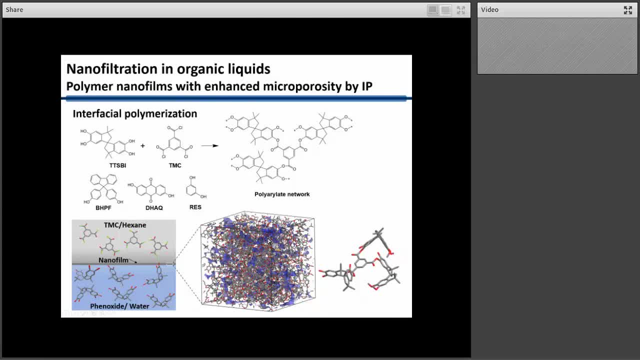 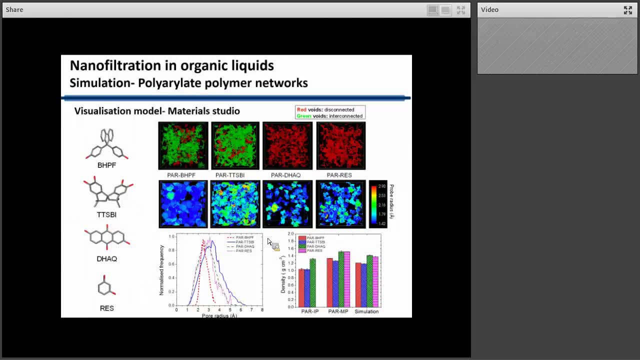 network might look like here. Now we're lucky in our chemistry department to have Kim Jelps, who's an expert in molecular modelling of polymeric materials, and so Kim did some modelling for us, and what she predicted from these models that she did is that 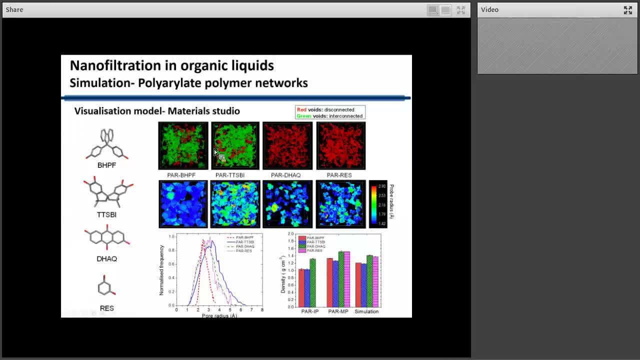 using these two contorted monomers here- these are these two boxes- we would have far better interconnected pore structures than if we use these flat monomers here. So these are models made from the flat monomers and the red signifies the pore structure, and 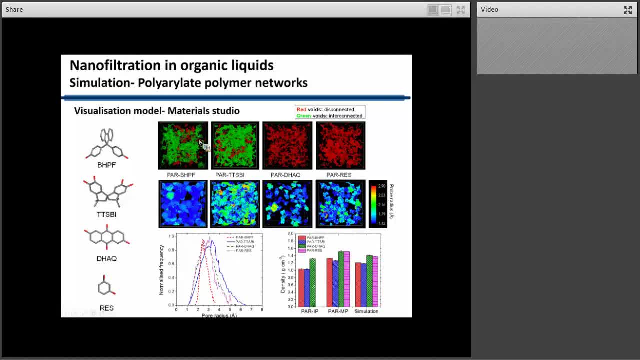 the green signifies the interconnected pores, and you can see here that the interconnected pores are much bigger when we have these contorted monomers, Even though, if you look at this plot, the pore size isn't that different. the key to using these contorted 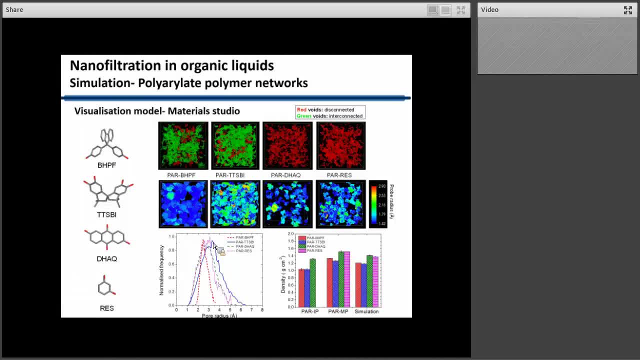 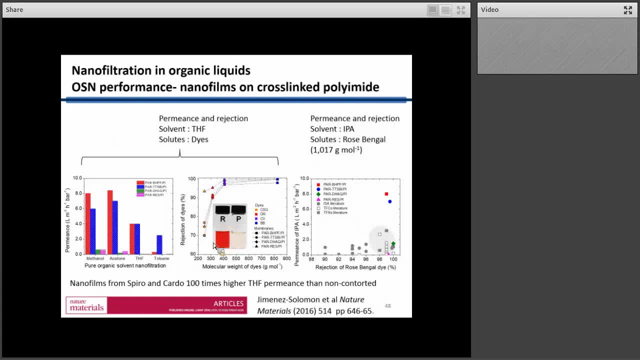 monomers is that the pores are far more interconnected, and when we looked at the permeate to those polymers and the permeate to those membranes, we found that that was exactly what we observed experimentally. So what you can see here on this, 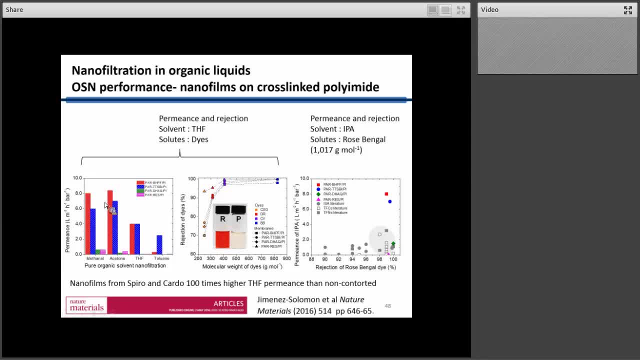 left-hand plot is the red plots for the membranes made from the contorted monomers, so the red and blue offering very high permeances, and the membranes made from the flat monomers, the green and the pink offering very low permeance. And if you look, 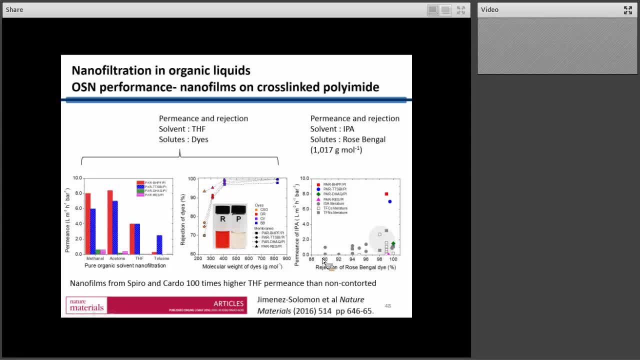 at the rejection of these membranes versus their permeance. you can see, these are the typical membranes available in the literature and these are the two membranes we made with the contorted monomers. So by adding contorted monomers into our mix we can get some. 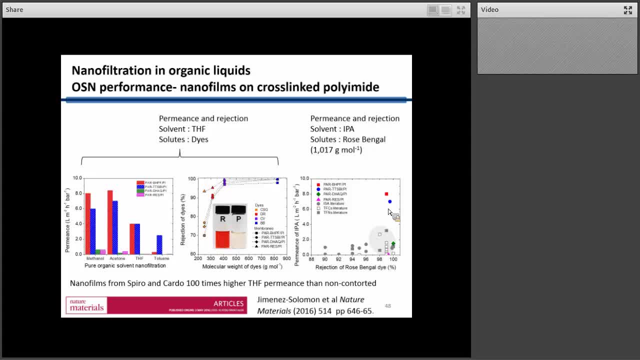 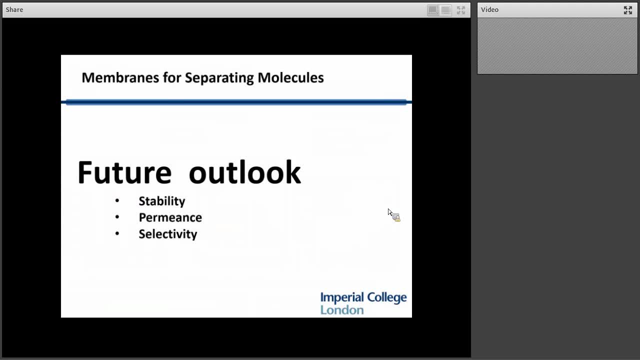 control over the pore structure of that very thin film in the top layer of the membrane, And that came out just earlier this year in Nature Materials. So now I want to finish with a few slides on future outlook. So I think there's three key. 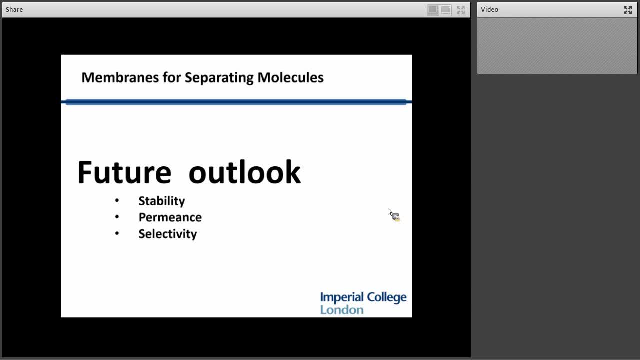 things that are important in membranes. One is their stability, and by that I mean with respect to chemicals and solvents and their environment, and also their stability over time or ageing. There's their permeance: how much liquid you can get through them per unit. 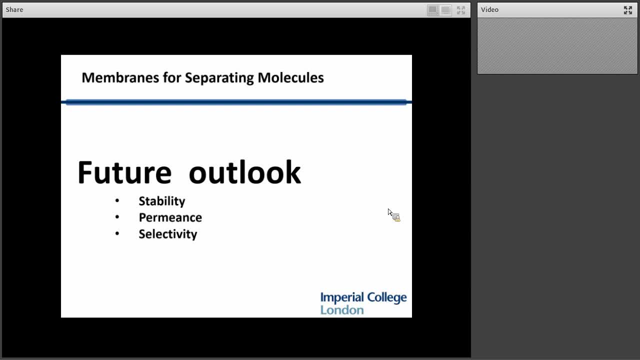 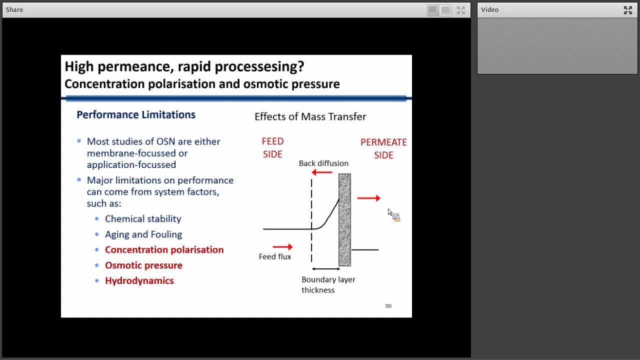 of time per applied pressure and there's selectivity. So how good they are at discriminating between different molecules. I think it's fair to say that most of the work so far has really gone into the permeance, trying to make membranes with. 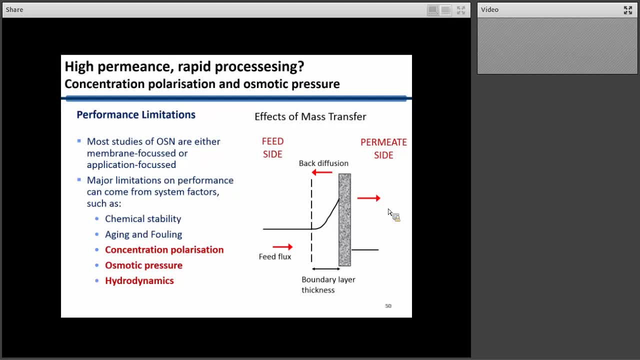 higher permeance and then their chemical stability. But if you look at the performance limitations on the membranes, most studies are either membrane focused or application focused. The major limitations on performance can actually come from your system factors, for example chemical stability, ageing and 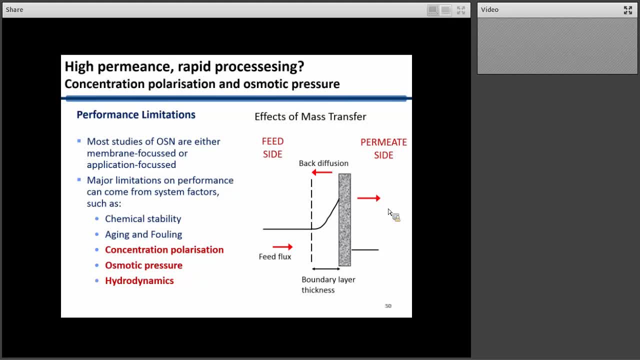 fouling, but also concentration, polarisation, osmotic pressure and hydrodynamics. So if this is the membrane- here, as I have a flux towards the surface of the membrane- the non-permeating species or the solute will. 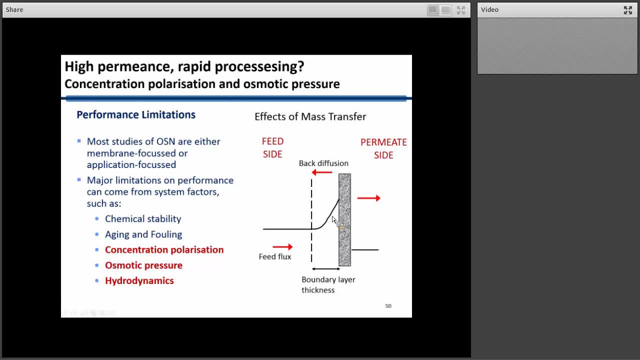 build up and form what we call a concentration polarisation layer here, And this is the membrane permeance, And this eventually leads to a higher concentration of solute at the surface of the membrane than in the bulk liquid, increases the osmotic pressure. 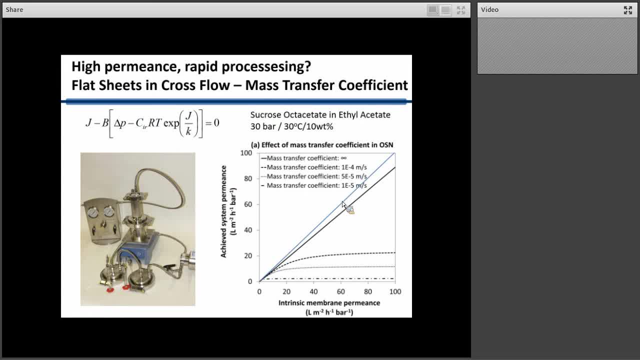 and reduces the driving force available for the process, And that's reflected in these curves here. So you can work out what effect that will have by just solving a simple equation here where you take account of the mass transfer, And what you can see is: this is a parity. 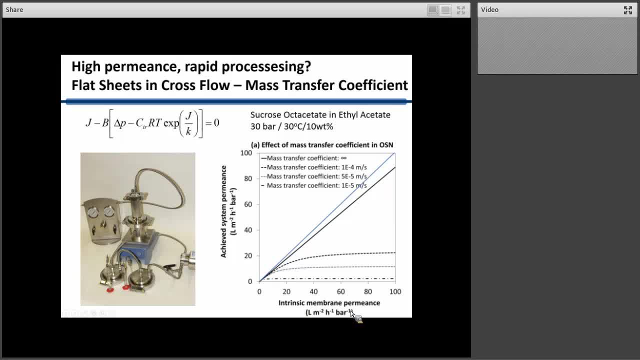 line between the intrinsic membrane permeance. I have a membrane and I measure its permeance in perfect conditions versus the achieved system permeance and what I get is a solution of ethyl acetate as a solvent and a 10 weight per cent solution. 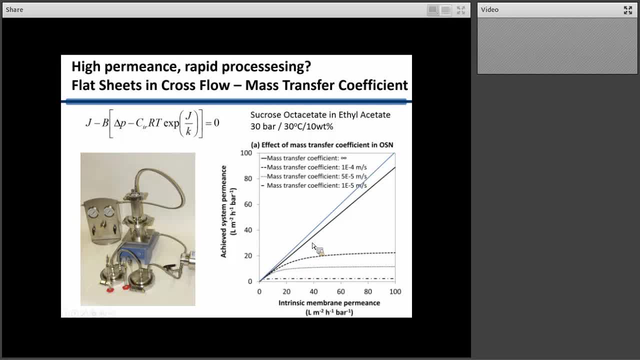 of sucrose octoacetate as a solute. So if I had an infinite mass transfer coefficient in the system so I pump fluid over the surface of this membrane quickly enough and I had enough turbulence at a very high mass transfer coefficient, I get a. 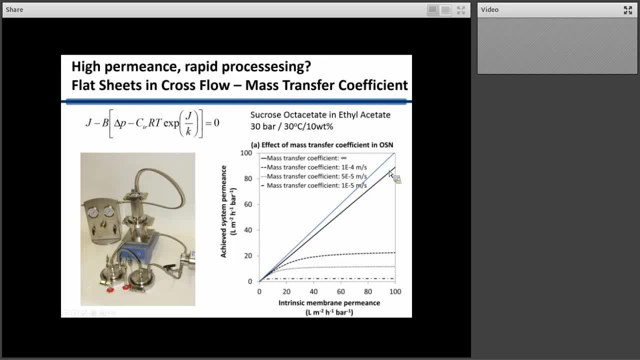 slight difference between the achieved and intrinsic permeance is because of the osmotic pressure. But as my mass transfer coefficient goes to 1 times 10, to the minus 4, which, by the way, will be a very good mass transfer coefficient, down to 1 times 10, to 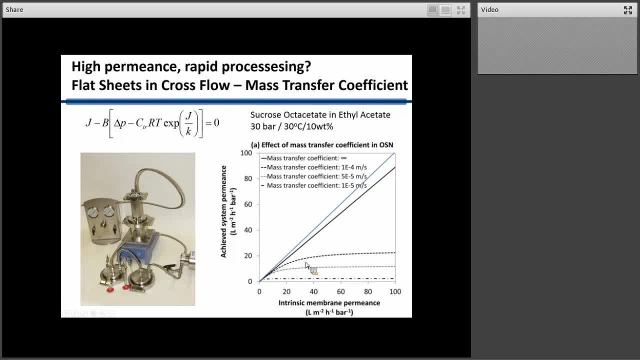 the minus 5, you can see that the achieved system permeance- what I get out of my membrane- starts to level out and does not increase as the intrinsic membrane permeance increases, which is to say that I can improve the permeance of my. 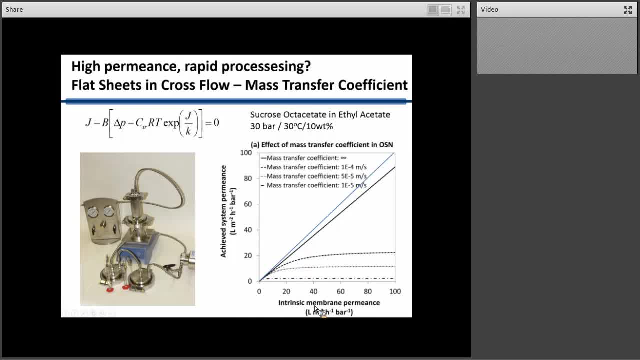 membrane. but it won't necessarily improve the permeance I get out of the system because I'm totally limited by mass transfer in the boundary layer above the membrane. Another limiting factor is pressure efficiency. So if I have a system permeance that I can get out of, 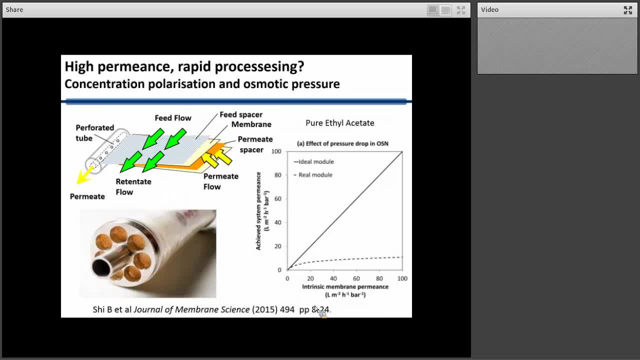 the system. I can get out of the system because I'm totally limited by mass transfer. So I can get out of the system, but I'm totally limited by mass transfer. So what happens is that the pressure efficiency drops. We've already gone over. 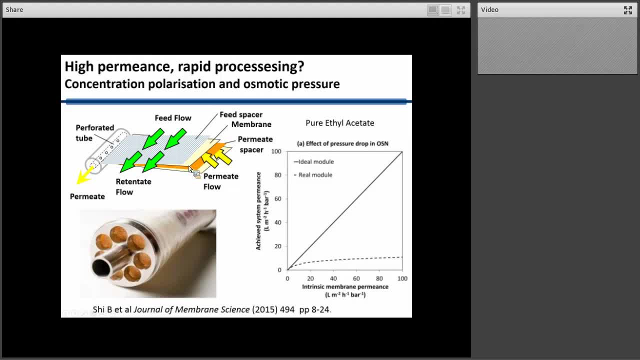 spiral well modules and what happens is you have some pressure drop down the feed flow side and you have some pressure drop on the permeate spacer here, so that the pressure you have here will have to be greater than the pressure you have here to get flow to. 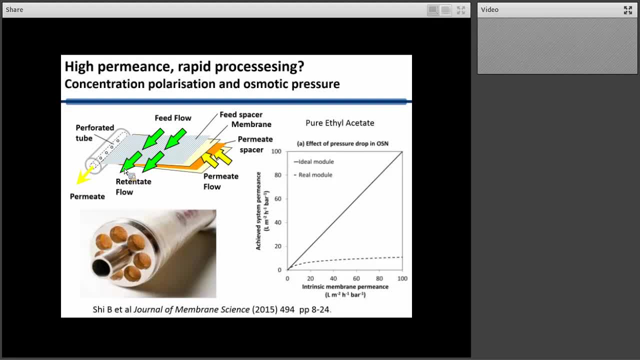 go down the spacer, which means you apply a pressure, but the pressure inside your permeate spacer will build up, and so the actual difference in applied pressure won't be as high as your feed pressure. So what happens is you get a higher and 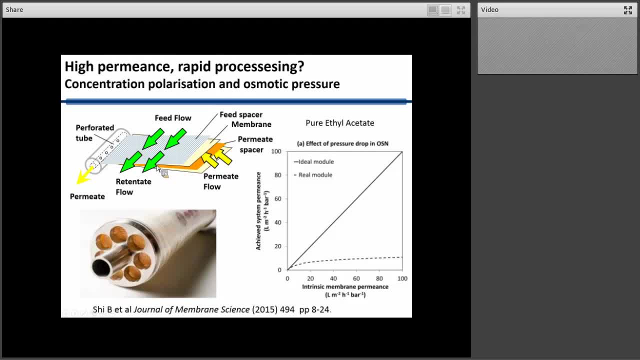 higher pressure drop inside the permeate spacer because as more and more material comes through the membrane you get a higher and higher pressure drop inside this permeate spacer. So purely on pressure alone for a pure solvent. you can see, here's my 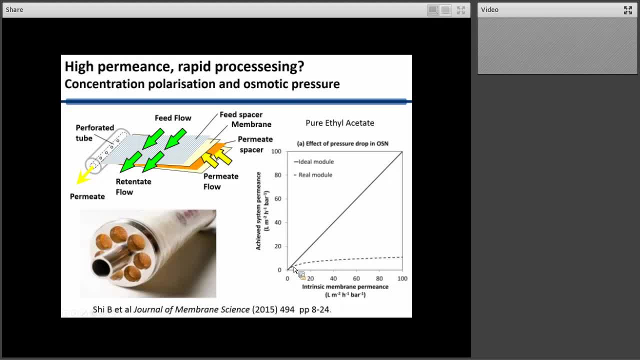 parity line and this is what I would actually get out of a typical membrane. So initially I get some increase with the system permeance because of my membrane permeance but at some point increases in the intrinsic membrane permeance simply won't. 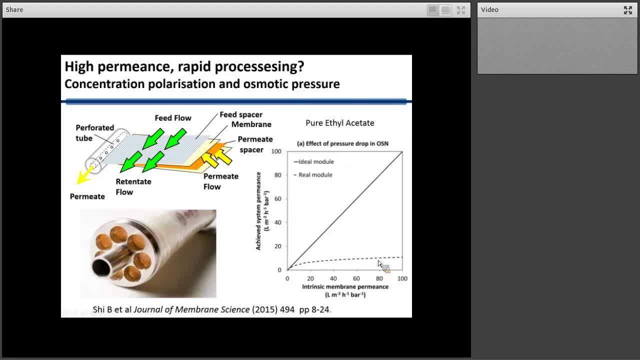 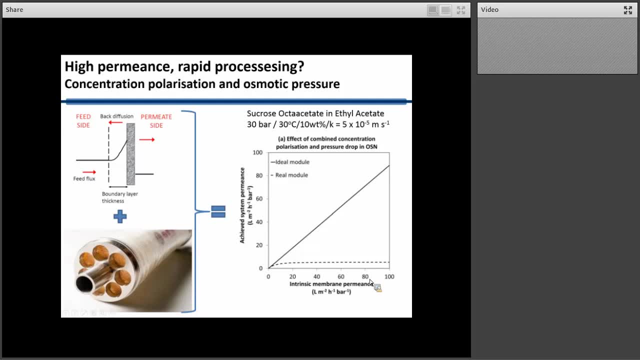 increase my achieved system permeance anymore. And if you put together concentrations of the permeate spacer you get a concentration, polarization and pressure drops in spiral membranes. You get this rather dismal curve here which shows you that if I increase my intrinsic membrane permeance it's 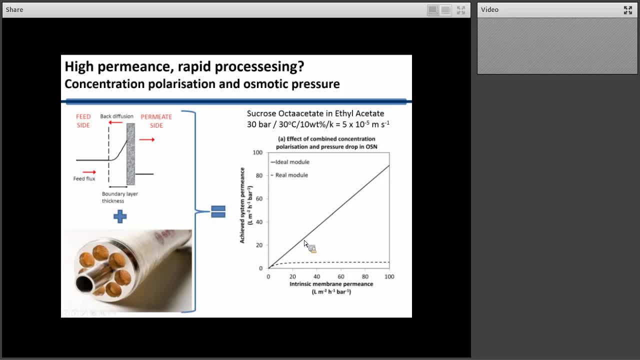 actually not going to do much for my achieved system permeance, which is to say that other factors in the membrane permeance are limiting the system Concentration, polarization, pressure drops in the module, And so in concluding remarks I would say that 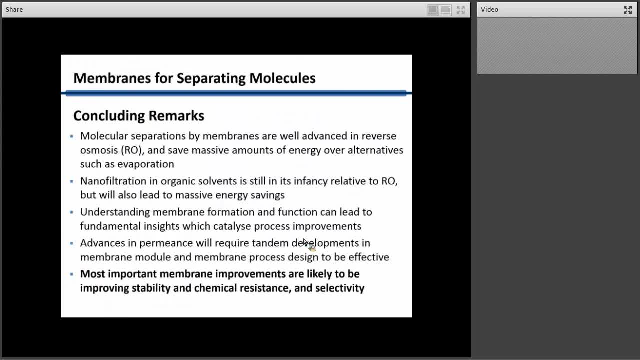 molecular separations by membranes are well advanced in reverse osmosis and they save massive amounts of energy. So in conclusion, I would say that molecular separations by membranes are well advanced in reverse osmosis and they save massive amounts of. 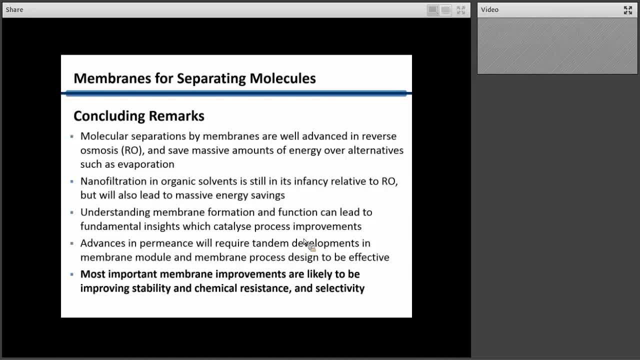 energy over alternatives such as evaporation. So the invention of reverse osmosis technology has meant that we can recover water- fresh water from sea water- using very much less energy than if we only had evaporation available, Nanofiltration and 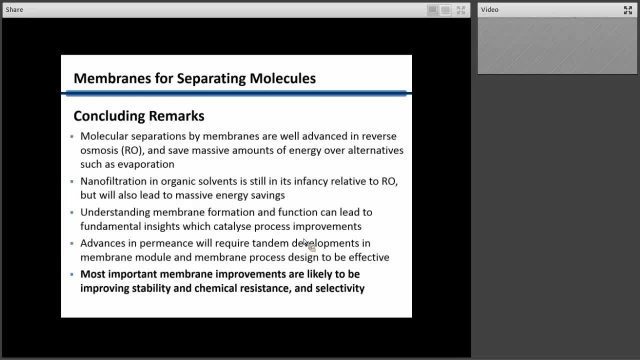 organic solvents are still in its infancy. relative to reverse osmosis, It's not nearly as well established, but I think there is also the potential for massive energy savings if we can develop ways of filtering organic liquids into the membrane. So I think that 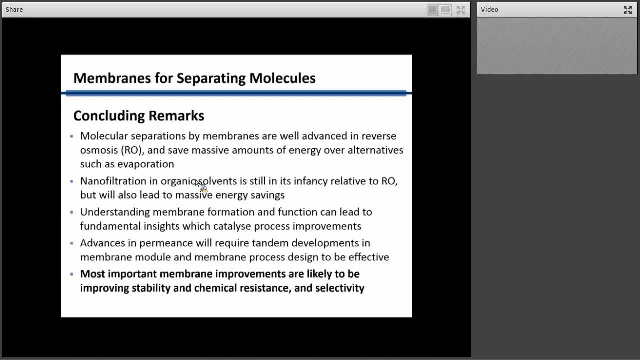 there's a lot of interest in using membranes instead of using energy to evaporate those liquids. Understanding membrane formation and function can lead to fundamental insights which catalyse process improvements. So, for example, by having a platform where I can play around with. 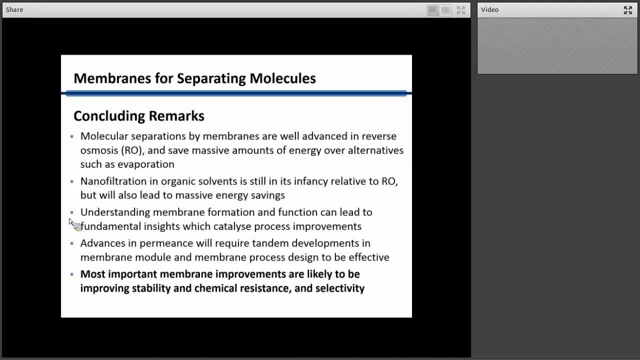 the membrane separating layer and the support independently. we've been able to show that fouling, previously thought to be a function of the roughness of the membrane, may not actually be dependent on the roughness of the membrane, but may be more effective than. 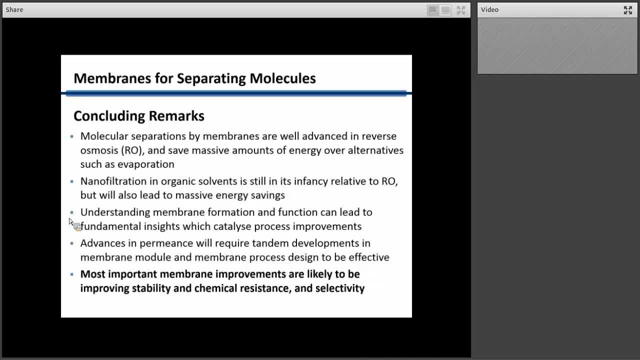 a function of the roughness of the membrane. So I think that there's a lot of interest in using the membrane to create a function of the membrane. So I think that the system is going to be much more efficient than the system itself. 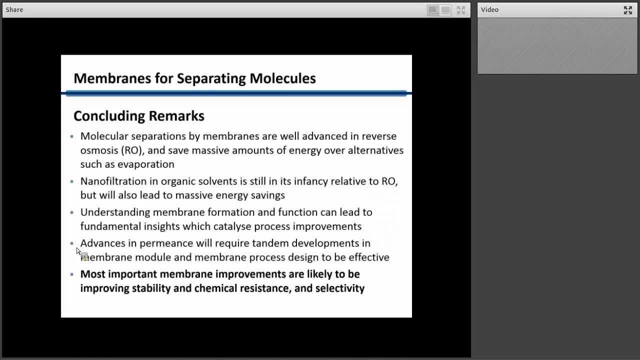 So I think that there's a lot of interest in working with a system that can be more efficient than a system that can be more efficient than a system that can be more efficient than a system that works thoughtfully, collaboratively. 束 and secondo c. 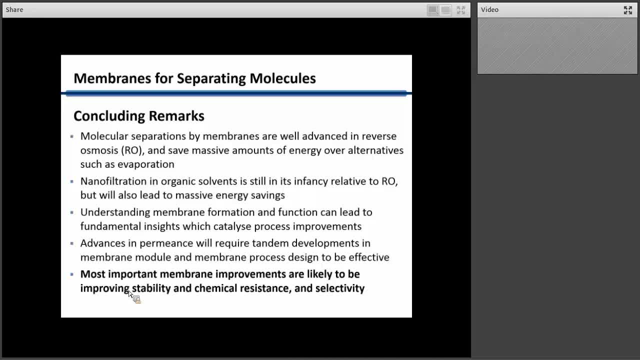 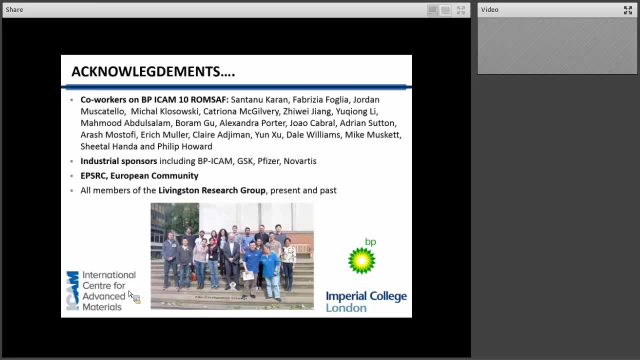 and when music should be expensive, actually with ever better selectivity, so we can start to compete with the sorts of selectivity we can achieve with distillation. So just in conclusion, I'd like to acknowledge my co-workers on the BP-ICAM-10 Romstaff project.